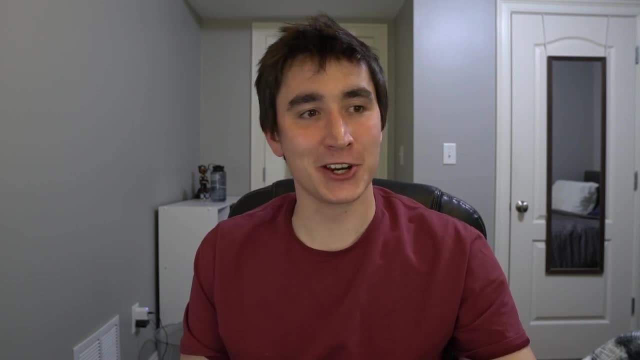 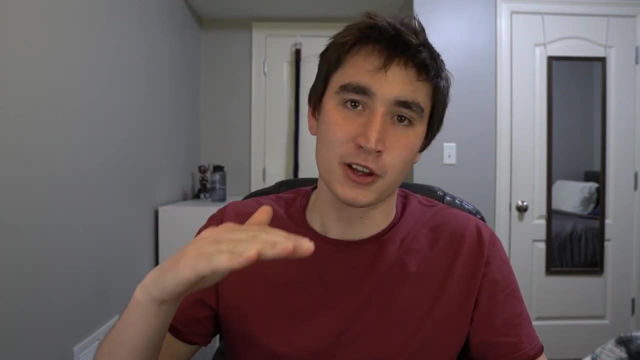 in Python. I'm bummed that I couldn't be there in person to share this with all of you, but this online presentation is the next best thing, so I'm excited to get started. In this tutorial, we'll kind of start with the basics and kind of some of the more traditional NLP models and we'll walk our way. 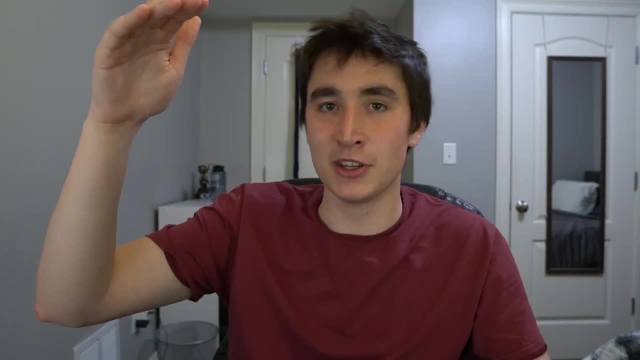 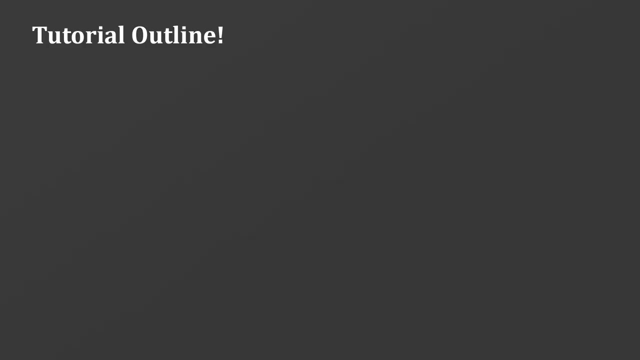 up to some miscellaneous NLP techniques, all the way up to these state-of-the-art language models like OpenAI GPT-2.. So this tutorial is going to start with the basics. It's going to start with kind of the NLP fundamentals. We're going to look at basically how you can take text and convert it. 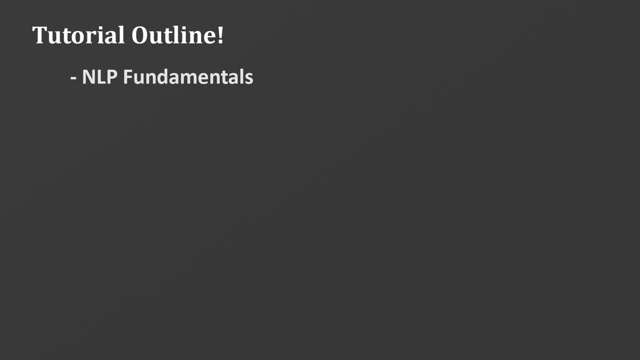 into a numerical vector, and probably the easiest way to do that is what's called bag of words. So that'll be the first model we look at. We'll spend a little bit of time high level overview of it and then we'll jump into Python code related to it. Then the next thing we'll look at is a. 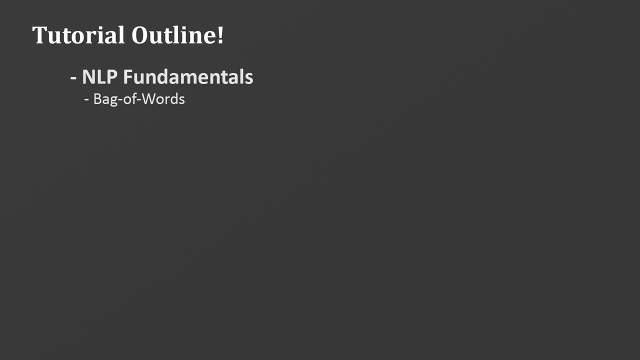 slightly different variation of how we can convert text to a numerical vector and that will be a word vector approach, and we'll also see how we can use Python code to implement models that use word vectors. After we go through kind of the NLP fundamentals, we're going to go through all sorts. 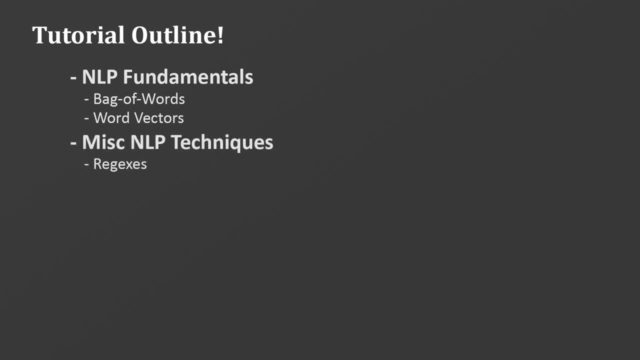 of NLP techniques. So we'll go through regexes, basically pattern matching in Python, We'll go through stemming and lemmatization, We'll go through some basic spell correction, some basic part of speech tagging, and we'll finish this tutorial off by kind of giving it a high level. 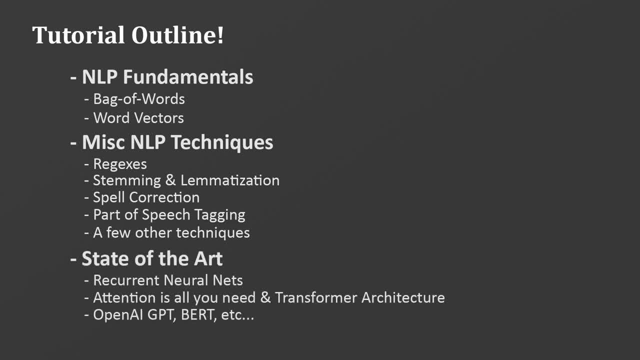 introduction to the state-of-the-art models that I mentioned, So this OpenAI GPT-2 model and, more generally, Transformer, what is called in Transformer architectures- So another big name one is BERT. So we'll kind of introduce and see how those came about and I'll show you how you can use Python. 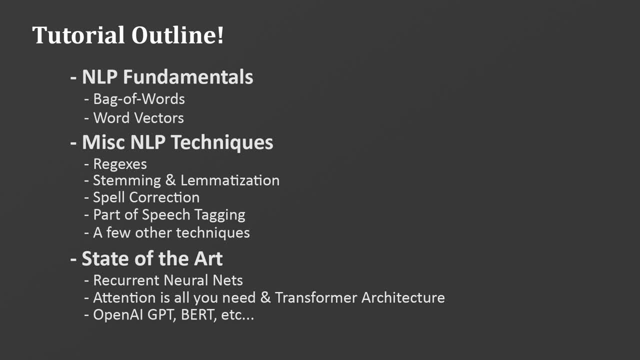 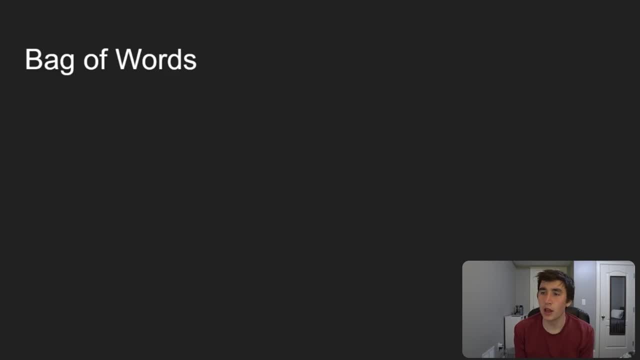 code to play around with those and build even more powerful models. The first model we're going to talk about is called the bag of words model, or also sometimes called bags of words model, and to give you a little bit of intuition behind this approach, I mean whenever we're doing any sort of 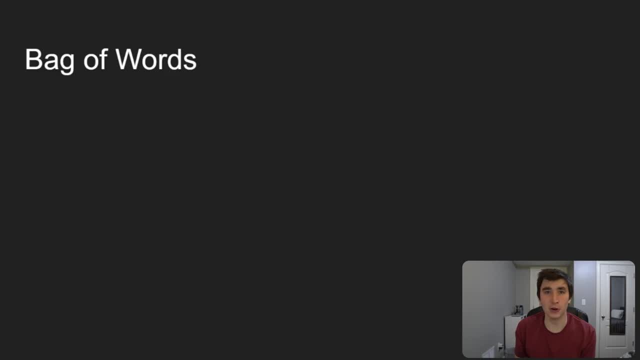 data science related task. we like working with numerical vectors and obviously our issue with numerical vector. So this bag of words approach is kind of the easiest way to take sentences and you know pieces of text and convert it into a numerical representation. So imagine we have the 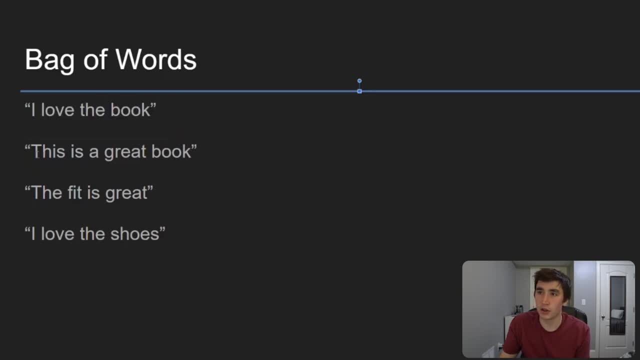 four utterances. I love the book. this is a great book. the fit is great and I love the shoes. These come from two different types of categories at our retail store- the books department and maybe the writing department- and we're trying to build a model to tell them apart. Well, what we can do with. 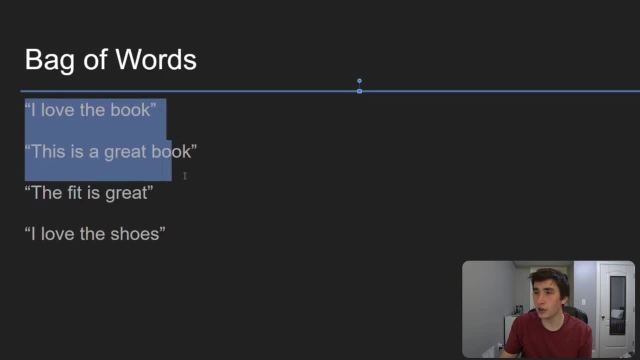 the bag of words approach is it basically says: take all of the words that we see in all of our utterances and just extract out each individual word, each unique word. So that would give us. I love the book- this is a great fit and shoes. Take all those words and then based on what words? 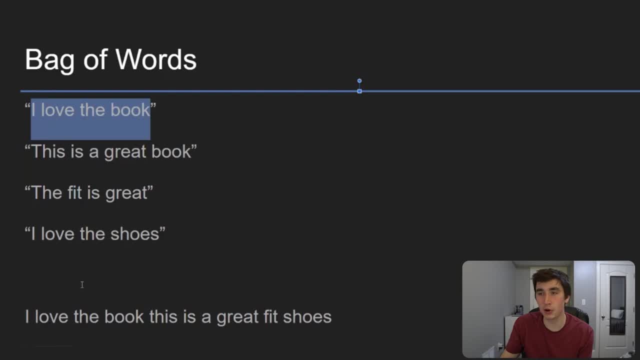 take all of the words we see in all of our utterances and just extract out each individual word, each unique word, So you can compare them. And what we can do is you can use this to form an iterative model where, like, we don't have to label them, we can just separate them out. So there's a couple of ways you can do. 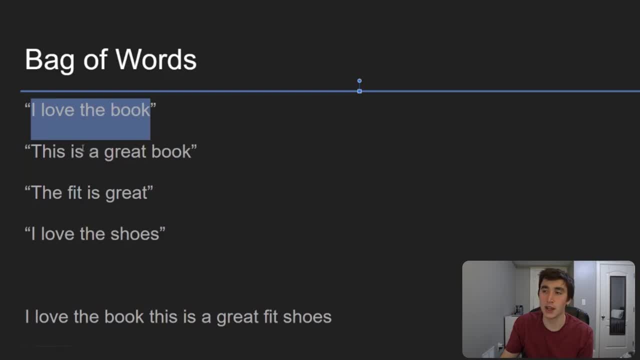 that. So in my example, we have the size of one sentence and I have the size of one word. You can do a binary bag of words model, where you have a ton of words in the bag and then you have a total number of words in the bag, And so what does that look like in code? Well, I think whenever we're 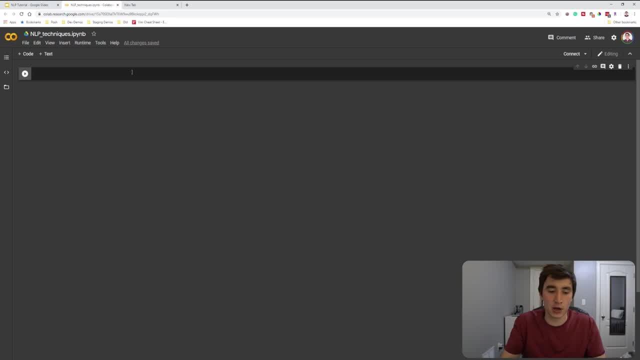 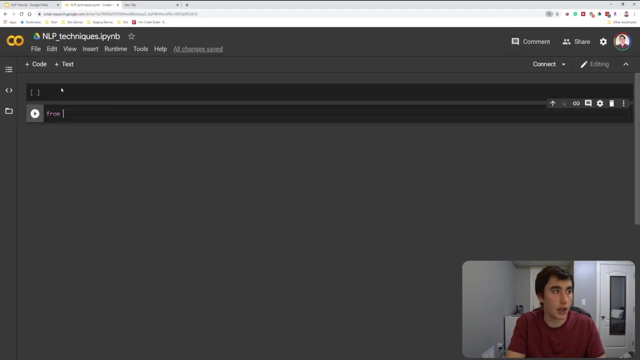 building a bag of words model. the easiest library to use is the standard form of a binary bag of words: scikit-learn library. so we're going to extract a couple things from the scikit-learn library- i'll make my text a little bit bigger- from sklearnfeatureextractiontext. 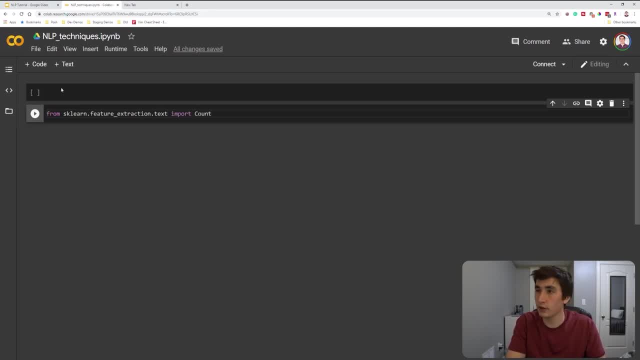 import, count vectorizer and tf, or sorry, we'll just start with the count vectorizer. so when it says count vectorizer, this can be either a binary bag of words that we just mentioned ones and zeros. it also could be, if you imagine, one of these phrases i mentioned: i love the book, the book. 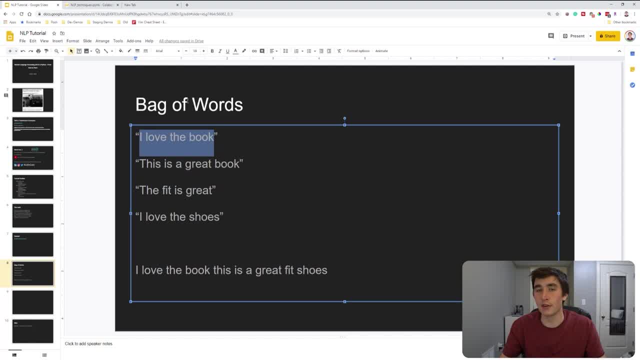 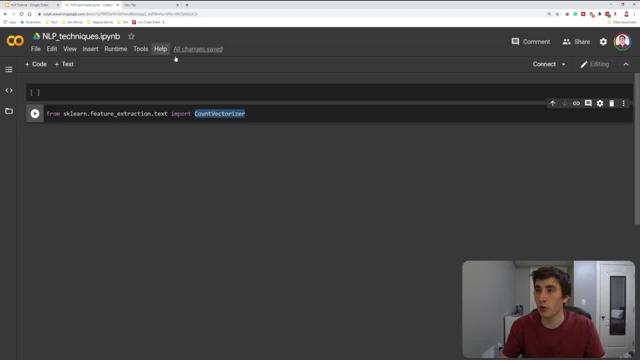 was great if that was all like one sentence. maybe a count vectorizer could also say that book appeared twice. so it would be a rough a straight count of the word in the overall sentence how many times the word appeared in a sentence. but i usually just tend to use a binary approach. 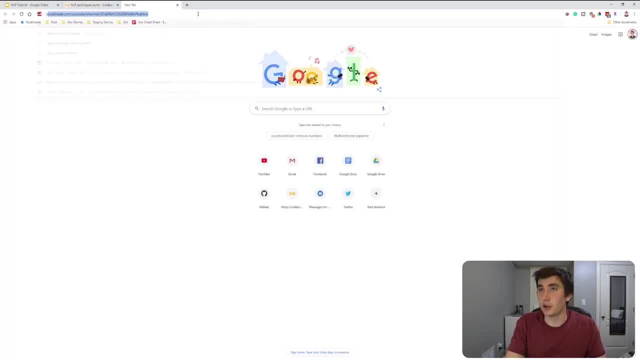 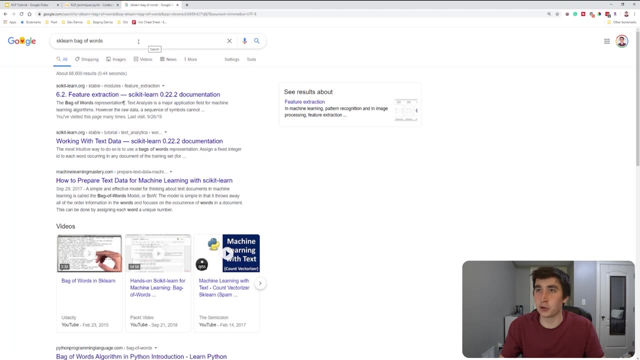 you if you ever don't know how to find something like this, if you know of the bag of words model but you don't know where to look to find it, i just literally would do like a google search sklearn bag of words and you'll get to the scikit-learn documentation and through that 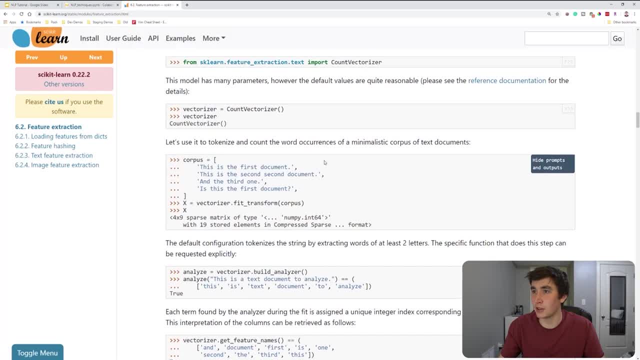 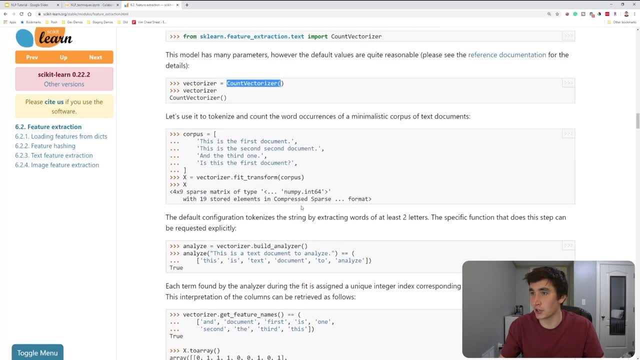 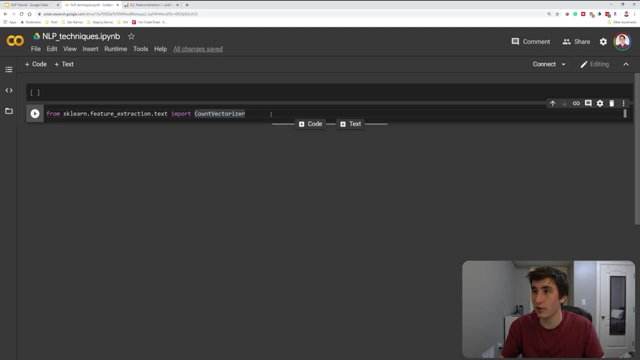 you should be able to find some examples using a bag of words, basically, so here we have the count vectorizer that i just showed you, and it shows us how to to utilize it. so we might reference this a couple times as we do this. so we have our count vectorizer. 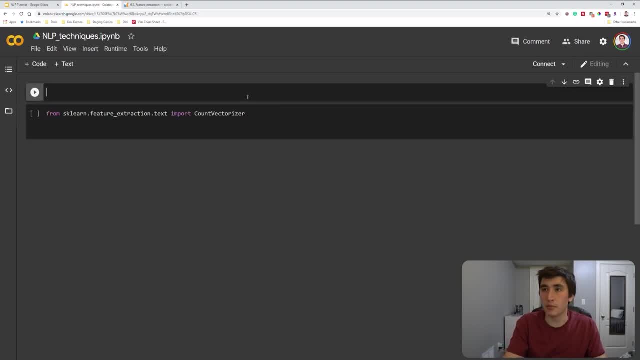 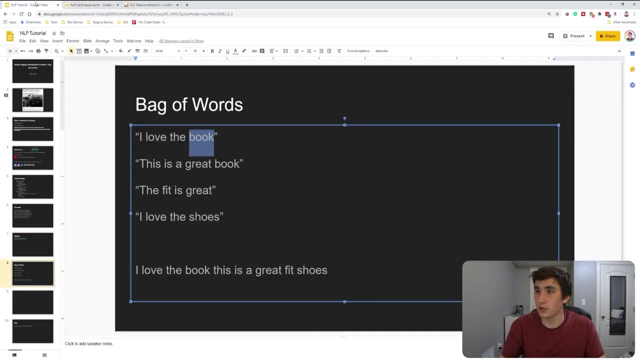 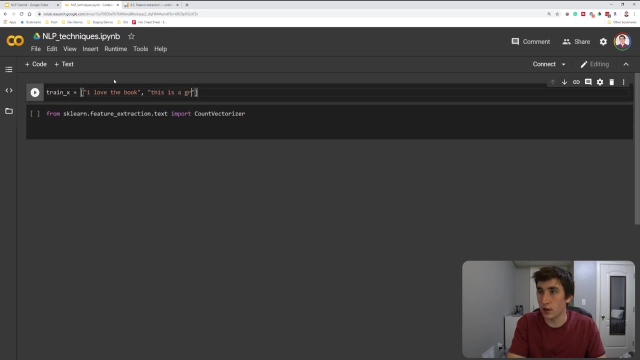 and above this, i'm going to just real quick to find some training references. so i'm going to call this train x. i'm going to say: let's use our examples. i love the book. there's the first one. i love the book. this is a great book was the second one, and then the last two were: 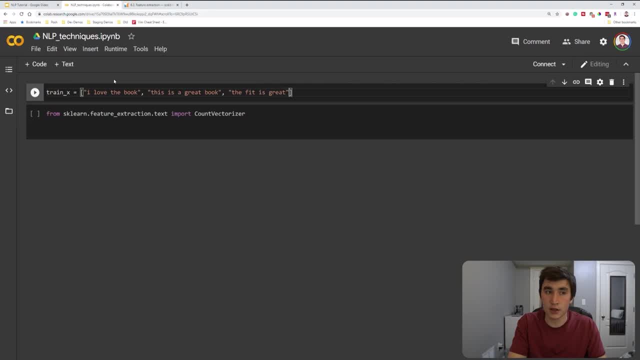 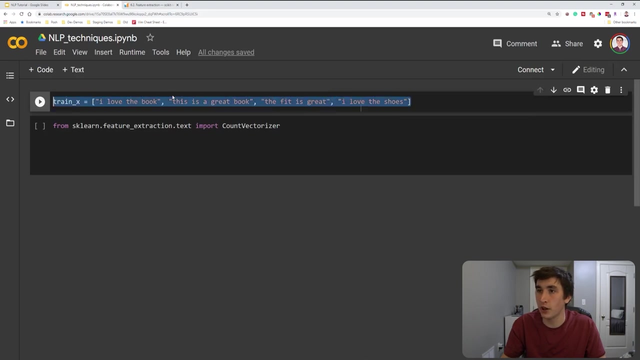 the fit is great and i love the shoes. all right, so that's our four training utterances we can imagine. so the first thing we might want to do is utilize our count vectorizer to transform this into a vector representation. so once again, i'm going to reference the document. 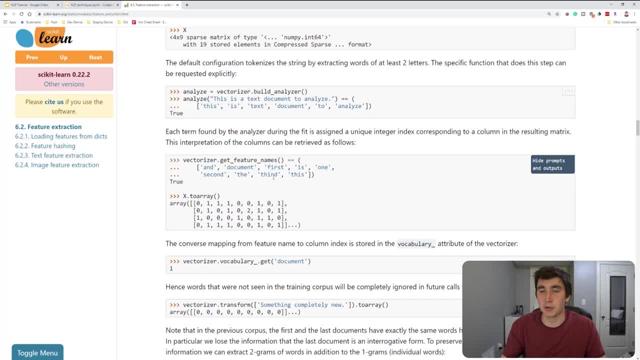 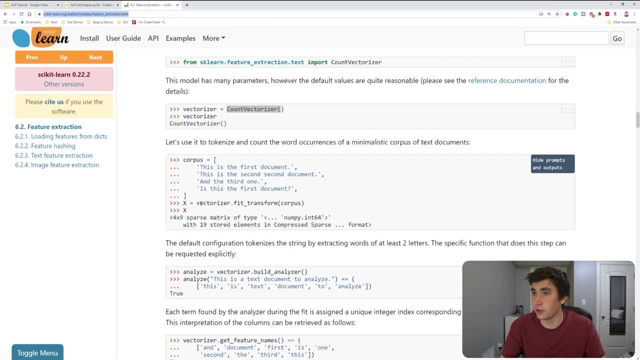 here and you know, I know what I'm trying to do, but I'd sometimes forget the syntax. so this is why I always reference documentation like this. so it looks like we want to use vectorizer, dot fit transform, so vectorizer equals count vectorizer and then fit transform on our sentences. so we can do that. so we can. 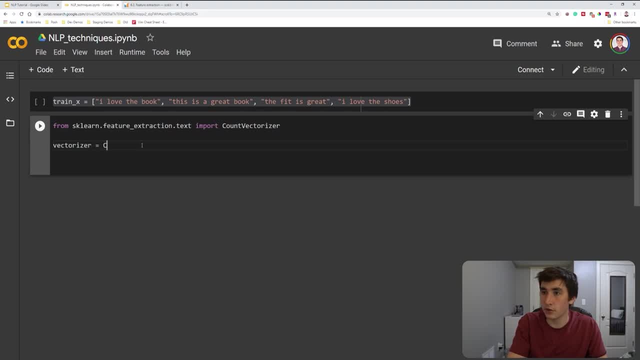 say vectorizer equals count, vectorizer, vectorizer, and then we can say our vectors are equal to vectorizer dot fit, transform, train X, and when this says fit, transform, it fits a dictionary around our training, on our instance. so basically, that's the first step and it's finding all the unique words, so it 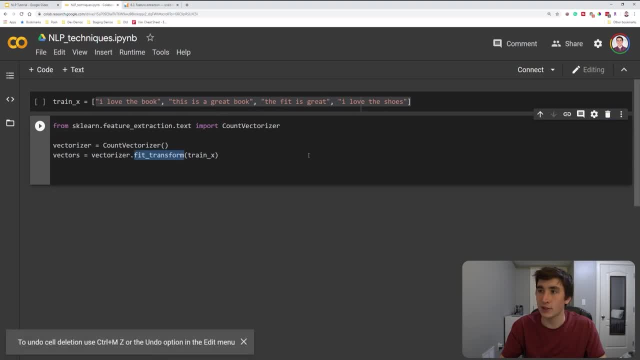 knows how to make these vectors and then it's going ahead and transforming the utterances we pass in based on that vector that we just fitted. so now we get our vectors. so I could do like print vectors zero and it'll be the vector for I love the book if this runs. 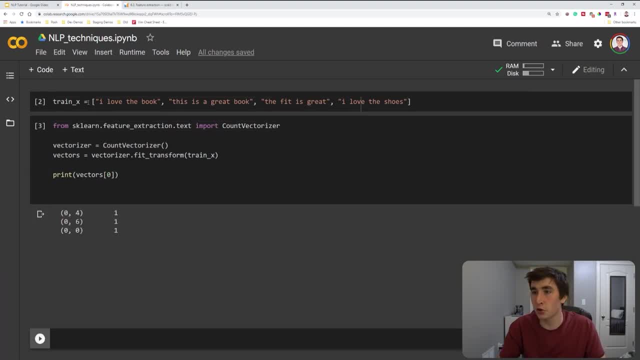 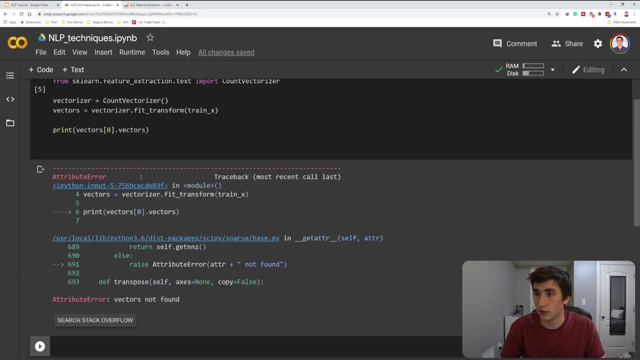 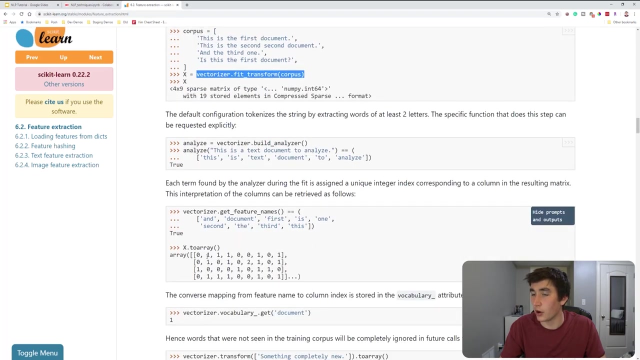 train X is not defined. Irun the cell to. I'm using Google collapse right now to run this. ok, looks good. my just do that vector. think it is found. tiers. just see our apprentice. real quick, i guess we do to array to see how it actually looks. 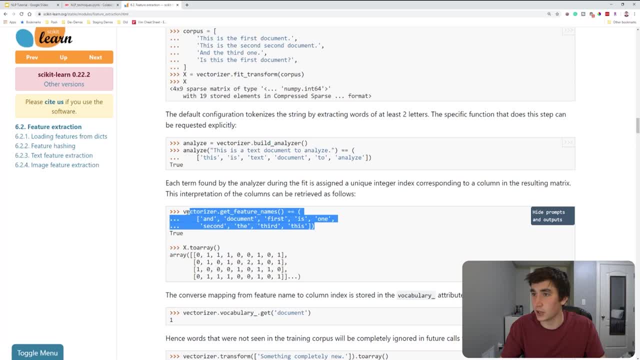 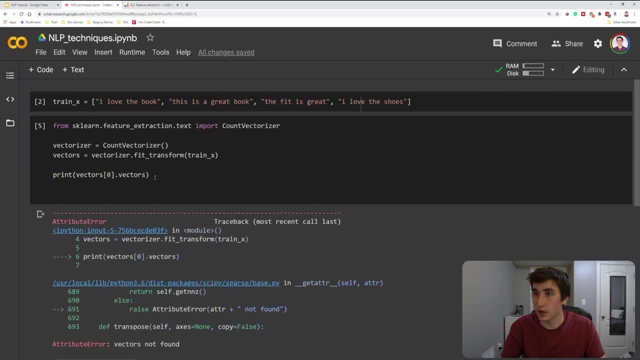 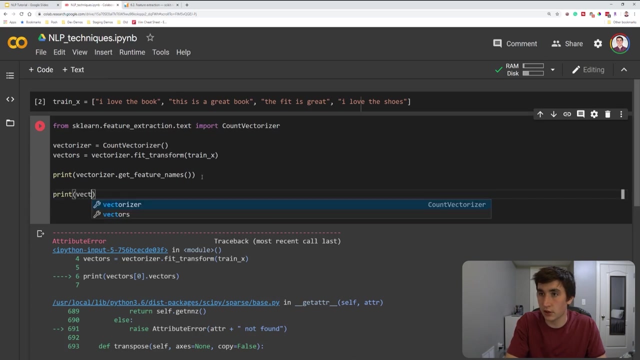 3: do vectorizer dot get feature names? that looks helpful too, so I'm gonna print some things out. I'm gonna print out: vectorizer dot get feature names and I'm also gonna print out, let's say, vectors. print vectors dot to array. let's see. 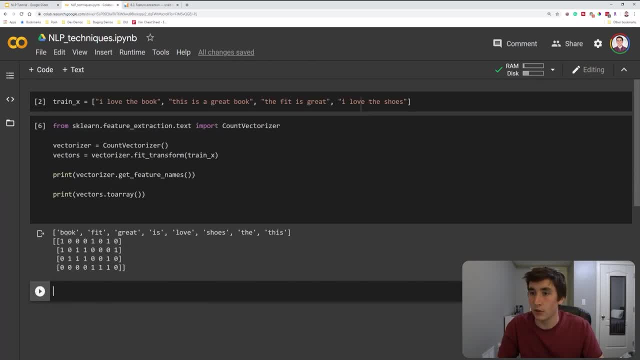 what happens. okay, cool. so our different words in this dictionary are: book fit great is love, shoes, the, this and one thing to note is it looks like it actually stripped away the a, so that might be just a feature of you know one word utterance is it? it strips away part of the way that this count vectorizer is. 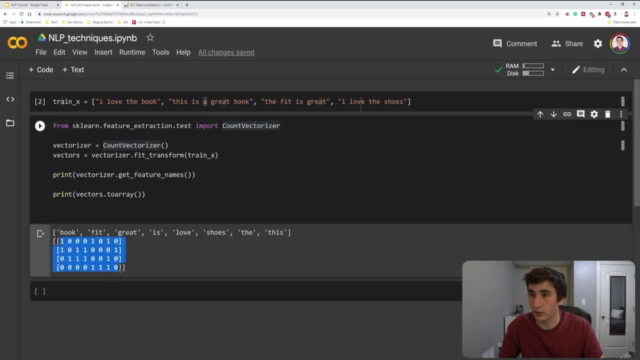 implemented. but if we look at the vector here, let's look at the first utterance. well, that's, I love the book. a one here for book right, one here for the love right. thus the second to last, we have a one there and I guess it's shipped away. I as well, so we don't see. 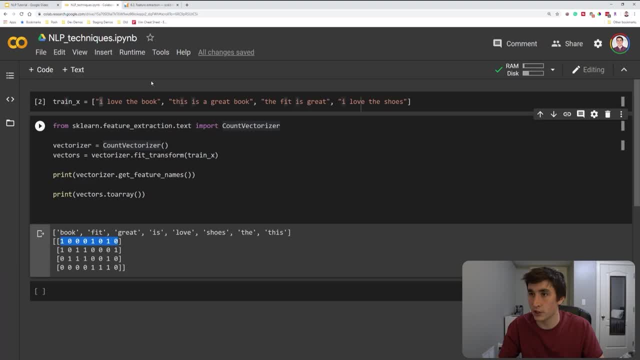 that, but we get a vector representation other than the one word utterances were this vectorizer doesn't count, and one thing to note is that I think by default if I need this, I love the book book, uh, count. vectorizer is non-binary, so it actually matters how many times you type. 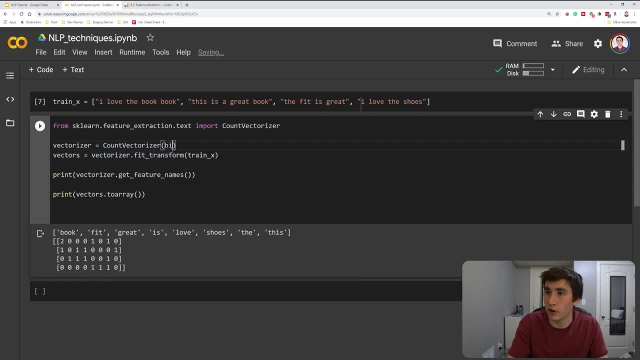 something in. so if you wanted to, you could do. i think binary equals true here, and now it switches back to ones and zeros. okay, so that's the basics of the bag of words, just seeing it and making a very toy example of doing it. let's build a quick model to actually classify these. 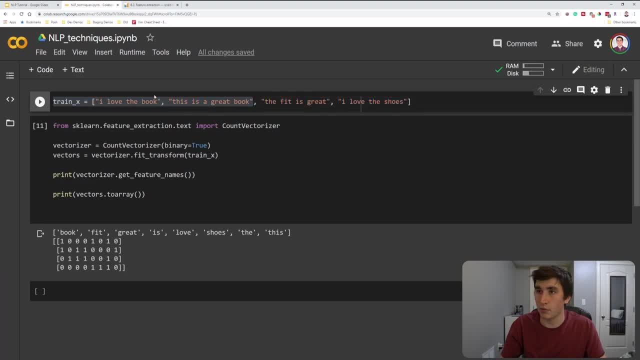 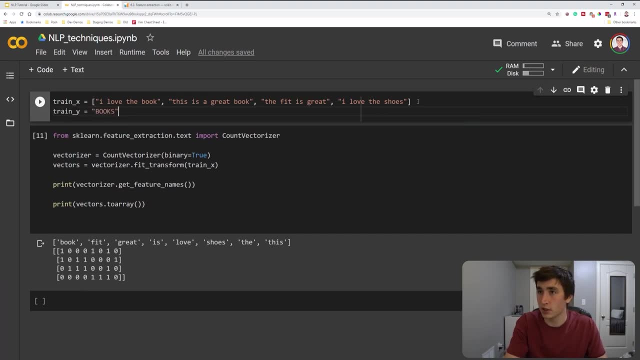 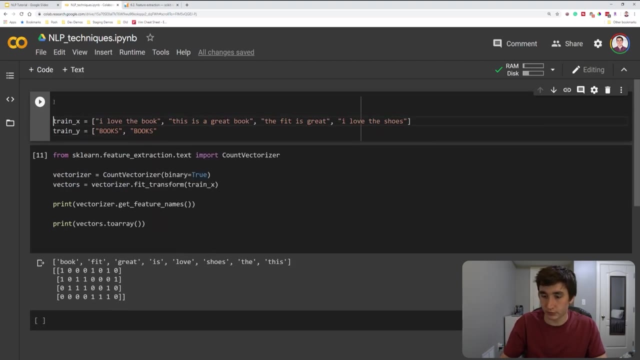 as being clothing related and these as being these first two being book related. so i'm going to call something train y. so that's going to be first one's books, second one's books, and whenever i have a repeated string like this, i like to make it its own variable, just so i make sure i don't. 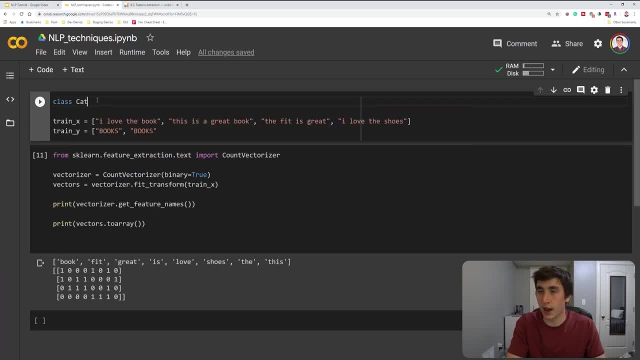 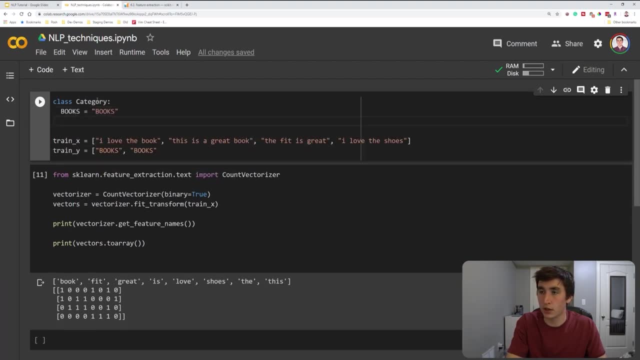 actually like misspell it. so we're going to make a class category real quick and just label books as one of the categories and that's going to be the string books and clothing as the other category. and you'll see why i'm doing this in a 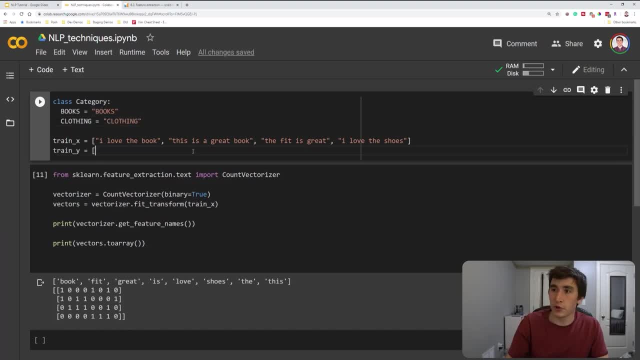 sec. so now, when i want to, i'm doing this in order. so i have four things. i'm going to give them their four labels in order. so we have category dot books. we have category dot books and then the last two are about clothing. so those are category dot clothing. 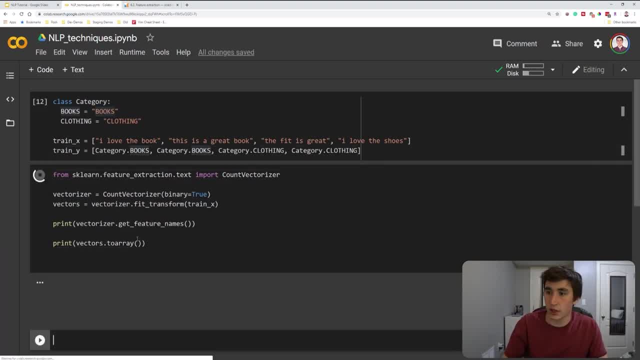 all right, and i'm going to run that again, run this again, i guess, and now we're going to build a simple classifier to. i'm going to just hide this print so you can see everything real quick. i build a simple classifier to classify whether these are book, a book category. 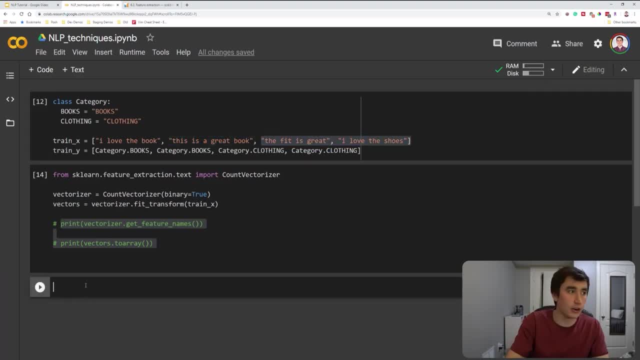 and this is clothing and we can use it on new utterances. so how do we do that? well, once again, the scikit-learn library is very helpful in this, and what a good classic classification model for text is often a linear svm. so that's what we're going to use, so we can do. 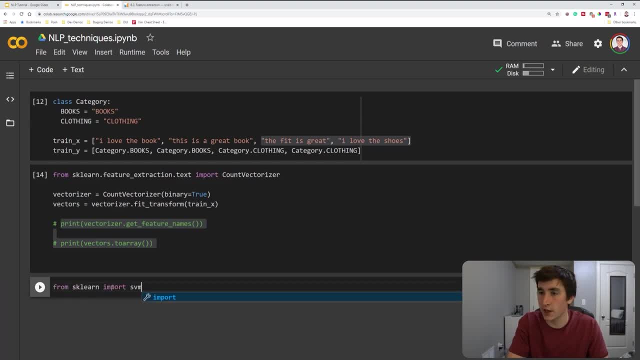 from sklearn import SVM. and then we can define our SVM by the following. I'm going to say: classifier SVM equals SVM dot SVC with a linear kernel. so I want to use a linear SVM because it's I know just with my knowledge, like background knowledge, that this is a good classification model for text oftentimes. and then with that SVM, 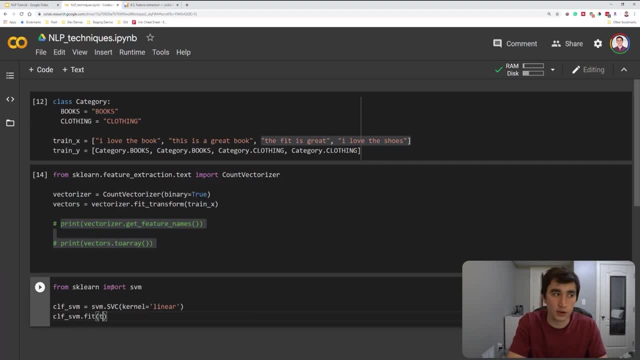 I'm going to do a fit on our training vectors, which is right here, these vectors, because we couldn't just pass in the text. so I'm going to call this train X, vectors, vectors, and then our Y labels, which is just train Y, so this should fit. 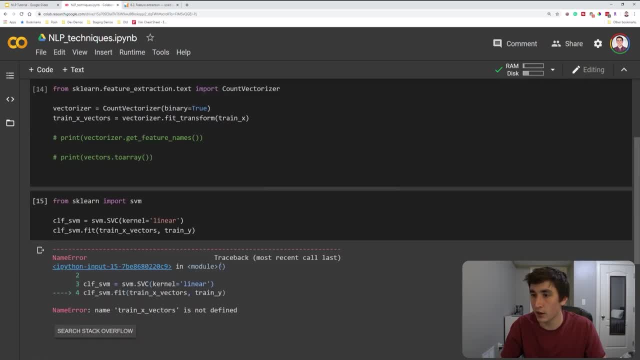 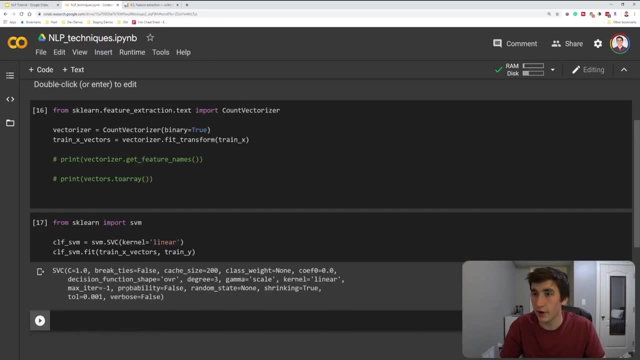 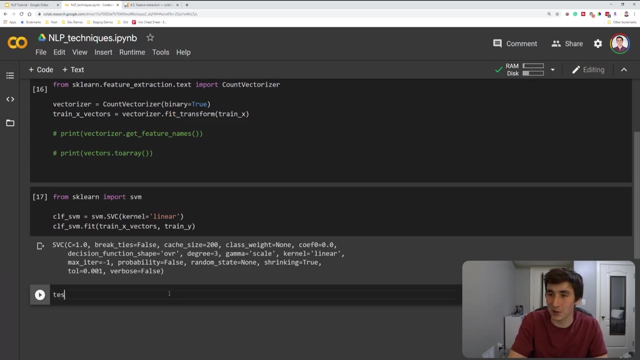 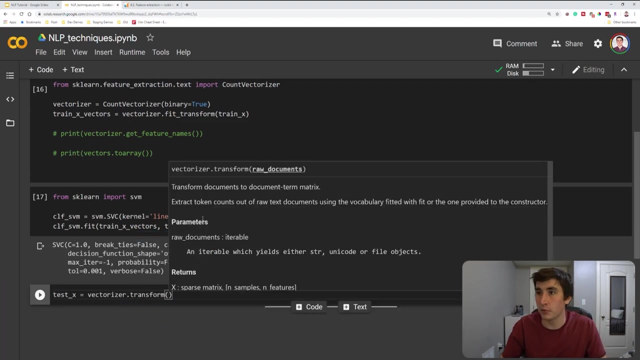 a model to the four utterances we have here. and we got a error. I didn't rerun this, so cool. then finally, let's do the fun part and predict new utterances with this. I'm just call this text: X equals vectorizer, dot transform. so before we had a fit, a. 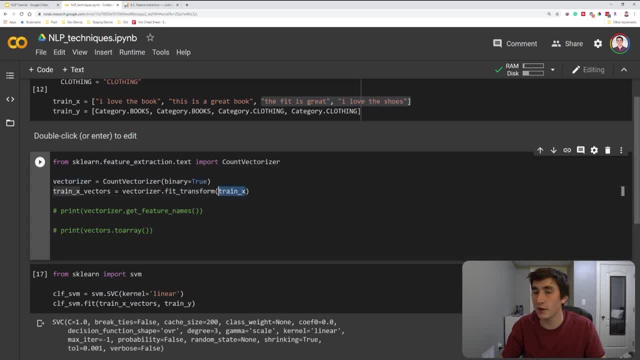 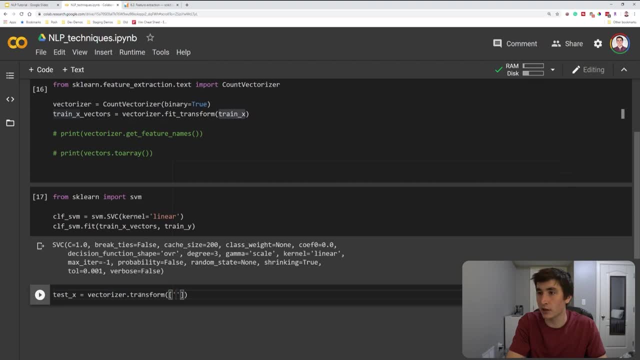 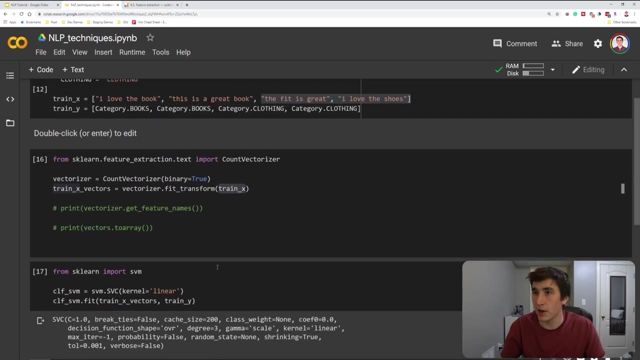 dictionary and transform based on our training utterances. now that we already have a vectorizer, we can just do transform instead of fit transform, and so I'm going to just say something like: how about I like the book? so based on what we have here, because we said the word book. 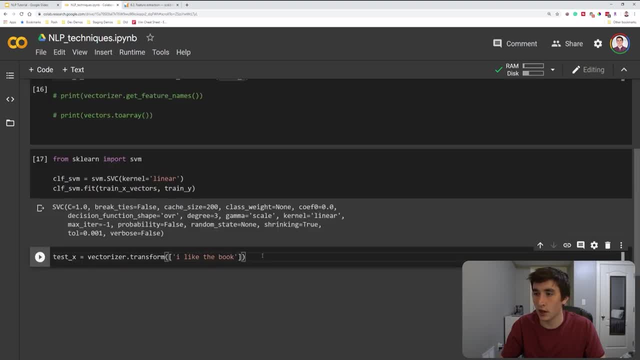 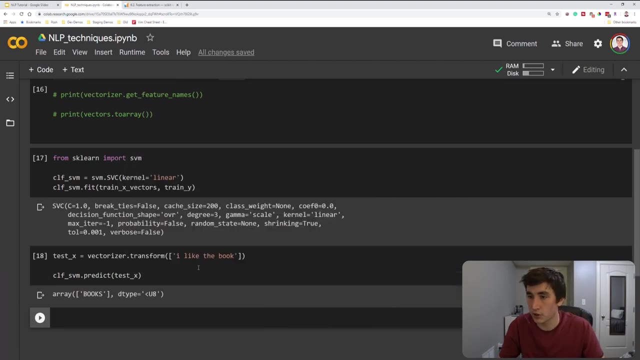 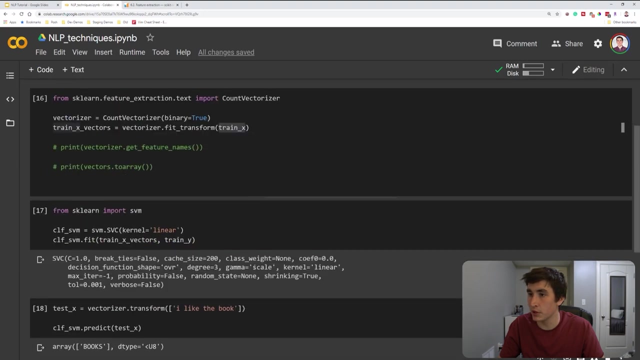 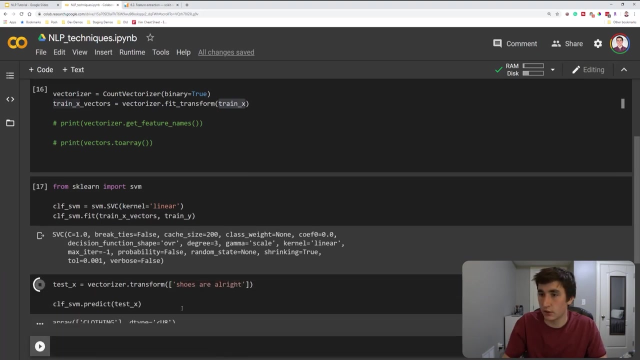 you'd expect that this would classify as the books category. so we can do: classifier, CLF, SVM, predict on our test X and see what happens. nice books, that's cool. let's try. like I love the shoes. maybe we say something like shoes are all right and wow, that says clothing. and obviously we only trained this with four. 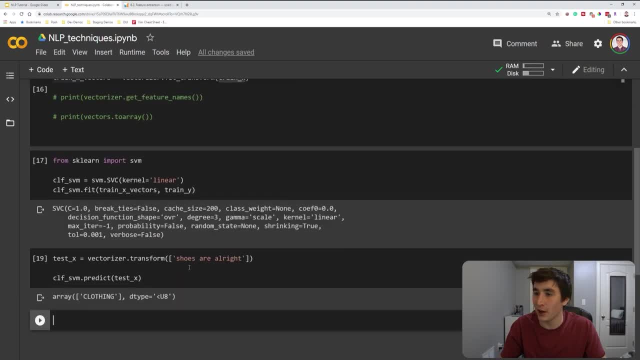 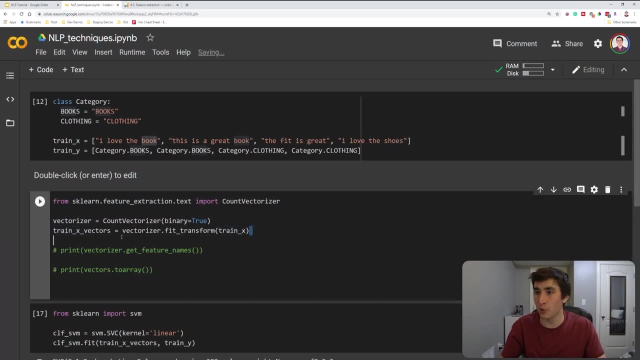 utterances, so it's only be so powerful. but so yeah, it's only going to be so powerful. but as we added more and more utterances to this, our dictionary would grow more and more or fit, transform, and we get a more powerful model. so the more training utterances we feed into a bag. 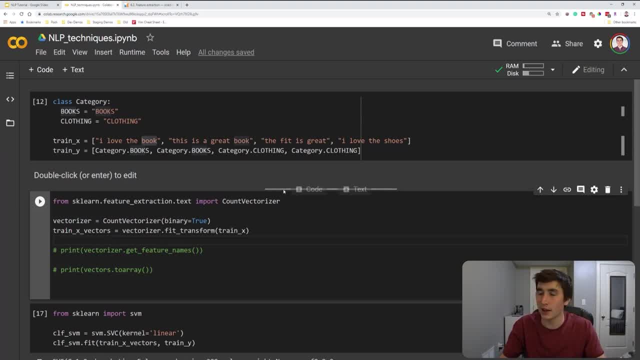 of words model. oftentimes the better it does, and i guess one of the caveats to that is you might build such a big dictionary that it might get hard to process, like the model. so another technique you can add in here, and definitely sk learn offers you some ability to do this is maybe you only 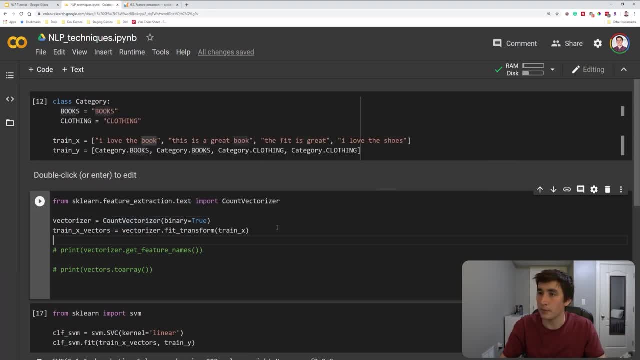 take the top 1 000 words that occur, so that's like another option. another thing to know about bag of words is: right now we are doing a unigram approach, where we're just taking each individual word by itself, but you could also do a bigram approach- it's called- which would categorize. i. 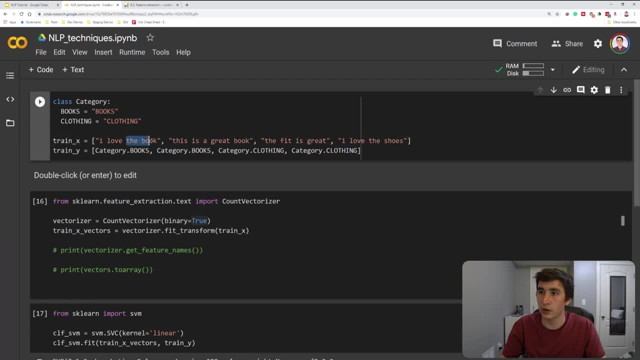 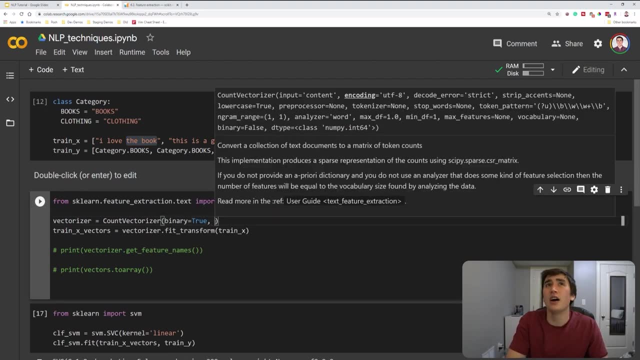 love, love, the, the book, all as their own unique utterances. so let's try to do that real quick. just you see, uh, let's see what we have: engram range. that's probably going to help us. so i'm going to type in engram range because it probably will give me some more information about 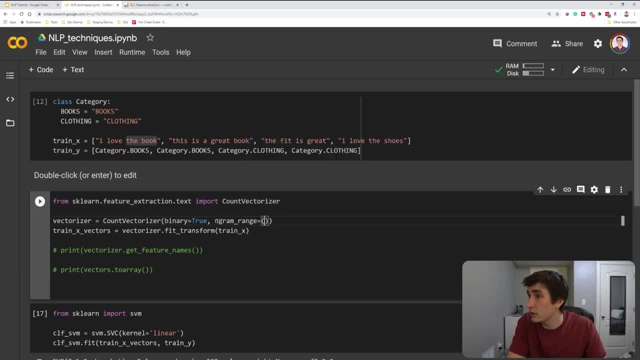 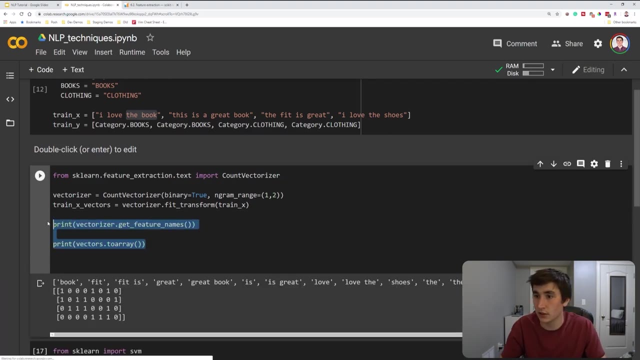 that equals: oh, so i'm going to say one, one and two together, i think both one words and two words, so we can print this stuff out again then see if that is the case. yeah, so now you see, we get two words as well. so that we just now captured you um bagrams as well. 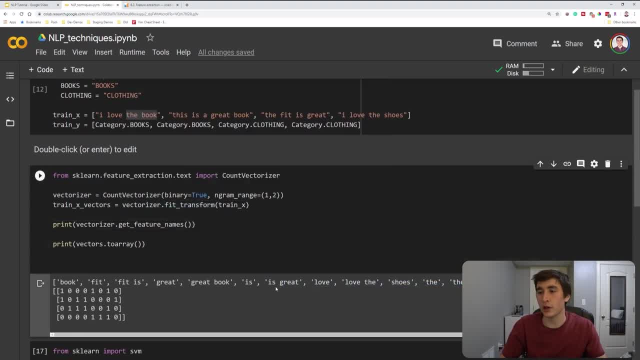 and one thing to note about these biograms. one reason you might want to use two words in a row is, let's say we were talking about if things were positive or negative. well, if i say something is great, that's very positive, but if i use a biogram and the word before great is not. 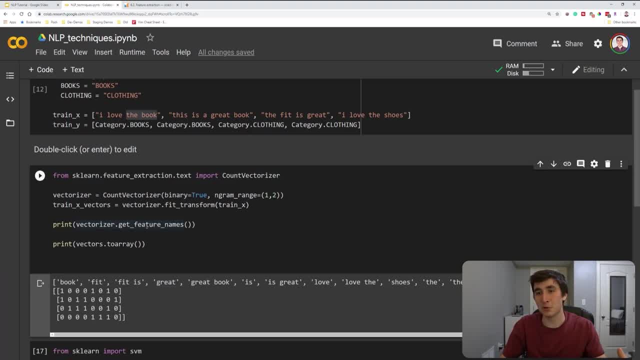 you know, not great, then that's a completely different sentiment. So that's one way. you know, engrams are important And, as you, you know, words depend on their context. So you know, adding additional words in this sometimes helps. It could also be detrimental. 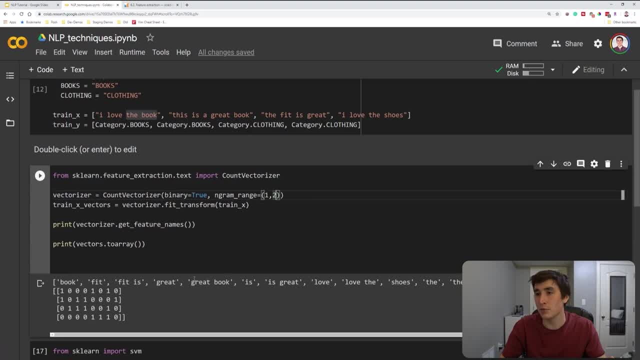 if you had too many words here in the engram range You might have so many like random, miscellaneous, like three word phrases that only occur once in your entire set, and it might actually skew the classifier off of it. So I'm going to just stick for now with just a single. 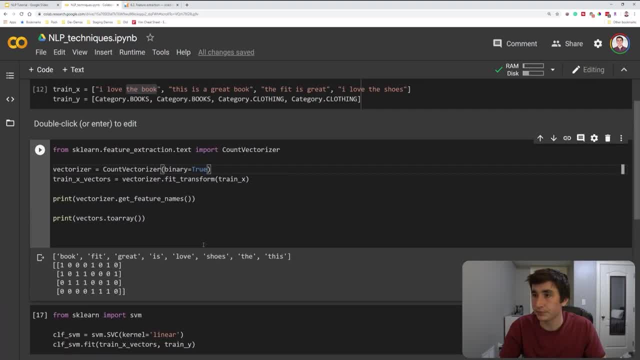 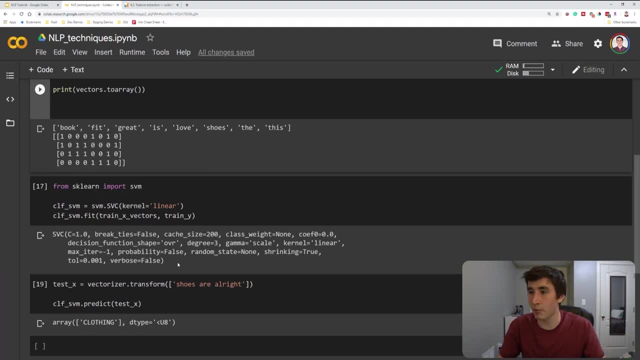 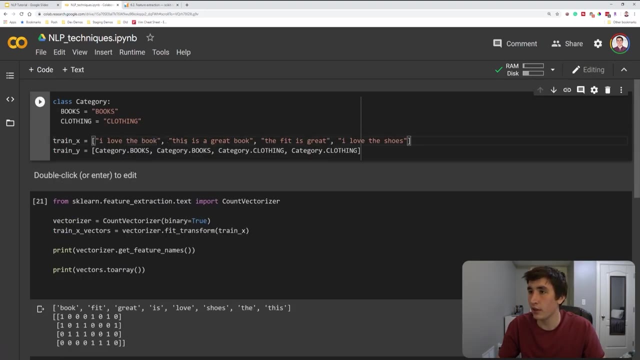 one unigram model, And here's the final. the final thing I'll say about bagger words before we get into the next model is: here's the limitation is: if we have a word that is not in our training utterances, we're not going to know how to handle it. So if I said something like 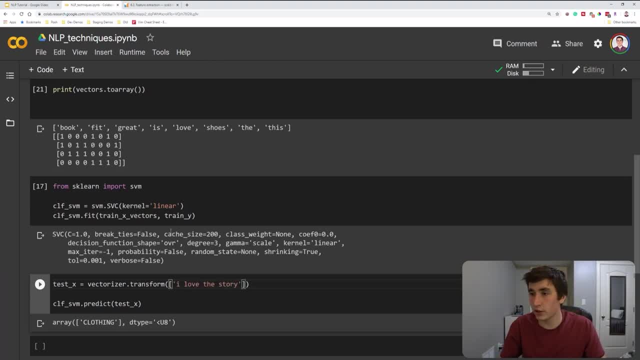 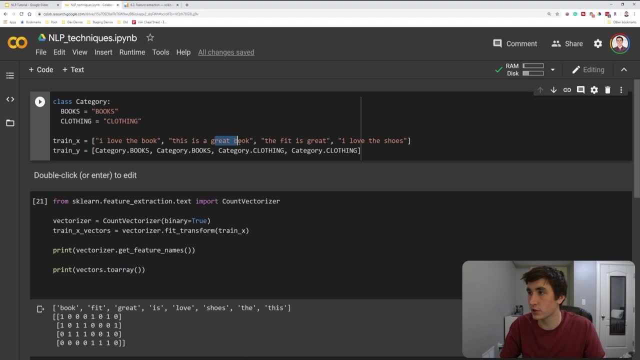 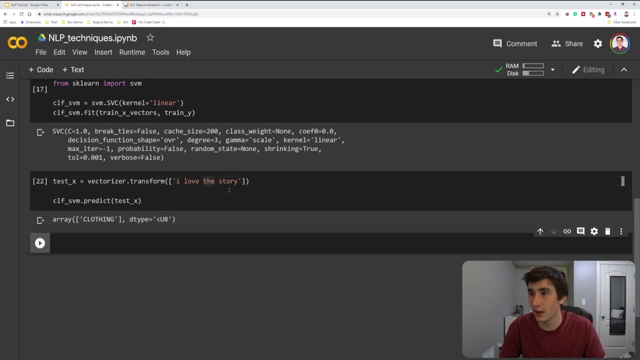 I love the story. Well, to us that's very similar, you know, to book and books, But to our model. we've never seen the word story, So we might not know how to handle this. So let's see what happens when we run this. And here's the issue. Yeah, it classified it as clothing. 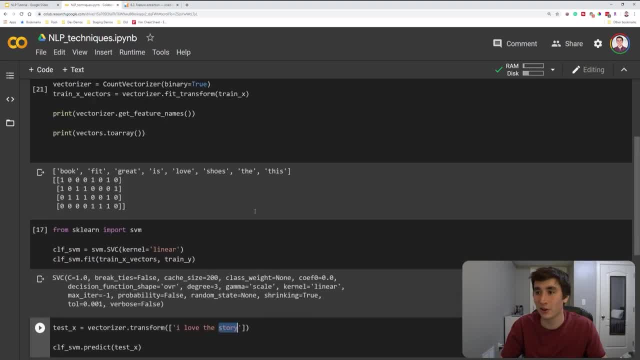 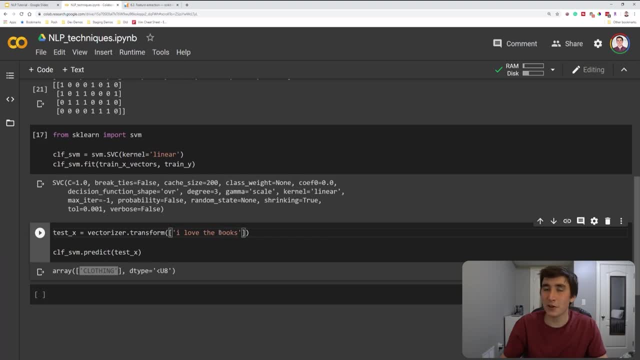 even though it's obvious to us that story and book are very related. And honestly, I think even if we typed in something like books, it doesn't know that book and books are the same because it has seen the word book right here but it's never seen books. So it's like pretty dumb if it hasn't seen a word. 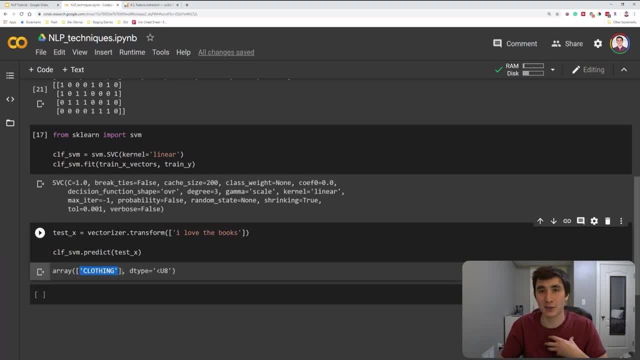 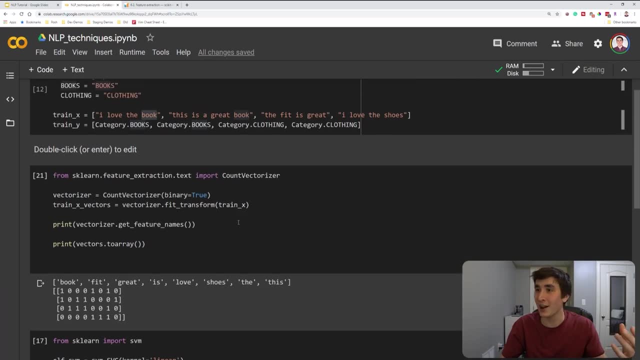 And yeah, again, it says clothing, even though it's very obvious to us that book and books are the same. So that's one downfall of bagger words is it's great on the stuff it's trained on, But if it hasn't seen a word then it just fails miserably. And you know that's not great when. 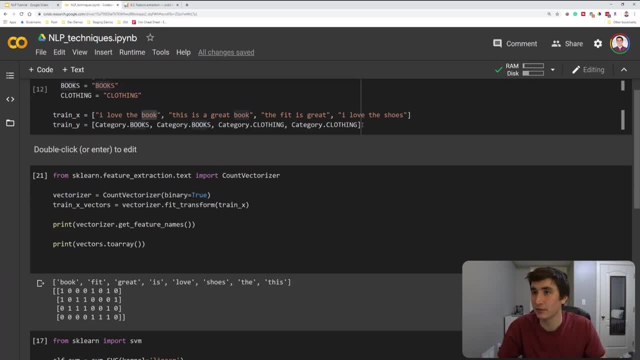 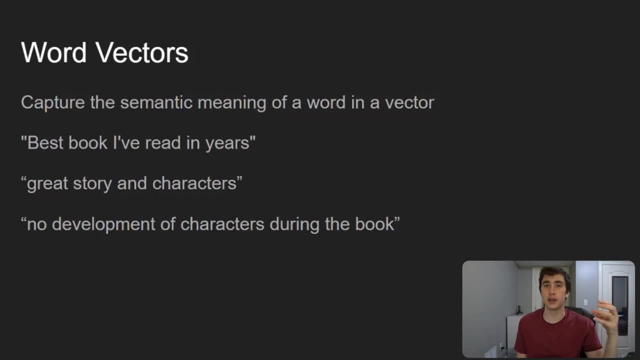 it's made on the upper side. But that little formula I just shared with you is good enough for things like running a book or a book in for classes and reading out like a oral exam, which, let's say, impression that that stuff is better, then those things that you're writing that book in. 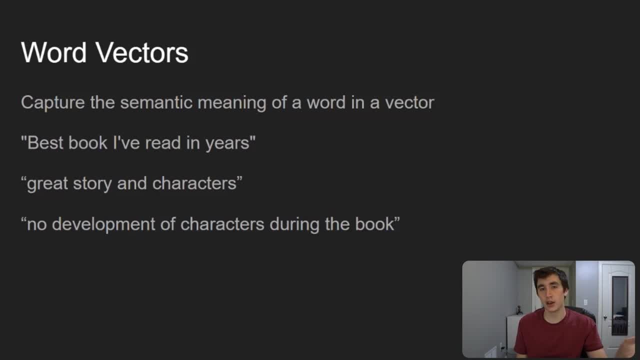 would fail miserably. So it's it's you can. you can try and convince people to purchase this therapy if they can't read it too, but they can affect it, And so if you can get the book out of that bagger book- you don't have it. you start to receive information from people like you who don't read. 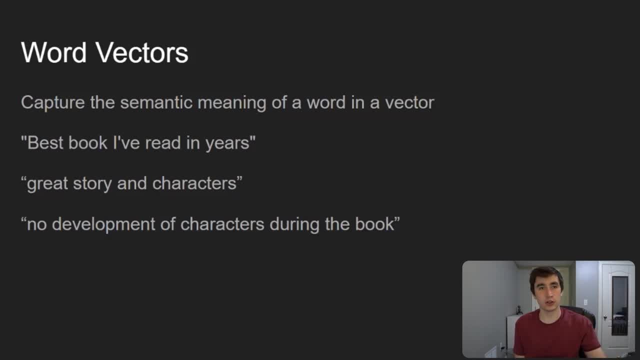 hang in there like something unique right And make them look great with a bagger book and then make themselves feel respected. yellow: these are all three different types of colors and what we're trying to do with word vectors is have in our we imagine you have this big like vector. 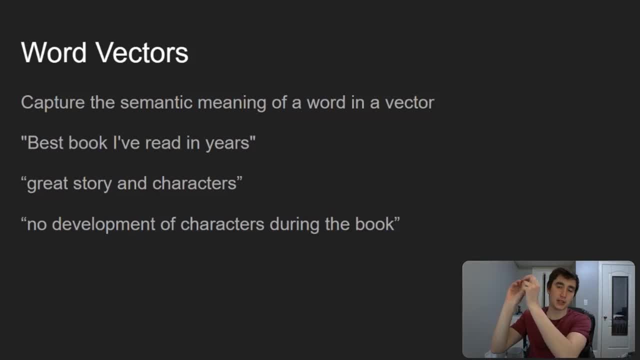 space, we want the similar words to be mapped in a similar spot of that vector space. so red, blue and yellow would all be colors and should be mapped somewhere similar, and there's many different approaches to training a vector to ultimately do this, and one of the popular methods is called word2vec. 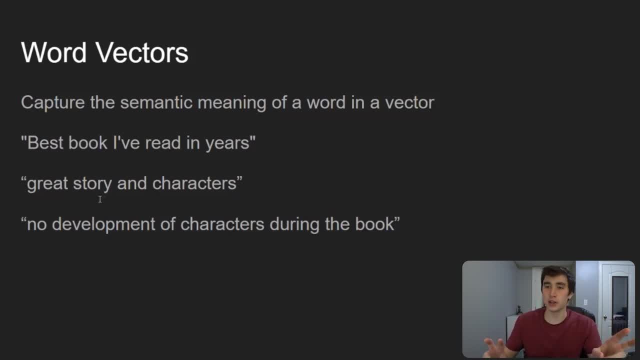 and word2vec works in one of two ways. usually there's two popular- like most popular, I guess- ways of training this word2vec. one's called continuous bag of words and one's called skip gram. the different details of these two approaches isn't super, super important, but what is important is to kind of 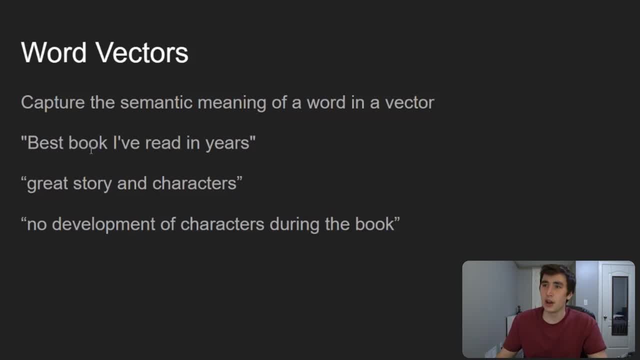 understand at a high level how they work. so imagine we're going back to our kind of example of classifying between books and clothing related tweets. so imagine we have the three phrases we say: best book I've read in years. we have great story and characters and we have no development of characters during book. so 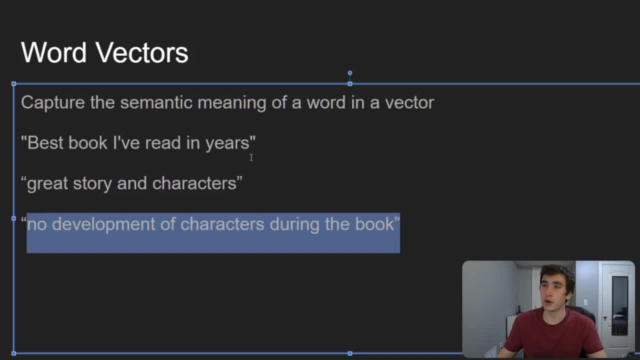 these are three phrases related to books. we can tell this pretty easily by reading these, but how do we turn a model to see that? and what the word2vec approaches do, the continuous bag of words and the skip gram approaches- is they look at a window of text, so oftentimes that window might be, you know, five tokens long. so 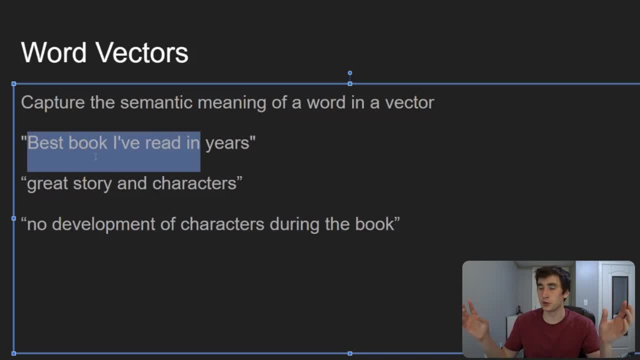 best book I've read in. so that would be kind of our context window and basically what we'll do is we'll selectively look at different tokens in that context window and, based on that token, will utilize the surrounding tokens to kind of figure out the context of each token and kind of start developing a meaning of it. 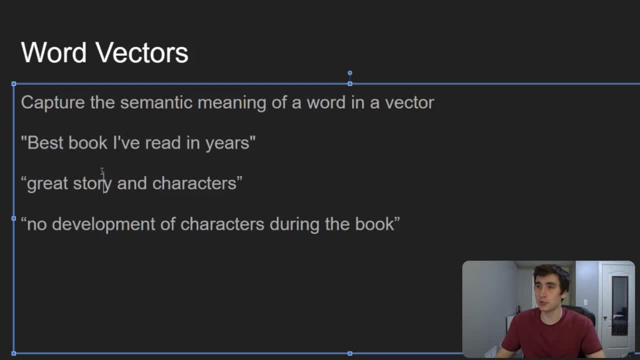 meaning of each token and so translating that to this example we can start. if we read enough text, we can start to see relationships between words. so for example here, one relationship we might develop over time is: book often appears close to read, so now we can associate book and read into a similar spot of the. 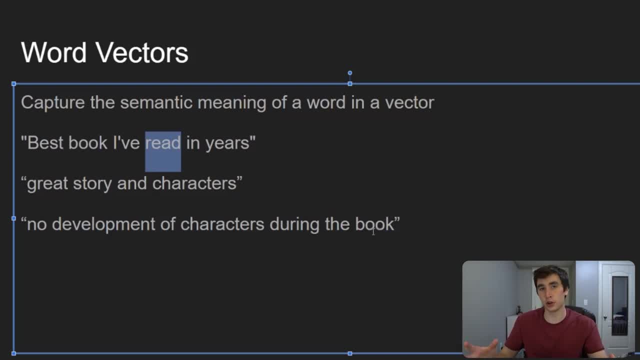 vector space and this is ultimately going to be trained through some sort of neural network architecture for the most part. so, given our neural network architecture, where you know our model is learning that book and read are close together, in this next example you know great story and characters. we might 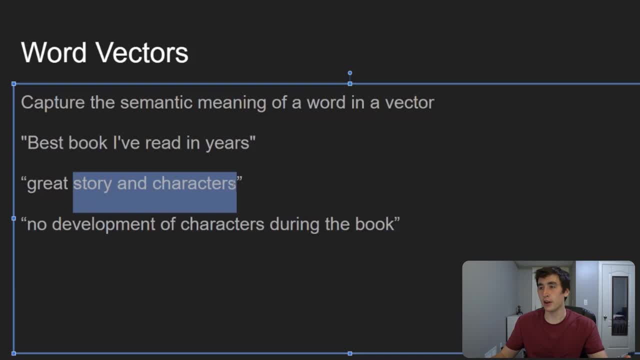 start relating story and characters together, and you know we'll see these together, so we'll know that those are related and should be similar vector space. and then this last example: no development of characters during the book. well, maybe we relate development and characters. that's what our models. 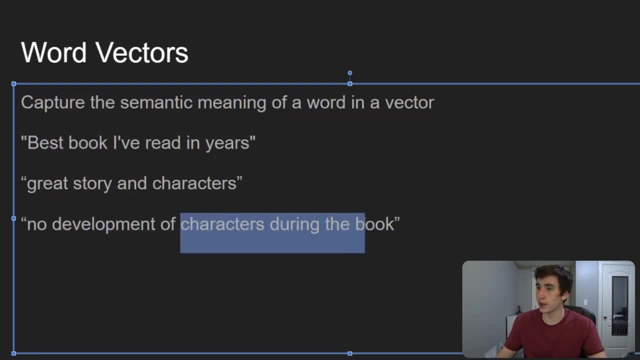 learning, you know, also by learning that characters and book are related and and we can kind of start building out far like bigger relationships, like okay, we've seen characters and book here. we know those are probably related. okay, we go up here. story and characters are often together, so I'm guessing that. 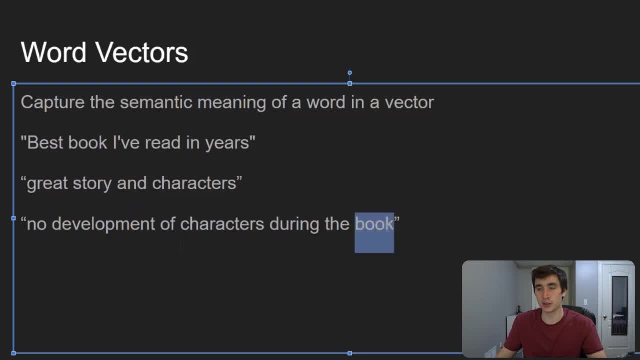 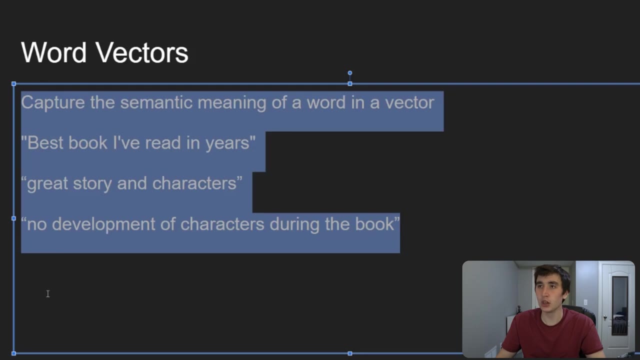 story and book are probably related as well, and this is a very toy example of what's happening, with hundreds of thousands of like sentences being fed into these types of models, and we're ultimately building up these word vectors out of that. so one thing to talk about it. let's start. 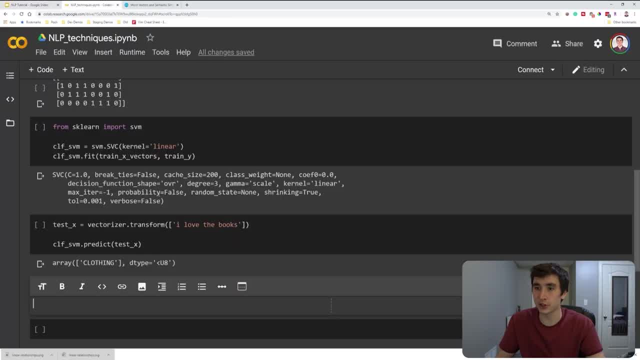 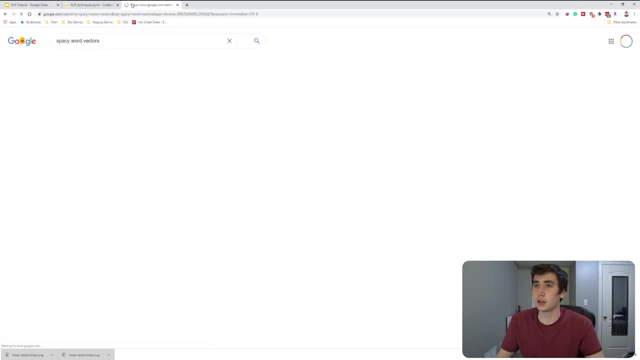 jumping into some Python code to actually show you what that looks like. and I think the best spot to easily utilize word vectors in Python would probably be to use the spacey library. so I, whenever I'm like, trying to remember how to do something like this, you know. 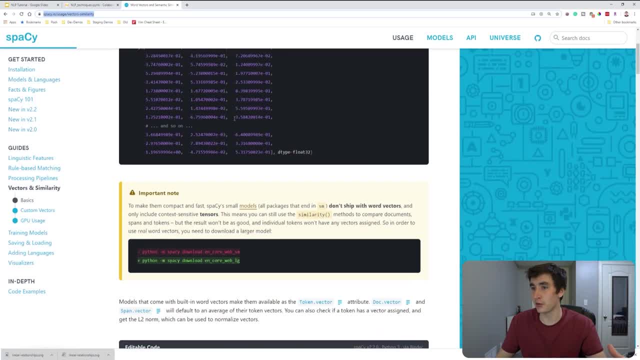 I'm gonna be doing a Google search, finding some sort of information on how I use a spacey and use the word vectors they offer. as I can see, we're probably have to download some word vector model, because we're not gonna train this from scratch. we'll use what, something that's already been trained, and then we can. 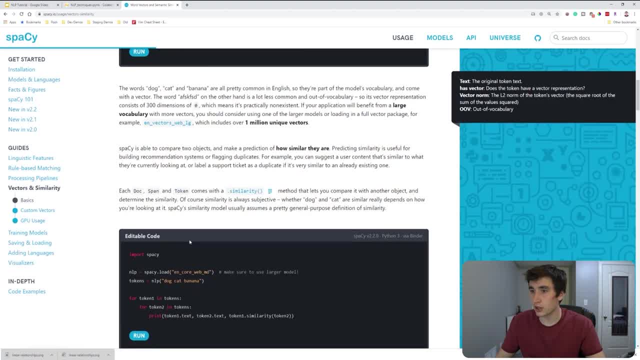 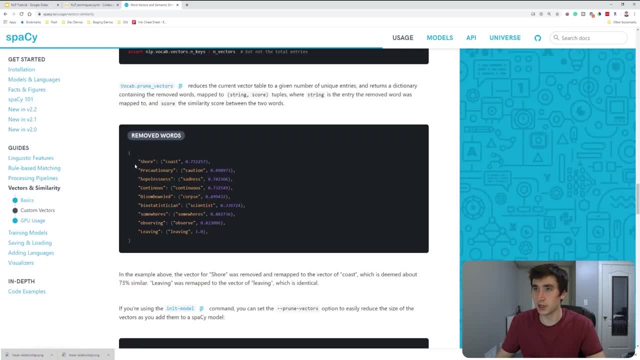 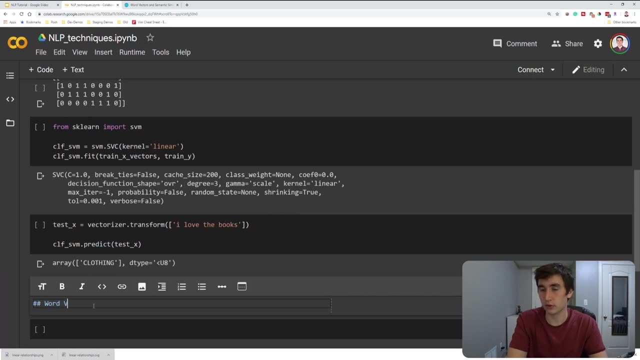 kind of follow along like this. it looks like okay, um, yeah, you can look through here. maybe you look through the actual documentation, but spacey is a good place to start and let's start implementing this. okay, so we're going to need to use the spaCy library before we can use the spacey. 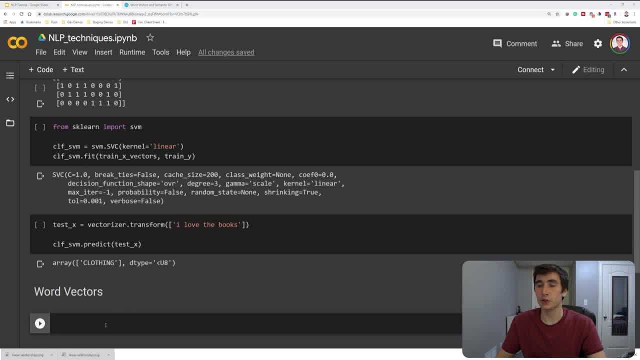 Library. we're going to need to download that language, these, these trained vectors. so that's what we're doing here, and then we're gonna begin with some of the things that we still have to do right now. so, first things first. we're gonna need to use the spacey library. we're going to need to download that language, these, these train vectors. so we'll just have a couple of notes. 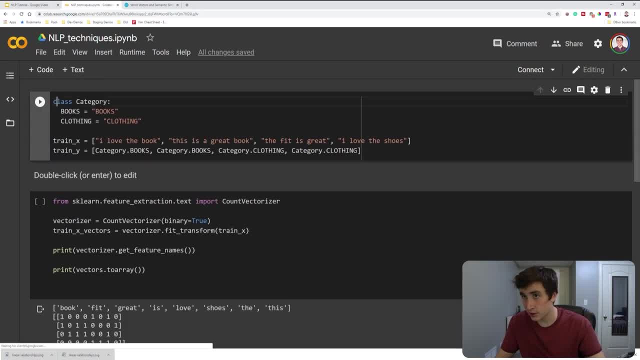 So I already did that previously, So I'm going to just go ahead to the top of my Google collab file, and this also probably should work with a Jupyter notebook or whatever you're using or your, your browser. if you might need to do like a pip, install here. 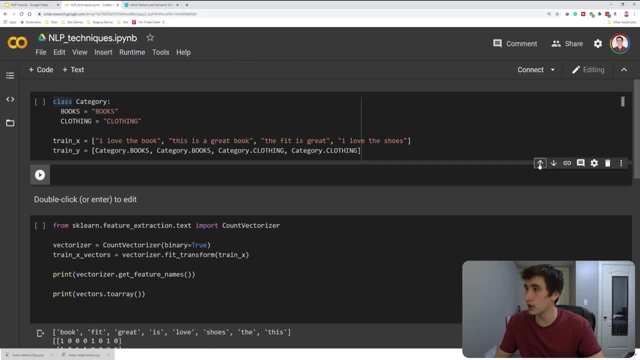 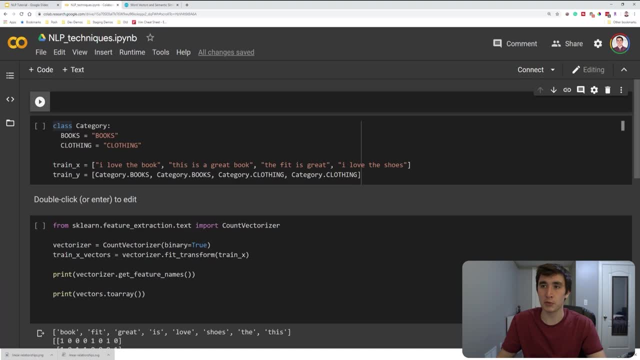 I'm going to insert a code cell and I want to make this above. I'll just do a couple installations of things that I need here, Because by default the Google collab that I'm using won't have the spaCy language model, that or the spaCy word vector. 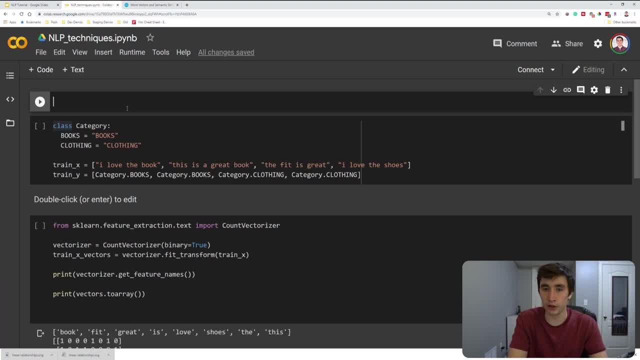 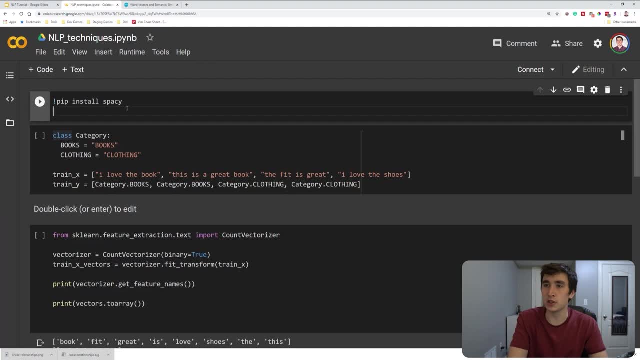 model Embeddings that we need, so we're gonna have to install those. so in here I can do pip, install spaCy. so I think spaCy is already installed, but sometimes you need the most up-to-date version, and I think this will help us do that, and 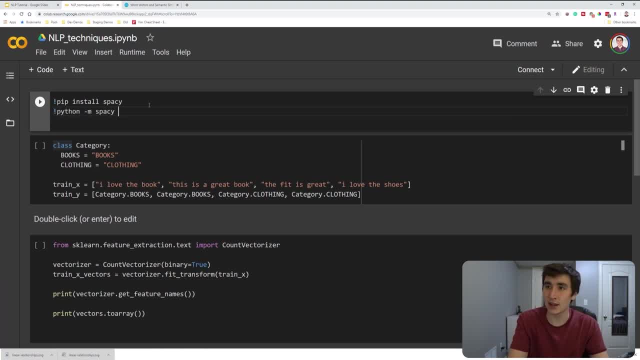 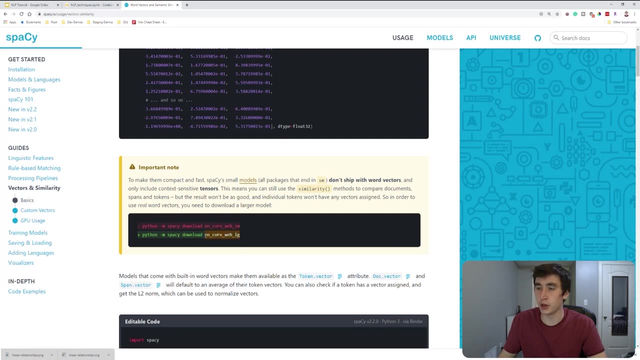 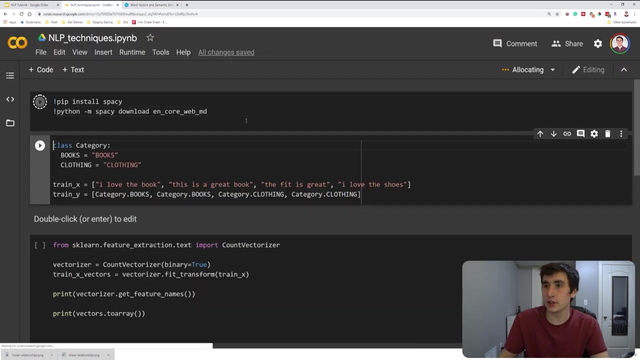 We're gonna do Python dash M spaCy download. We're going to download the medium sized Embeddings But, as we can see in this doc that I walk through, There's also a large model but that might take a bit long to download. But if you want to try some more powerful word vectors, maybe try that large model. Okay, so I'm gonna run this. 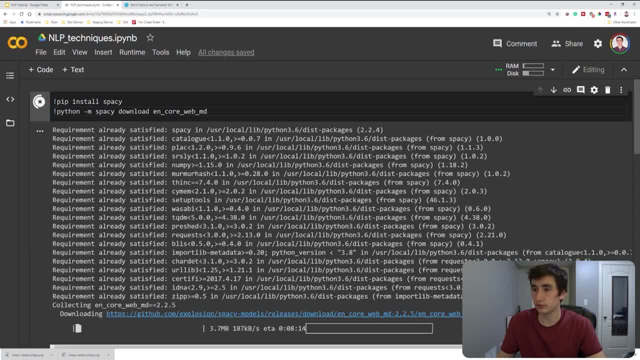 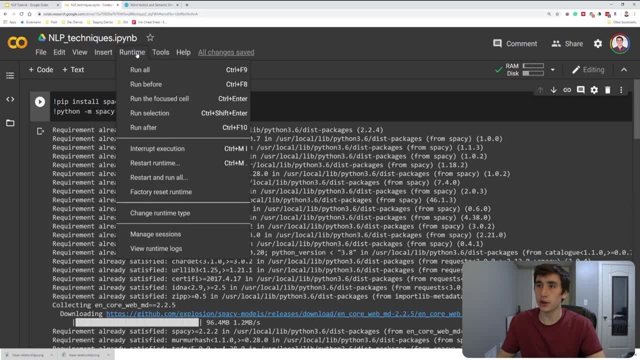 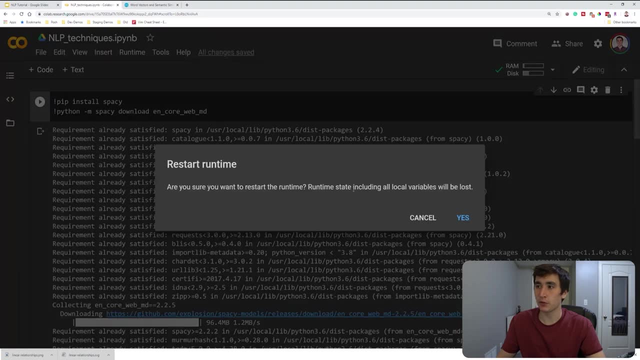 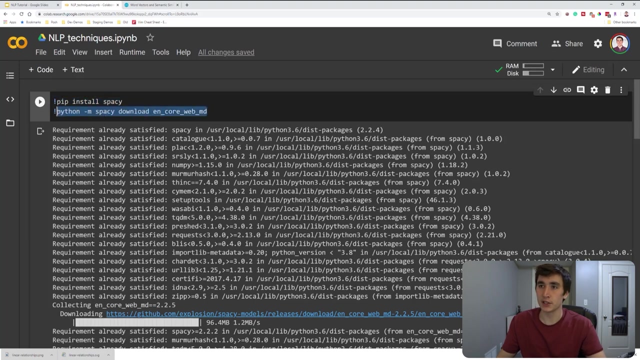 It's downloading. Okay, so we've downloaded it. and one quick note is: sometimes, if you're using Google collab And you do this, you might have to restart the runtime before Changes take effect. like, imagine, you already imported spaCy. I don't think that spaCy would recognize that this model is here unless you restart that runtime. 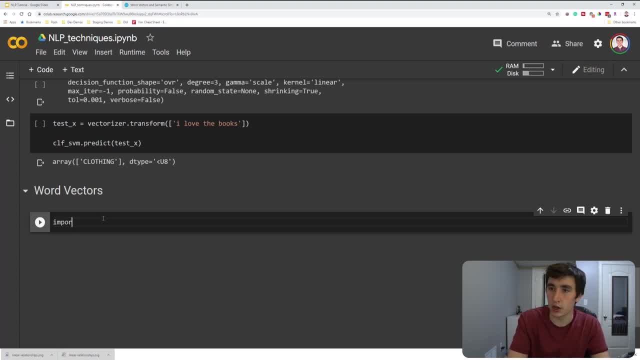 So I just did that to be doubly sure. so import spaCy. That's our first step. Okay, it looks like it imported properly, And Now what we want to do is load in that. we're gonna call NLP That Word embeddings model that I just downloaded. so N core. 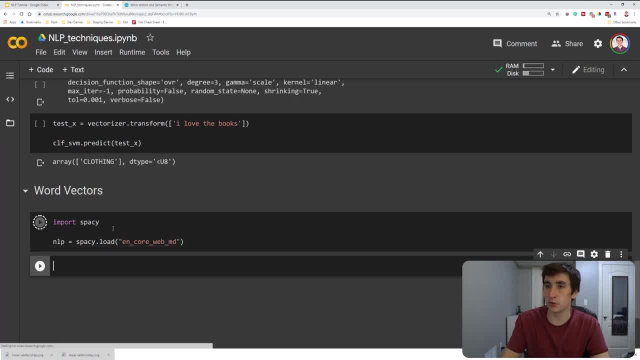 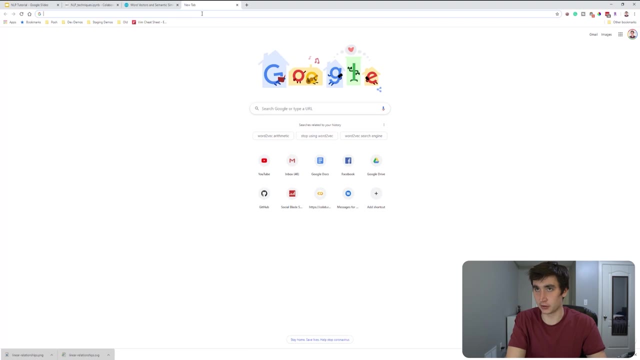 Web Medium size. so let's see if this works. Hopefully it does. Well, they need a load this in once and then it'll stay in memory And like: if you're not remembering how to do this, I always like to remind people. literally just do a google search word: vectors, spaCy. 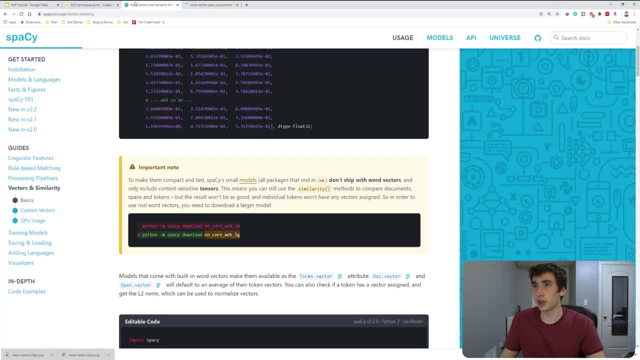 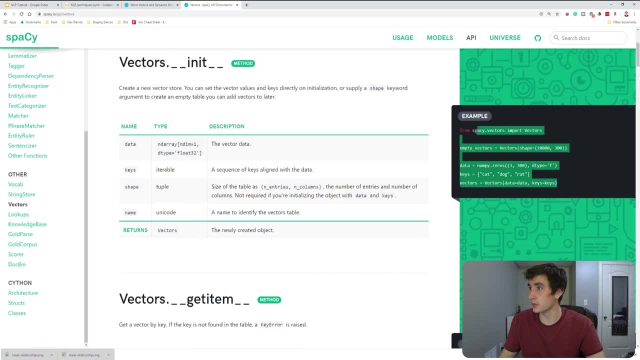 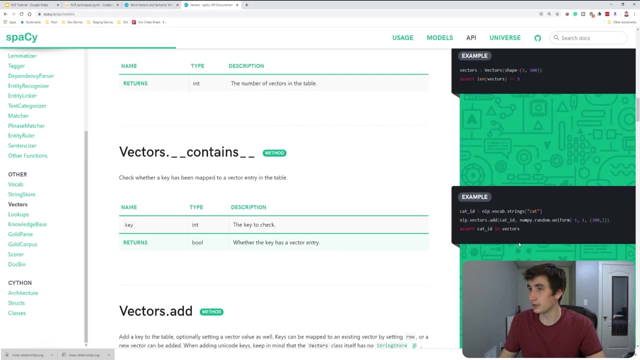 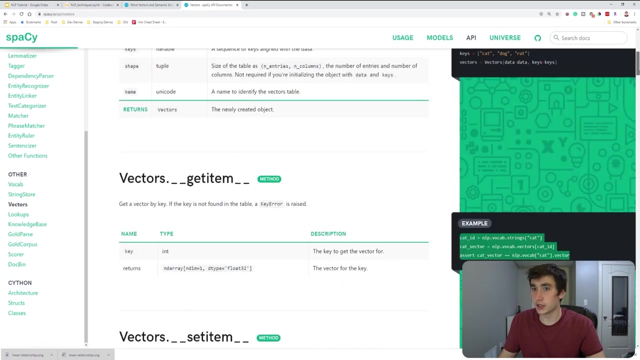 documentation. the article I was looking at wasn't the actual Doc's. you probably actually find the Doc's here and that will give us: yeah, look at this, this gives us some nice examples right there and that makes it a lot easier than trying to figure it out from memory. so let's see, I want to see a actual value. 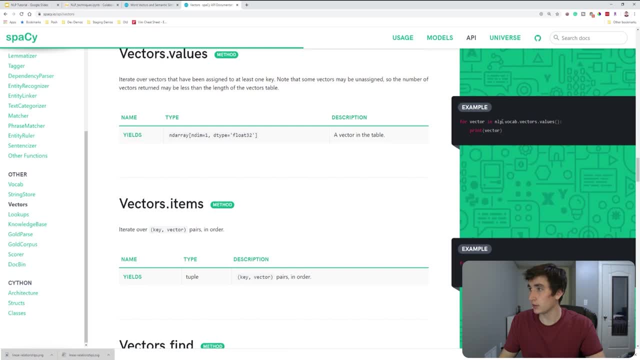 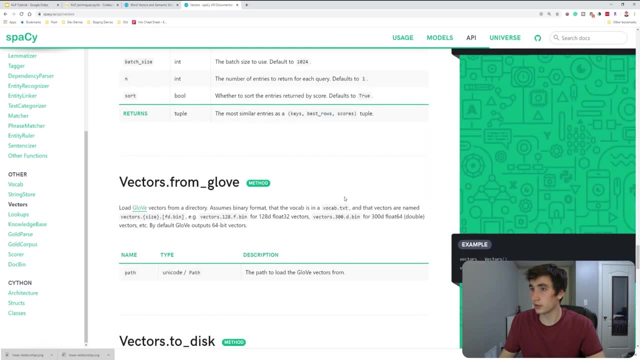 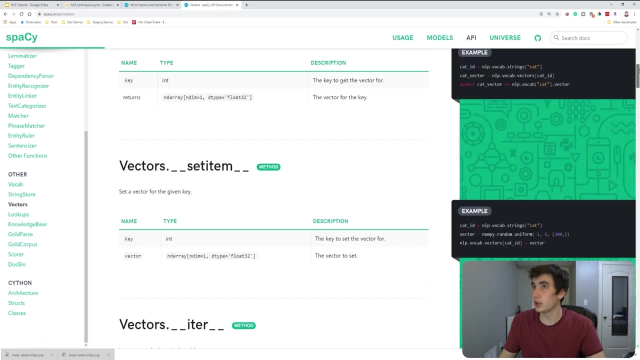 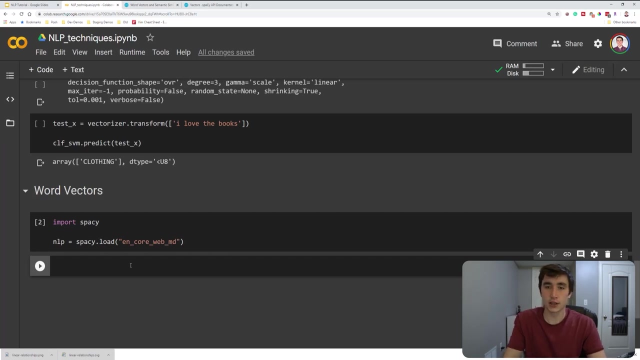 looks like factors or values. I think I can do dot value and get my vector all right, okay. so what we're going to do here is basically we need to take text so we can if we want to use the same text from above. so I'm going to just 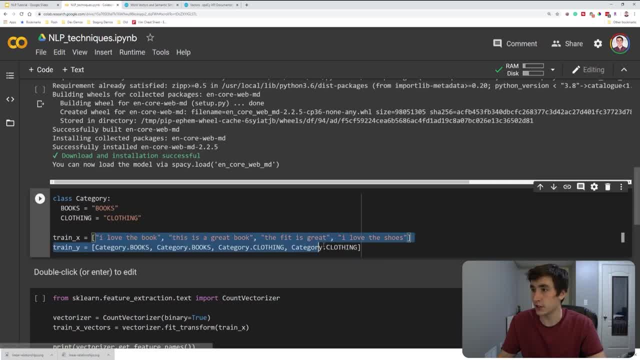 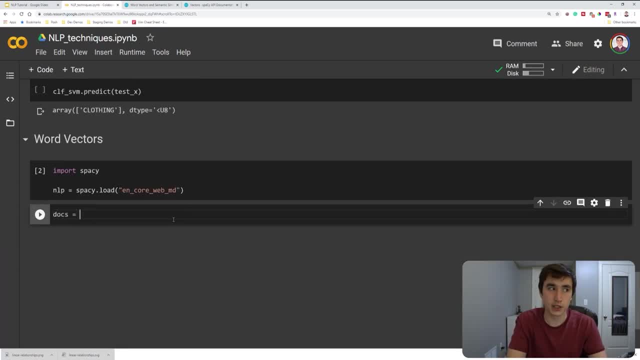 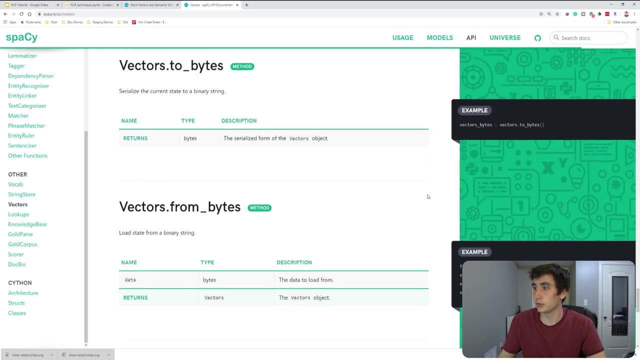 rerun this cell. so now we have all these examples that we were using previously with our bag of words: model, so that's called train X, and now I'm going to say our Doc's equal. basically, we're going to need to convert. if I can see the initialization here: 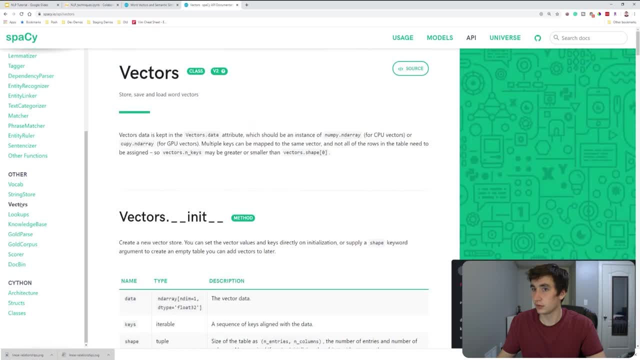 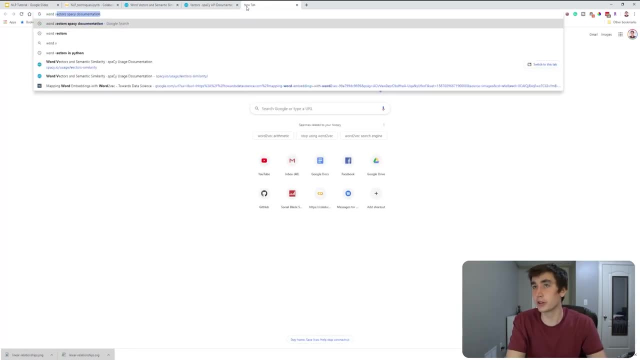 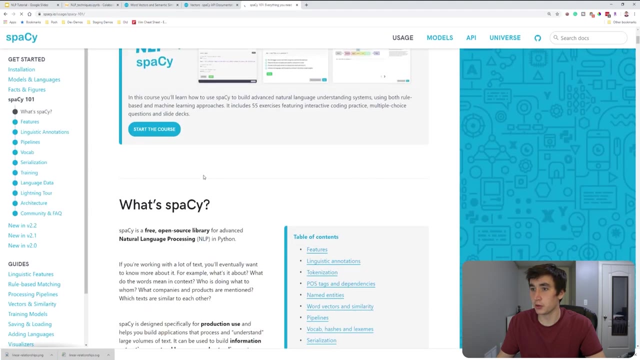 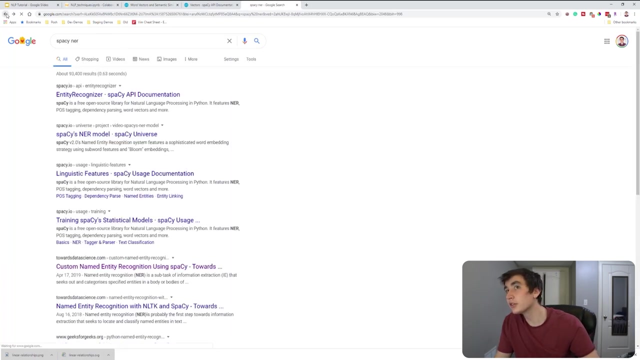 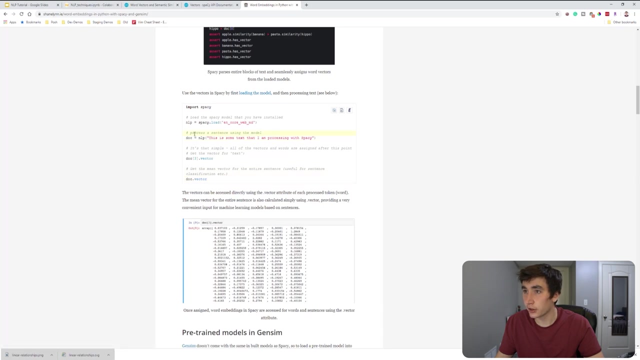 I'm gonna look up one more time word vectors- spacey example. I just want an example to see how I can do things. spacey 101 looks like I already had clicked this next one. no, this one right here, so let's try this. okay, look at this. yep, there we go. this is nice. it's showing us how we can make. 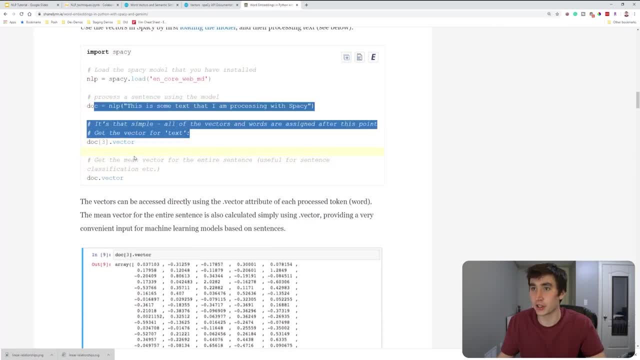 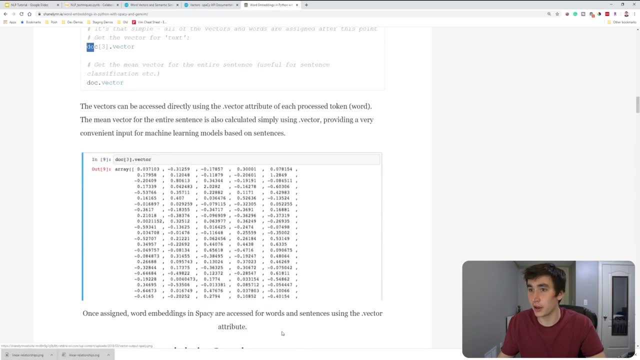 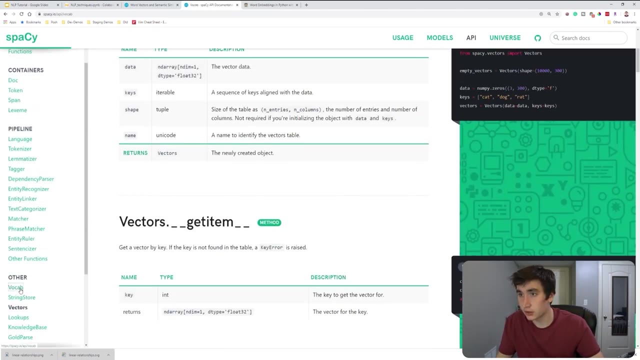 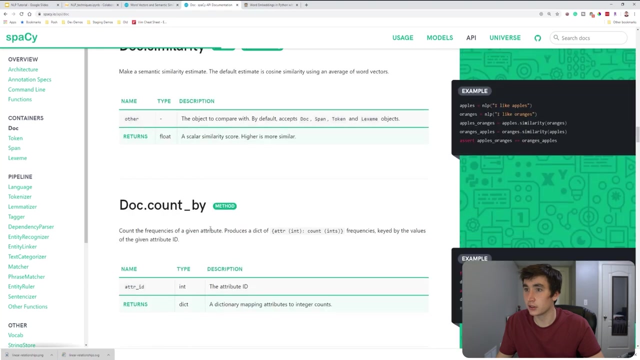 this a little bit bigger so you can see this is showing us how we can get that vector. if we pass in doc NLP do vector, then we get a vector representation, did that? let's see? maybe the doc container had the information here in the doc's. 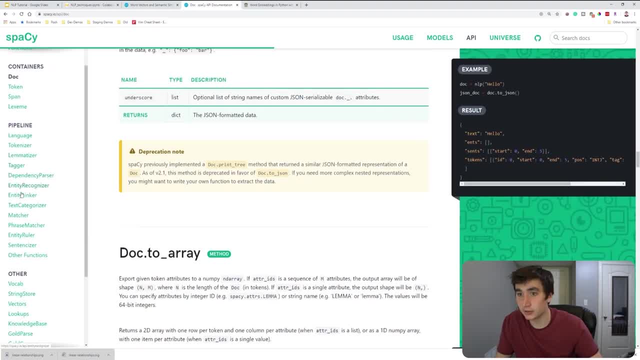 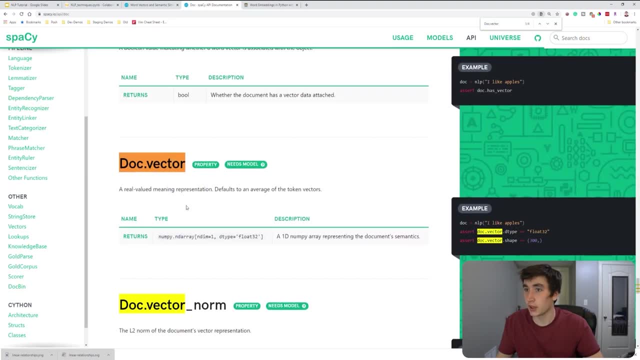 vector, vector, vector, vector. I want to find it here. okay, here we go. yeah, a real valued meaning representation defaults to an average of the token vectors. so basically, if we do NLP of our phrase and then do dot vector, it's gonna take all the individual word, word embeddings and 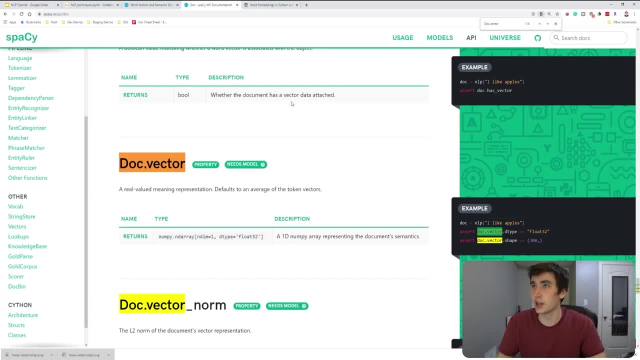 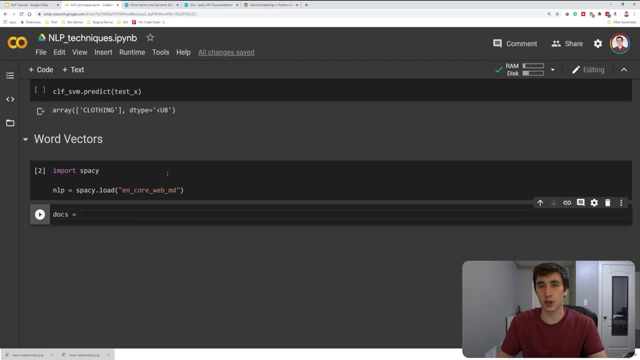 average them together. so that's, I think, what we ultimately want if we want to build a model around this, and also to note that these word vectors are usually hundreds of. they have, you know, a dimension 1 by like several hundreds. so they they're pretty big, but they kind of have to be to capture the information we 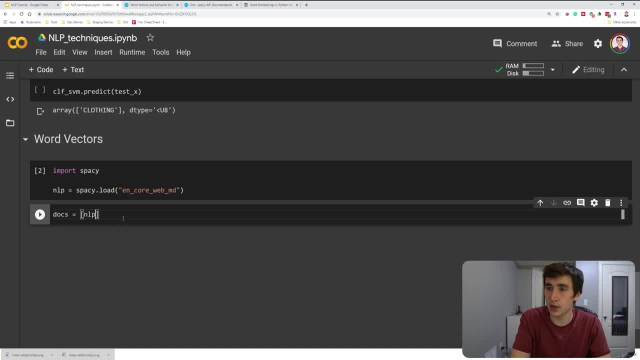 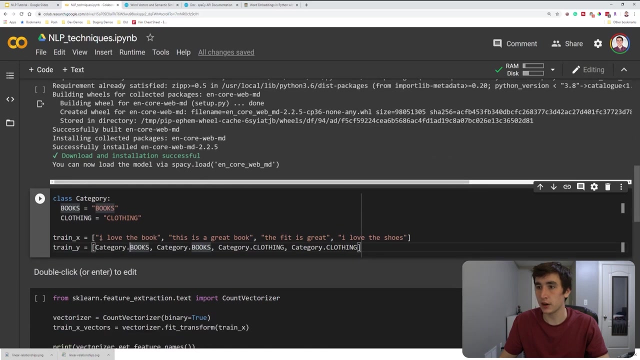 need. okay. so docs are going to be nlp of text for text in our train x that we just defined and now each of these items in this docs list is a word vector representation of our sentences that we defined above here. so i love this book. this is a great book. fit is great. i love the shoes. 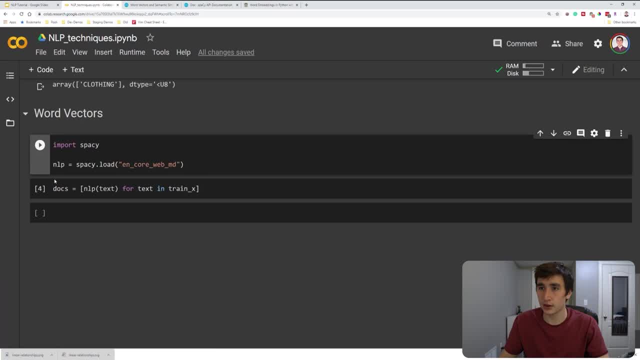 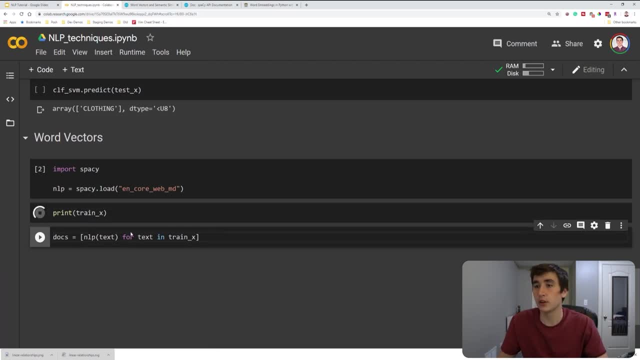 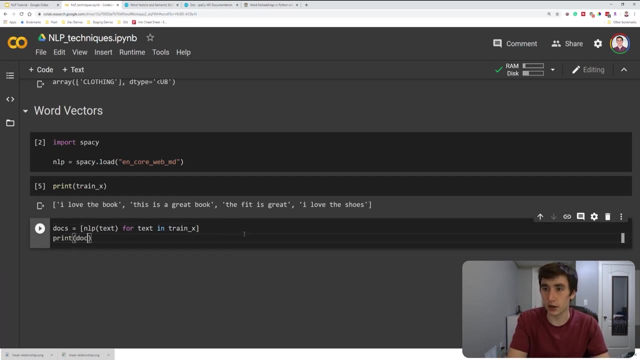 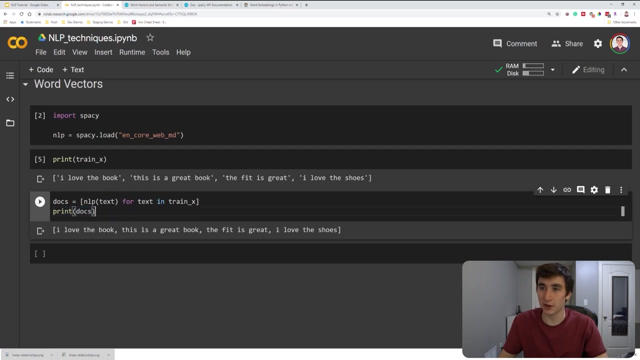 and just so you have that here, it might be helpful for me to just print out train x so i can remember that. uh, okay, so that's what we're ultimately converting. so now, if i print out docs, you're going to see that it's um, i guess it keeps the. uh, if i print out docs, dot vector or oops. 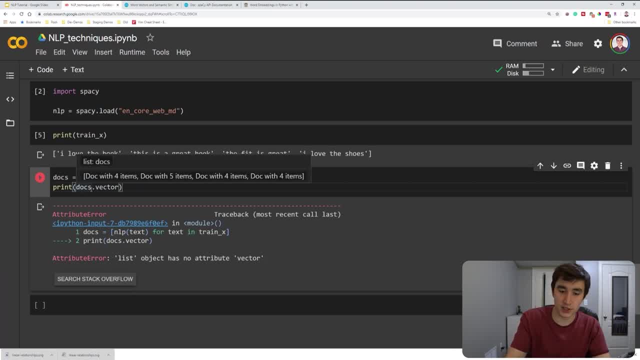 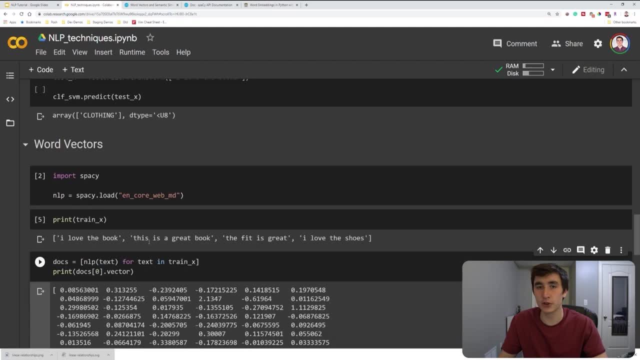 if i print out, uh, let's say, the first docs vector you're going to see, this is the word embedding representation, the average word embedding for each of the words in. i love the book, so that's cool. we did that pretty easily using spaCy and a couple lines of code, and now 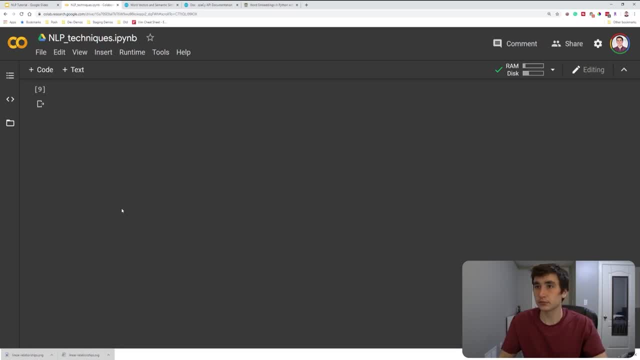 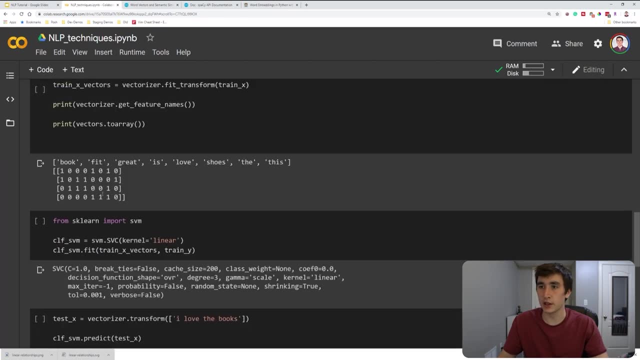 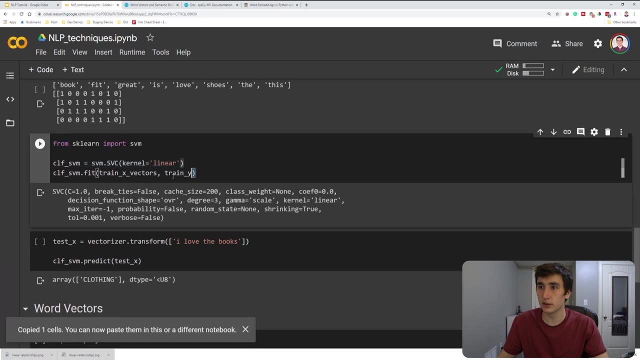 that we have this. okay, so now that we have this, let's build the same model that we built for the s uh- the back of words model, for the spaCy model, so we can define a classifier again, and i'll define it like this: so we're going to define a classifier, i'm going to give it a. 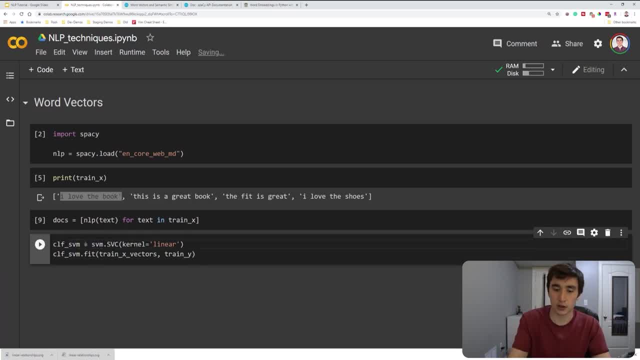 slightly different name. i'm going to just say svm and i'll give it wv for word vectors at the end, just so we can tell these apart. and we want it to not fit to the train x vectors anymore, but we want to fit to. uh, we'll define a word vector. 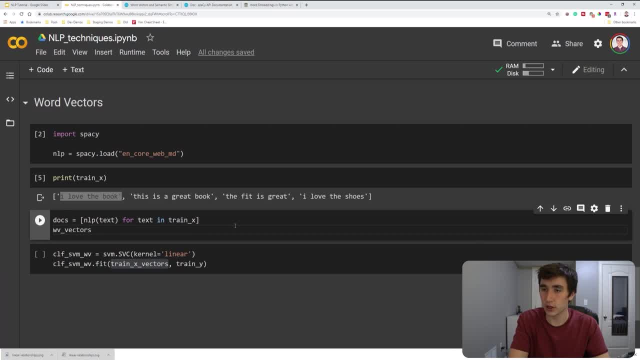 word vector vectors. we'll say i'll just call them train x word vectors, just to separate a little bit from the other word vectors. and that's going to be a dot vector, x dot vector for x in docs. so we're just getting all those as a list. so now we're going to pass that into our fit. 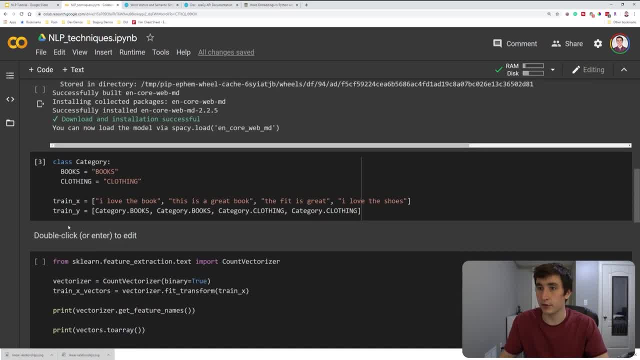 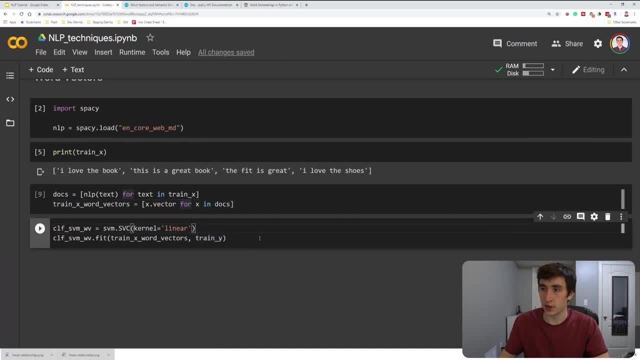 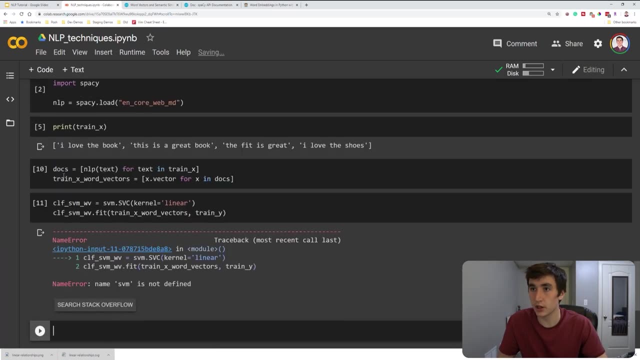 and the the y labels stay the same as above: books, books, category. uh, clothing, clothing, all right. so let's see what happens here. we're fitting this. run this again, run this again. svm is not defined. okay, I need to re-import SVM from scikit-learn. 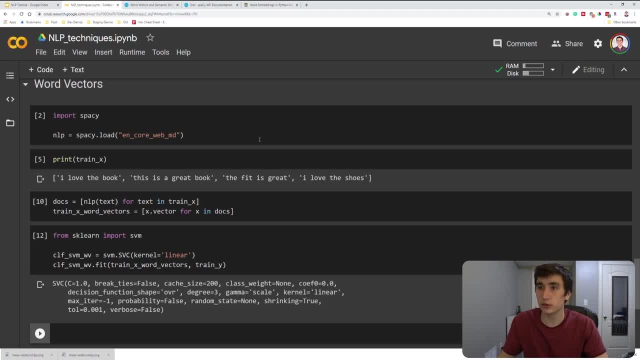 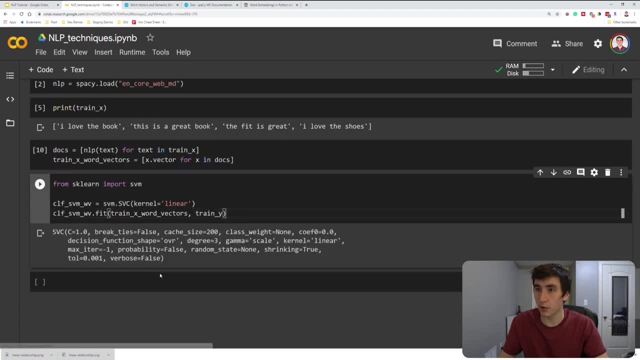 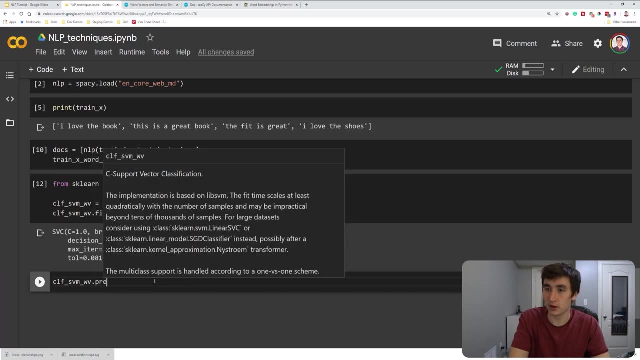 Cool, I think there was one other thing I needed to re-import. Nope, I think we're good. Okay, so we have our model. and now what happens if we try to predict some novel utterances? So to do this, we can pass in NLP of a phrase. 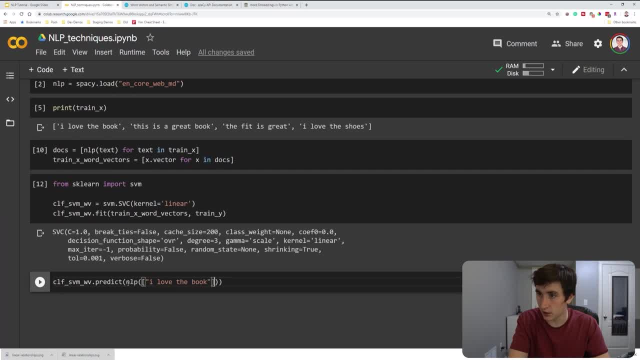 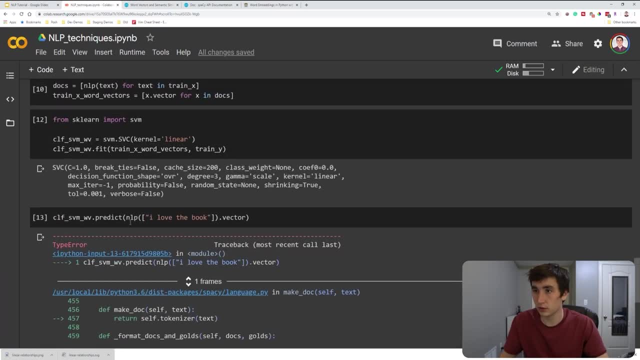 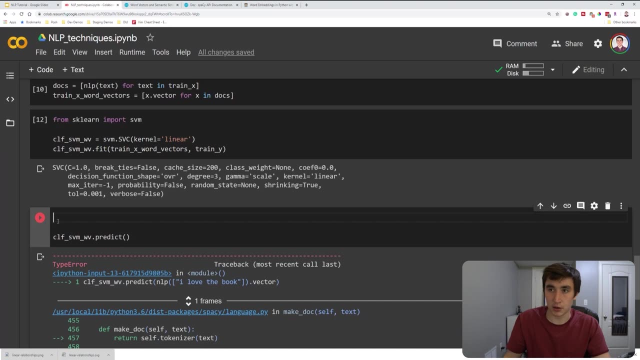 So how about I love the book? We'll just do that again here, and then we'll have to grab the vector for that. What's gonna happen here? Oh, it's trying to do too much in one spot, So instead of doing that, I'm gonna say testX wordVectors. 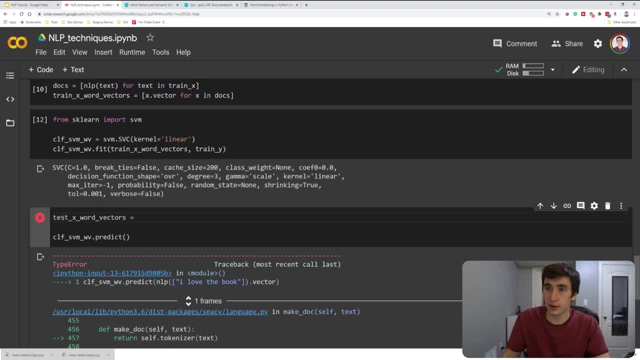 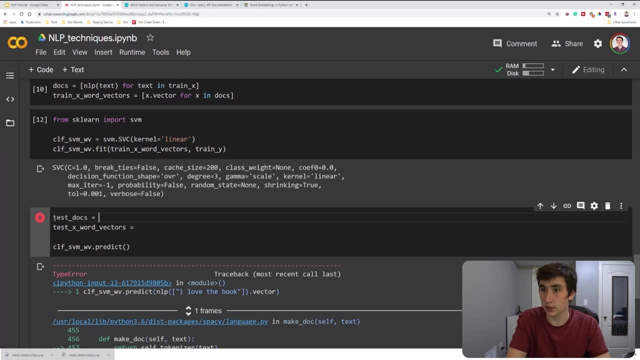 equals. well, we'll also define a testDocs. That's gonna be equal to: oh, I'm trying to do a little bit of math here. I don't know if that's gonna work. Okay, I don't know a lot here. 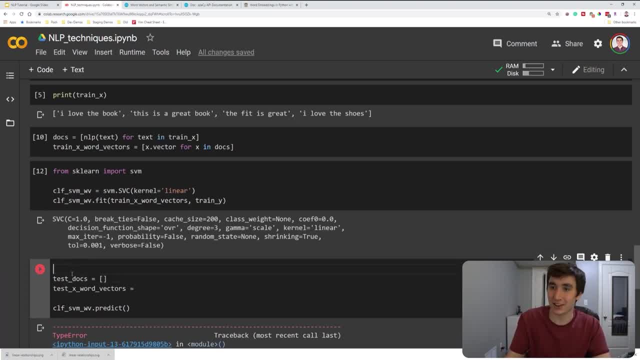 Sorry, I feel like this is simple, but as I do this live, it's sometimes tough. So test is gonna be equal to is equal to a list of words. So let's say I love the book TestDocs. now is the NLP representation of testX. 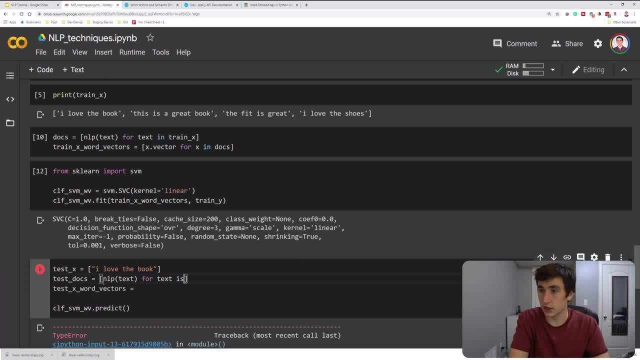 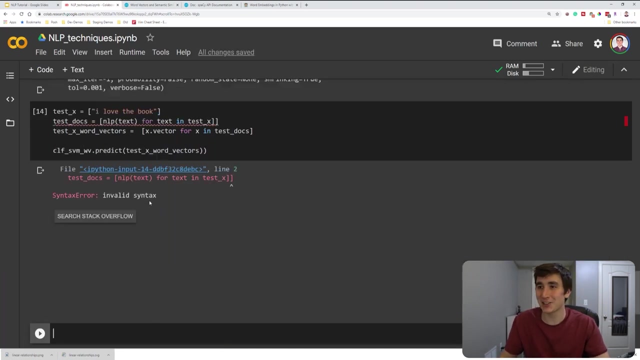 for text, for text, in for text in testX. And then finally, the word vectors are gonna be xvector for x in testDocs- Cool. So now we can predict testX word vectors- Cool. Sorry, I was trying to simplify it too much. 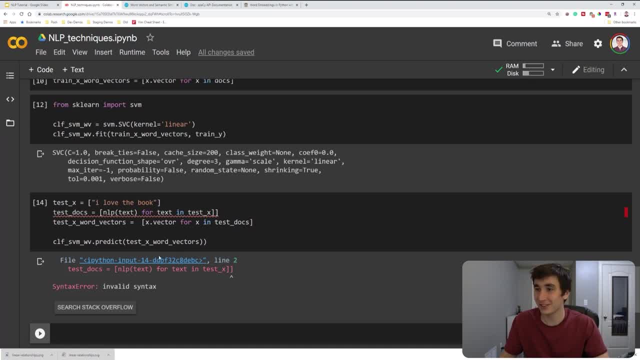 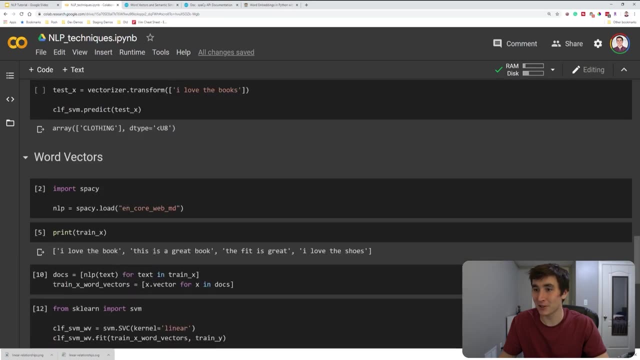 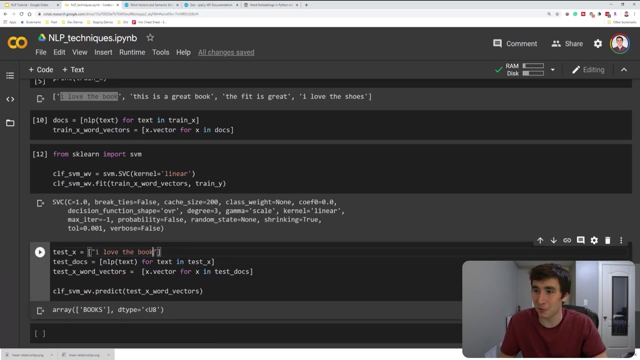 And, as a result, no Oops, So close. How did I keep getting double things here? Okay, I love, the book Works as expected. I mean, that was an exact take from here, So that recognizes books. But now let's try to find the power of word vectors. 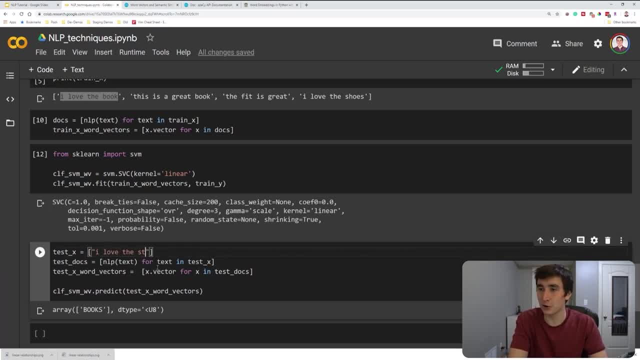 And let's type in something like: I love the story And we're hoping that story and book have a similar word vector representation, so that when we do this averaging, when we do this NLP text which basically averages all of those word embeddings, 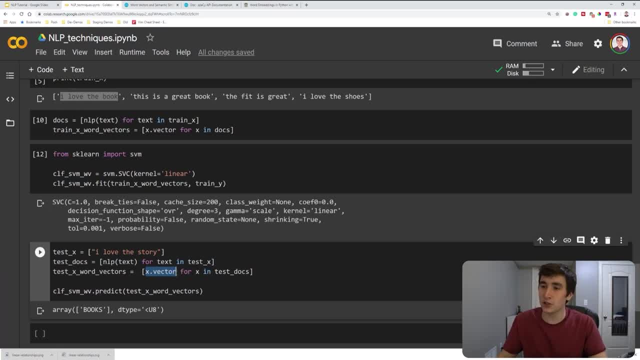 together and actually get the vector value of that averaged. embedding that, we get a books classification again. There we go. Look at that. I love the story. It's books as well. And now let's try testing out some things for clothing related. 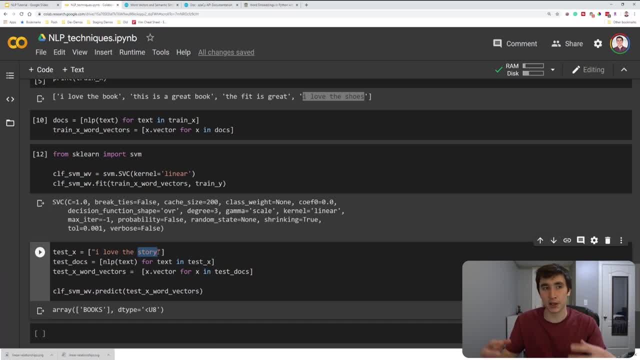 So I love the shoes works. So if this is properly capturing the semantics, you should be able to say something like I love the hat, And hopefully that says clothing. Look at that Cool, I love the hats. That should also be clothing. 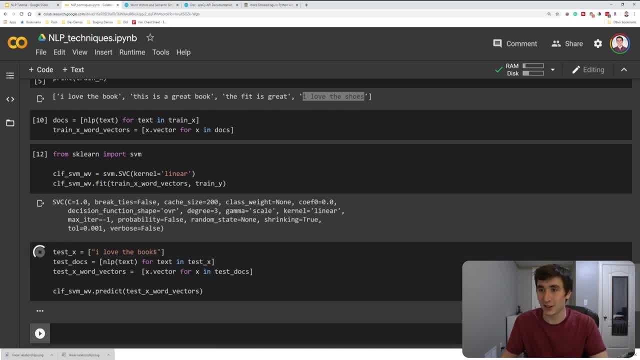 I love the books, even though we haven't seen books exactly. And now it knows that book and books are more related because it's seen those And similar context windows. And, yeah, there's all sorts of cool stuff that we can do with this. 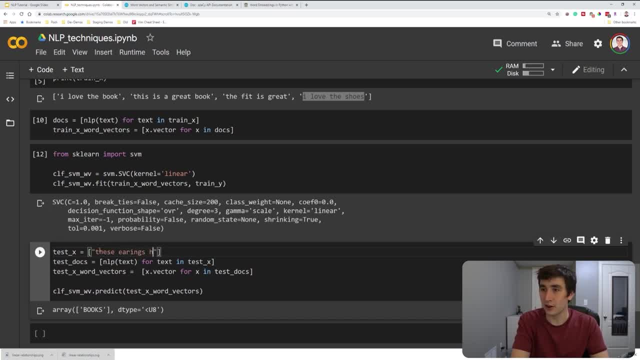 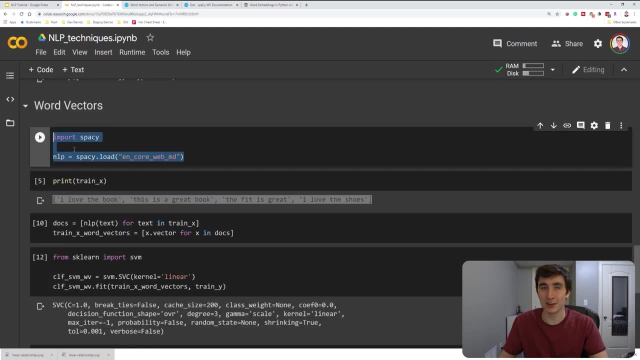 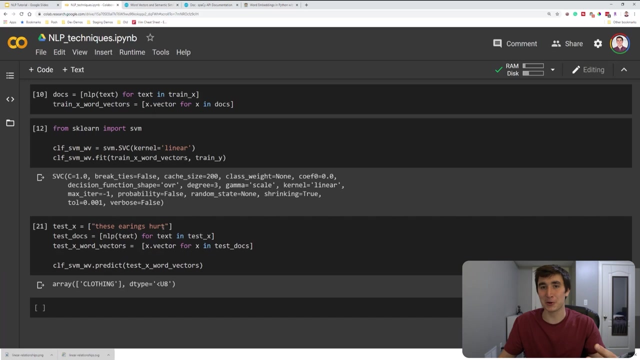 You know, these earrings hurt or something. And already, with just four training examples, because there's so much power baked into the spacey word embeddings, the word embeddings in general, even just with this medium sized model, I think it's a very interesting tool. 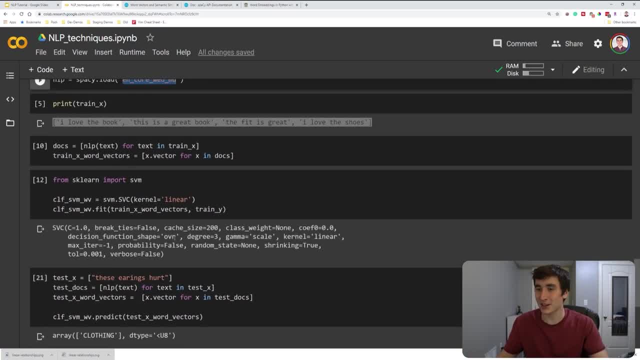 And I think that we can already predict a lot of things correctly just by knowing that you know. semantic space And I think there's like word vectors are so cool and this concept is so cool that we can do so much with language like this. 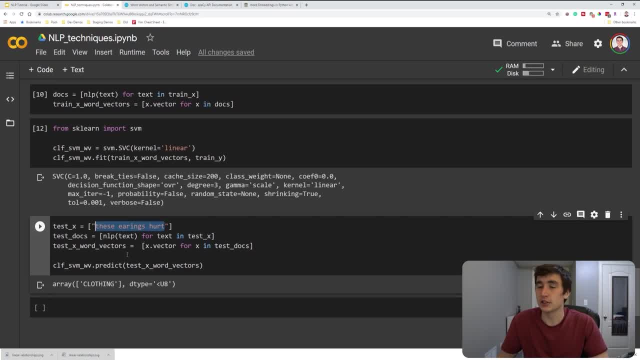 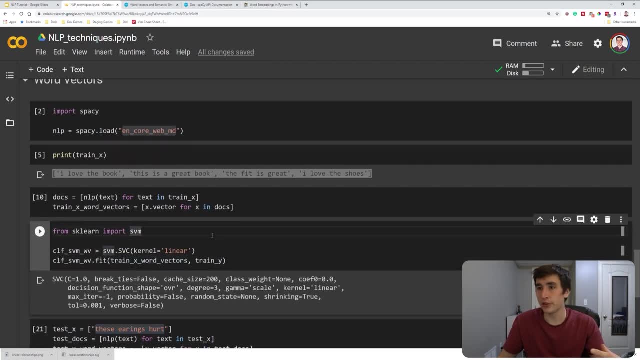 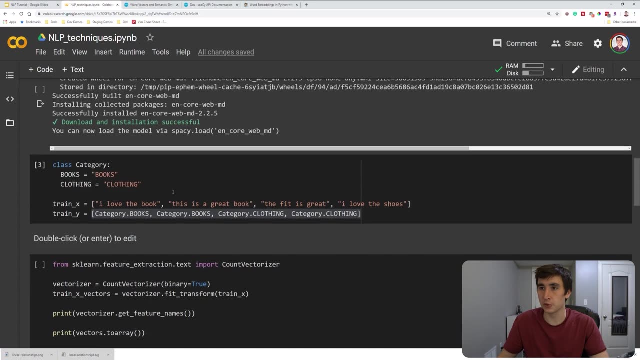 So this gets me really excited. I guess, before I end this little section, there are some drawbacks to word vectors. I think one thing you'll see is that it worked out pretty well for us because we only had two categories, We only had books and clothing. 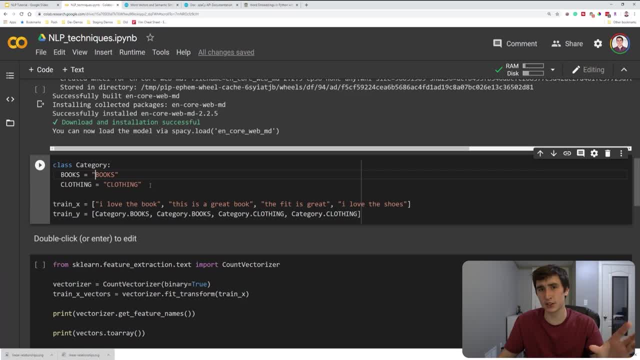 But if we were trying to use word vectors by themselves- and I think at the exercise at the end of this tutorial, we might see this. If we were to say use 10 different categories, instead of these phrases being like four words, they were like 50 words. 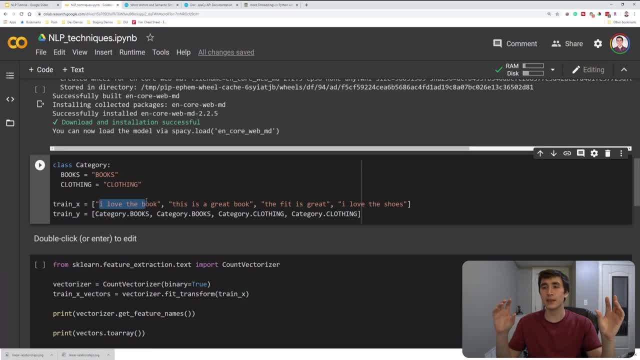 Then when we're trying to capture a embedding for the entire sentence, we're averaging together like 50 individual word vectors And the actual meanings of all these individual words might get kind of lost in that averaging process. So sometimes they're not quite as precise as maybe using bag of words in that case. 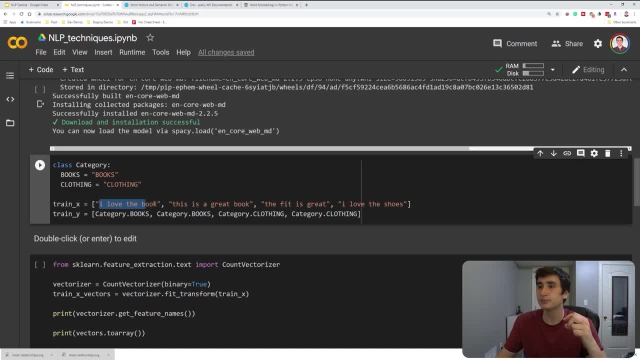 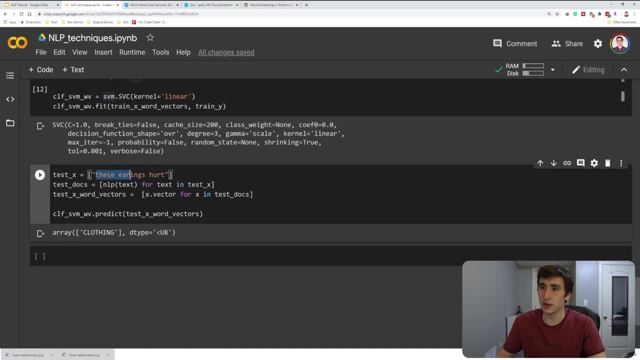 because things get kind of mixed together. Another drawback of the standard word to vector word embeddings is this is a little bit different than the context that we're worrying about. But imagine we were trying to get some sort of meaning for the word check. 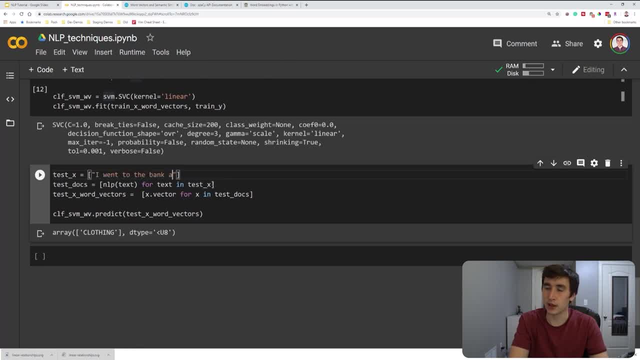 So I went to the bank and wrote a check. So the check in this case is going to have a specific meaning. But if I also had a check, I would have a specific meaning, So I would have another word embedding another sentence. that was: let me check that out. 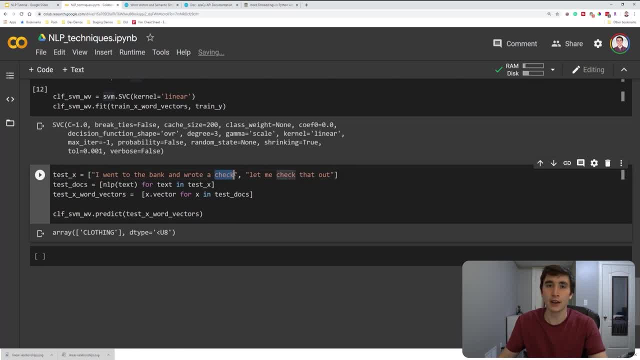 Check- and let me check that out- is very different than writing a check, But the word vector is going to be the same for both of those. So you do get for words that have multiple meanings, you do get a little bit of messiness. 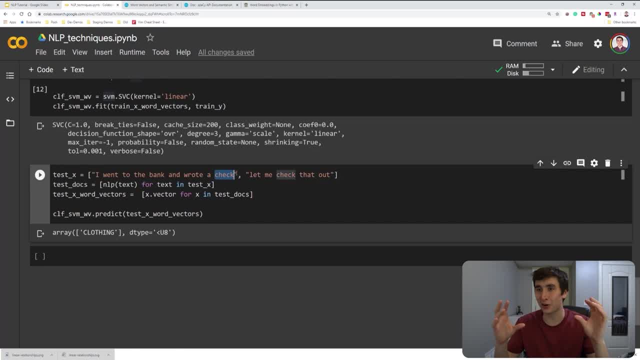 because both their meanings are kind of captured in the training process and ultimately part of those meanings are probably lost. So word vectors are. they're very cool, pretty powerful, but they don't solve everything and ultimately left a lot of room for improvement. that it was ultimately. a lot has been developed recently. 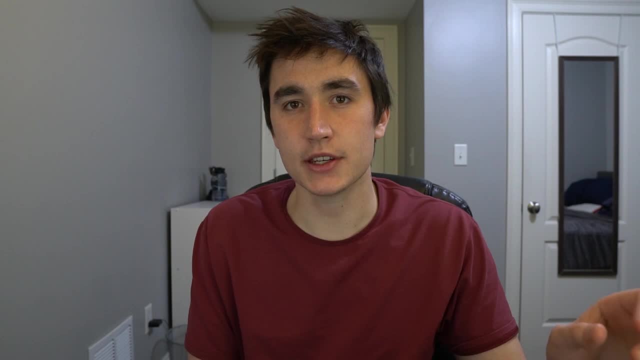 as I kind of mentioned at the start of this tutorial. All right, in this next section of the tutorial we're going to kind of do a rapid fire overview of a bunch of different NLP techniques that are good to add into your NLP toolkit. 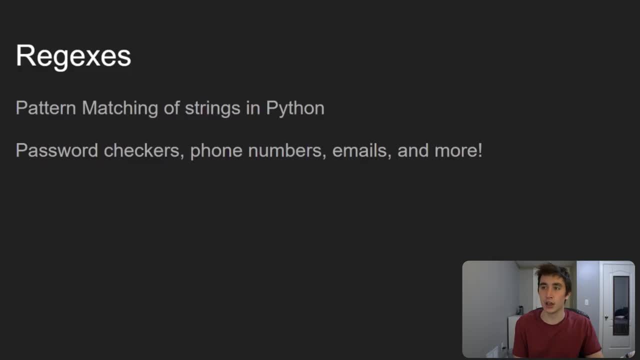 And so the first technique we're going to look at is using regexes. So regexes are pattern matching of strings and they're not a Python specific concept, but we can definitely effectively utilize them in Python. So, real quick, I'm going to start with a quick overview of regexes. 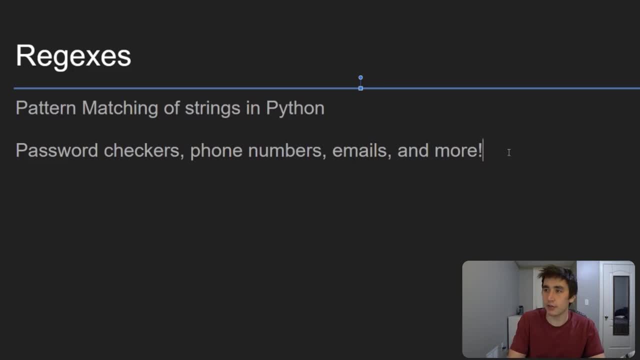 Basically, the way you can think about them is you could have all sorts of different types of phone numbers, So like 1231231234 would be a valid number. you know, maybe a different set of numbers, That's the same format. 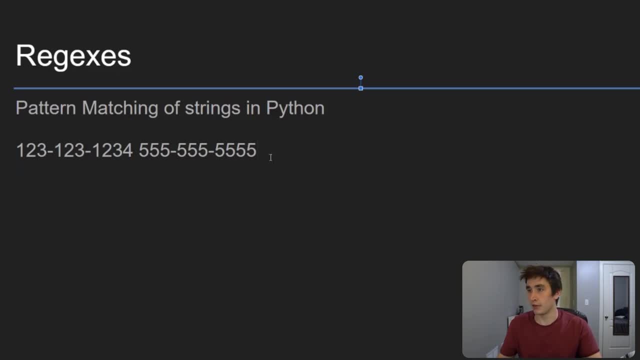 5555555555 would also be another valid phone number. Maybe you want to write it a little bit differently and maybe you do like plus one dash parentheses: 123-123-1234.. These are three different ways to write a phone number. 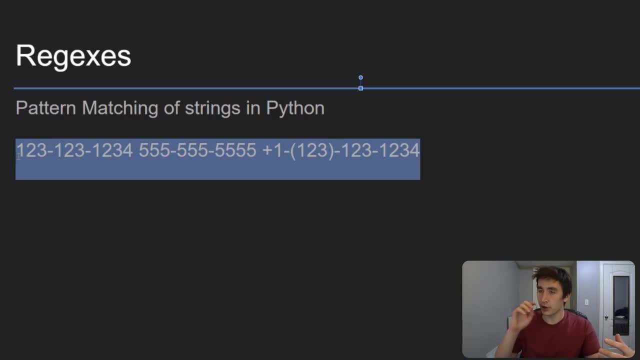 but they're all like technically valid ways to go about it. So one one way we could use regexes is pattern matching on, like figuring out if something's a telephone number or not, And so like. in this case, one thing we could see is that it has three digits followed by some sort of punctuation, or maybe no punctuation, followed by three more digits. 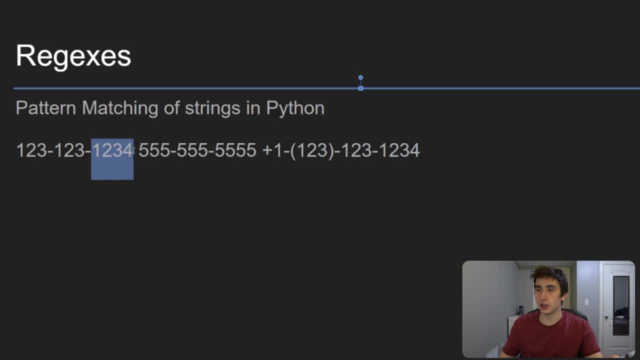 followed by four digits, And basically we could define a regex for that And similarly for this. like last one, you could define in your regex that it could have a plus one plus some number optionally, And so regexes allow us to easily capture these different types of patterns and effectively add this into kind of like code that we're writing. 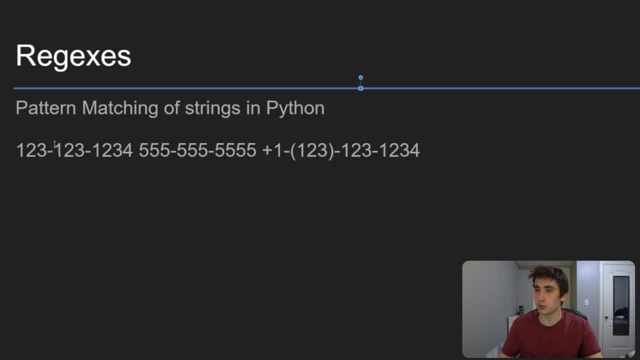 So you know phone numbers. writing regexes for phone numbers is one thing. You also might have like a password checker where, if you're like logging onto a site and they say, oh, you need one symbol, one character, one uppercase character. 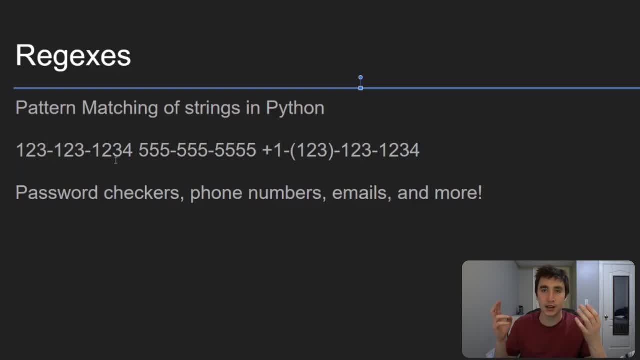 and a number in your password And it has to be plus 10, 10 digits or more. A regex can help the people implementing that site on the back end make sure that your password meets those specs. Email formats is another thing. 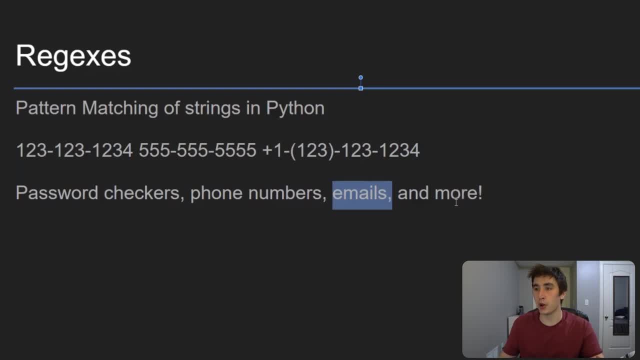 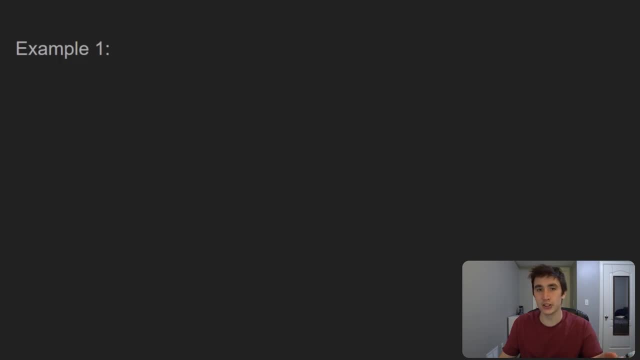 So I think the easiest way to get into regexes is to just start right away with an example. So I'm going to say, as the example is, that say we want to match a string that starts with the letters A and B, and they can have in between, in the middle of the string. 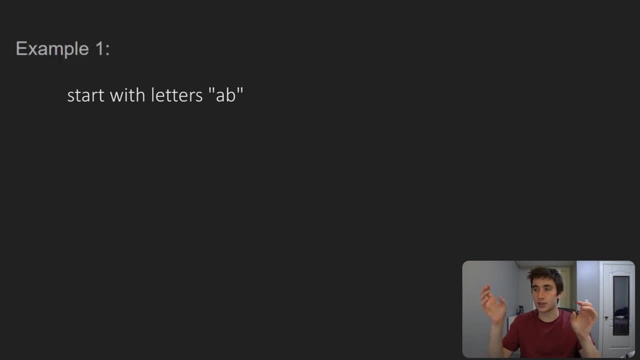 it can have any number of characters. It doesn't matter how many characters it has, as long as there's no white space. So we don't want any white space in what we're trying to match, And then it needs to end with the letters CD. 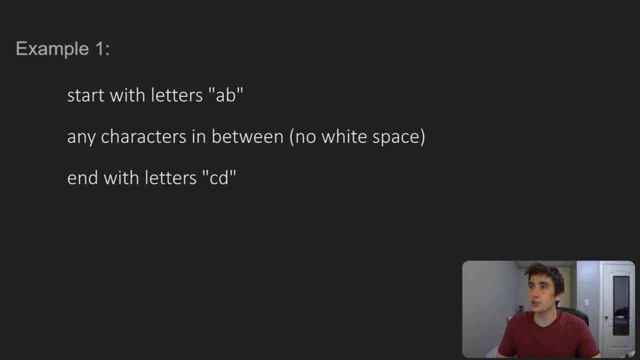 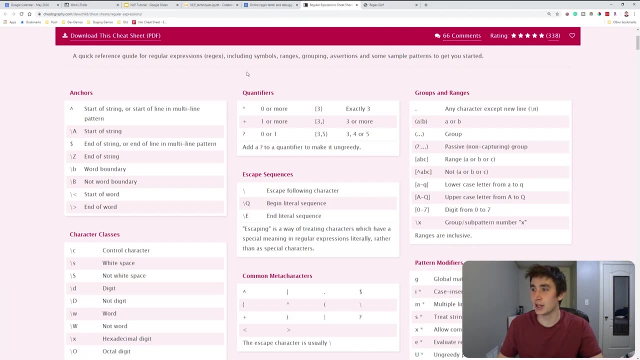 So whenever I'm going about working on a regex, I usually will start looking at a like regex cheat sheet to just remind myself of what we can do with regex. So I'll link this in the GitHub page for this tutorial. but a page like this has all sorts of useful tidbits. 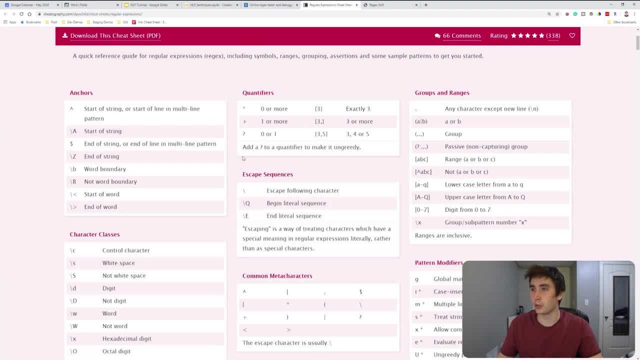 Um, so, ultimately, what we're going to want to do is, uh, have like exactly A or B, So, or exactly AB, which is going to be a group followed by any number of characters. So, if you see it, there's this special dot or period, that's any character except new line. 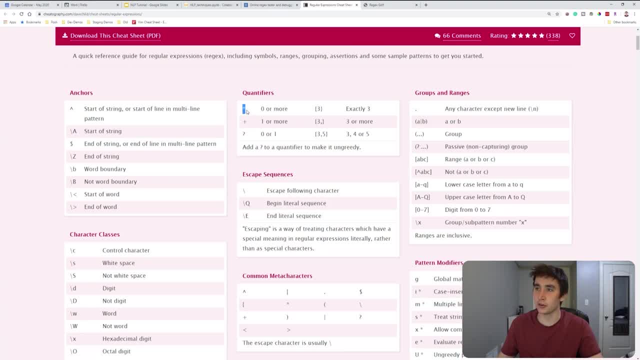 So maybe we will utilize that. And then there's these quantifiers. So if we uh could have zero or more, one or more, um zero or one, we can use these quantifiers, Um. and there's some other stuff too. 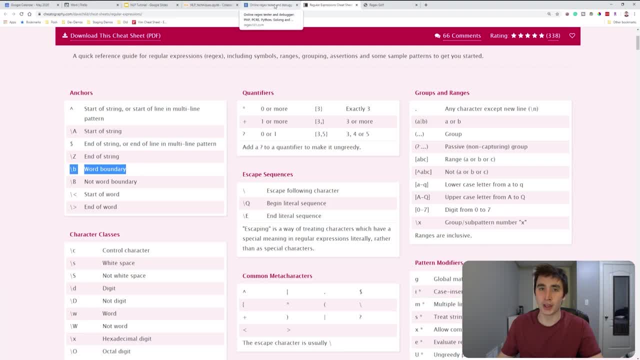 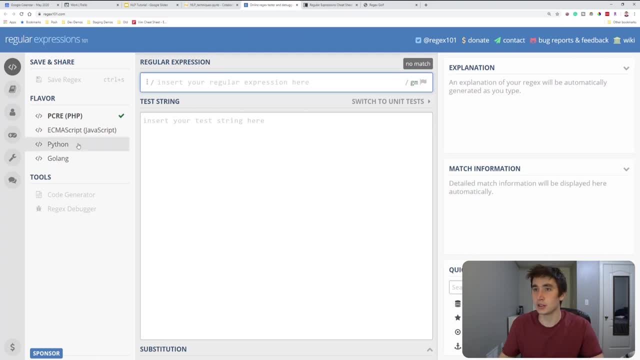 like word boundaries is useful, but let's try to write a regex for the case I just said. So I'm going to the site regex101.com and it actually has the flavor you can test. So I clicked on Python. So what I said is it needs to be AB to start, followed by any number of characters. 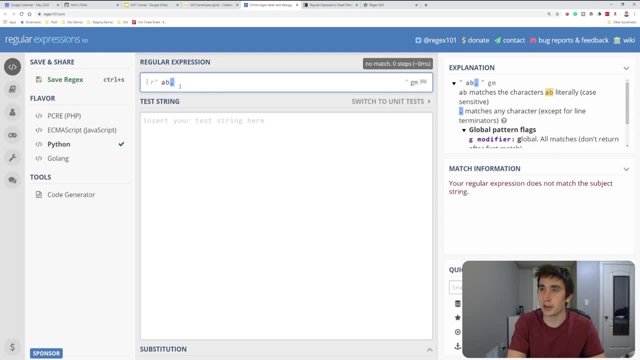 which is period, And then it doesn't matter how many there are, So it can be the star. That means, uh, it can be zero or more, followed by CD. So that's like the basic implementation, As we can see if I do AB. 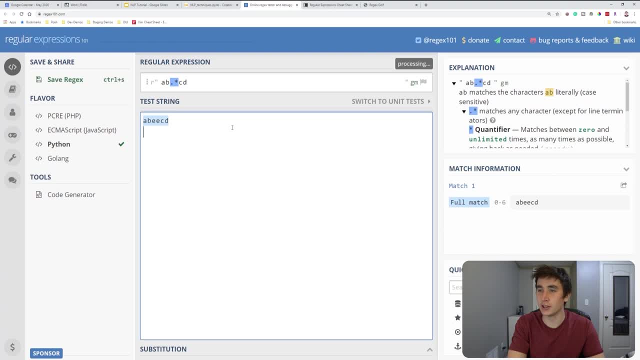 EECD. um, it matches, If I do BA, uh, all of this and followed by X or something. it's not going to match that one because it doesn't start with AB and it doesn't end with CD. Um, continuing on. 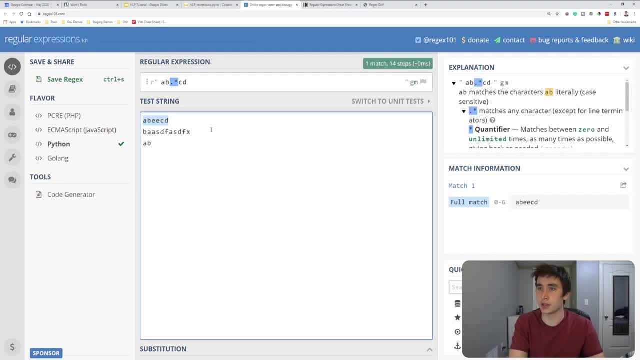 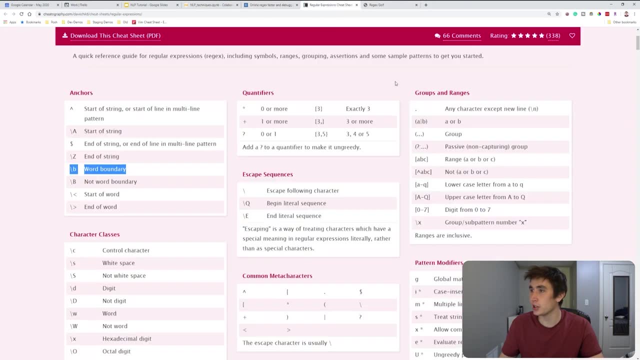 I said that there couldn't be any white space, So let's see if AB space CD works, and that does work. So now we need to fix our regex to disallow white spaces. Going back to our cheat sheet, we see that there's this, not character. 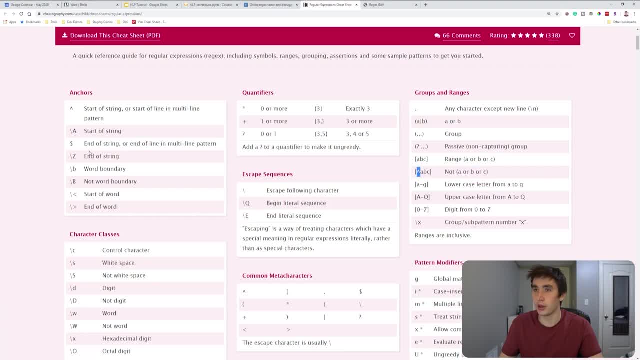 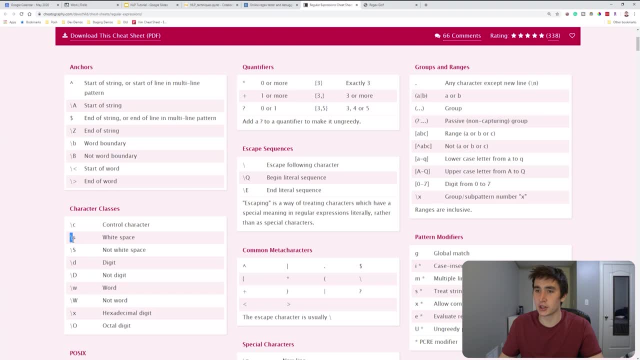 not A, B or C. So we can utilize that along with um white space, this character class, So we can do um forward slash, um forward slash S to to do the white space. So we're going to do in this brackets: 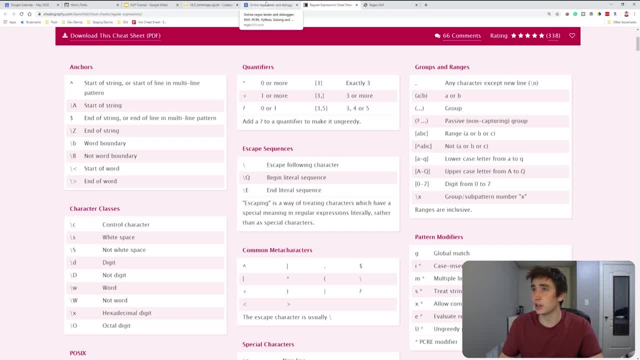 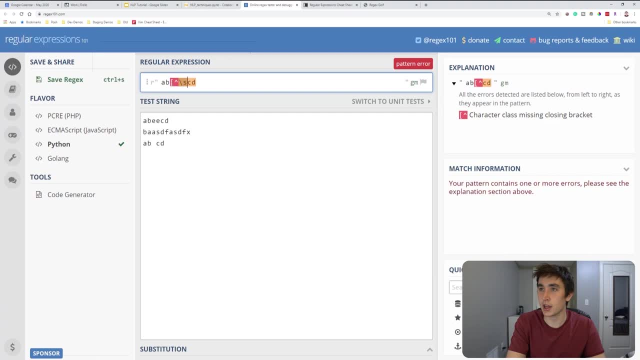 we'll do not white space, So let's go back to here. So instead of dot star, we're going to do brackets, not slash S close bracket and then one or more of that, And so now we see that this works. 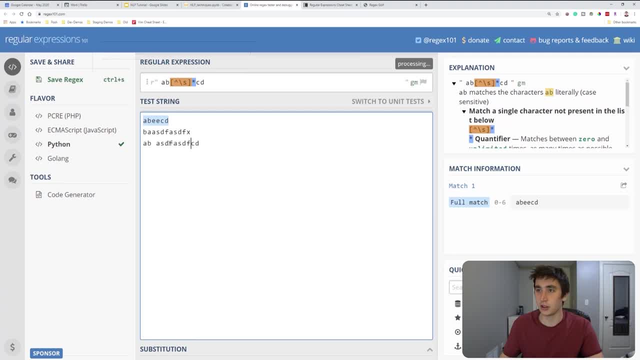 but this one now doesn't, because it has white space in the middle. Uh, if I remove that white space, it's now a match. That's pretty cool. Uh, one thing to note here is I could do something like: uh. 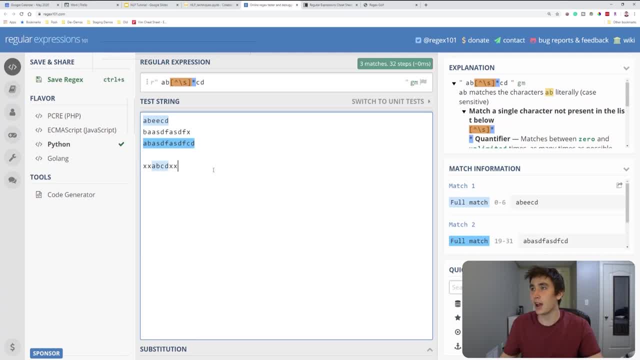 X, X, A, B, C, D, X, X. uh, and that's still saying it's a match, or at least, like it's saying the line is a match cause, that's included. Um, if we wanted to make sure that it's exclusively. 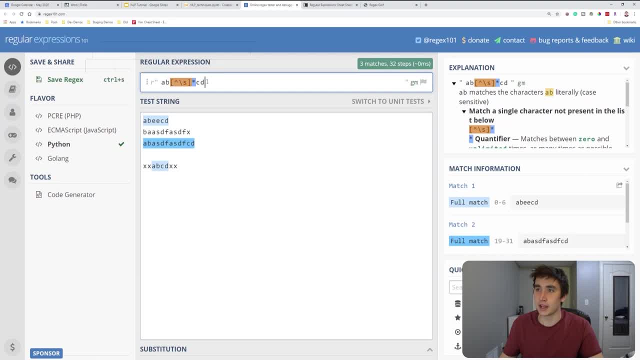 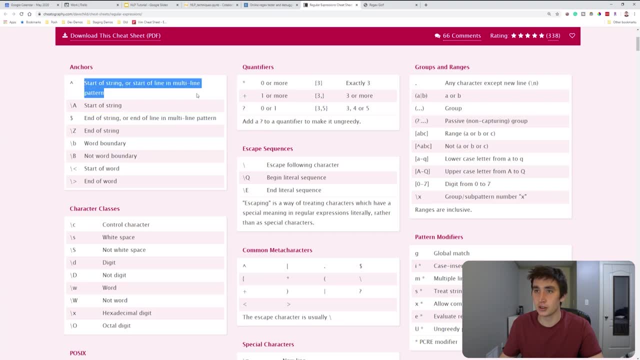 uh, this to start the line and this to end the line. we can use a couple of more special characters. So this is the end of a string And this is the start of a string. Um, this is used without the brackets and it means start of string. 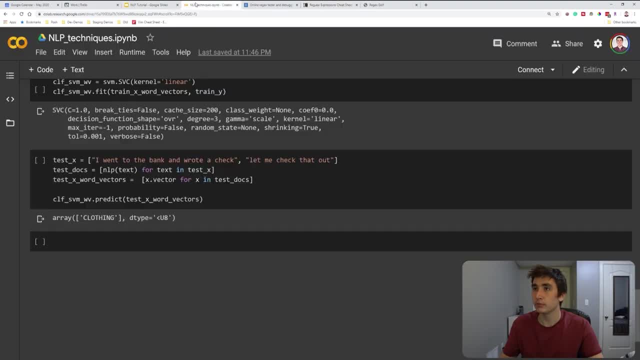 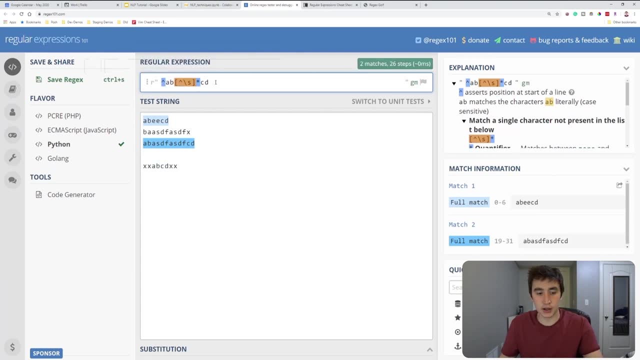 but if it's used in here it means not Um, so we can add that: So start of string followed by end of string. So now this one doesn't match at all, And that's the solution to that little exercise. So what does this look like in code? 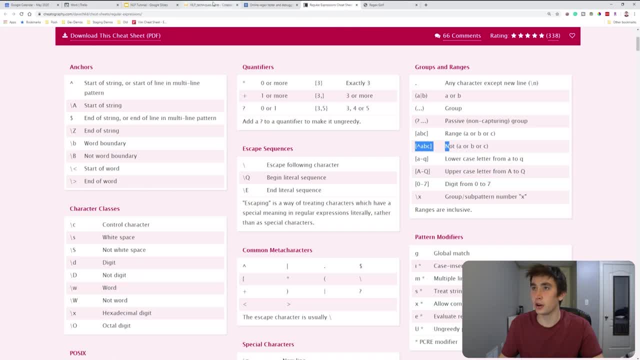 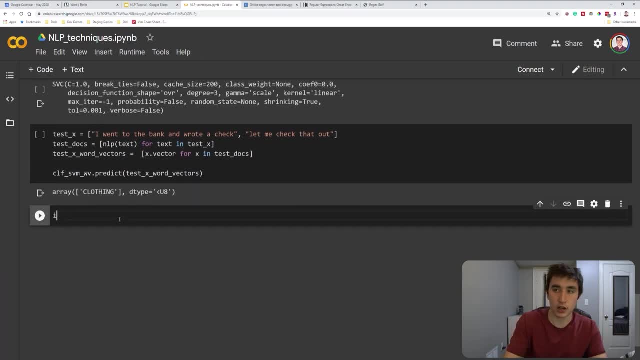 Well, we can quickly go ahead and do that. Um, if we go to our Google collab file, we can import the regular expression library, which is just um re in Python, And we can start out with our regular expression. 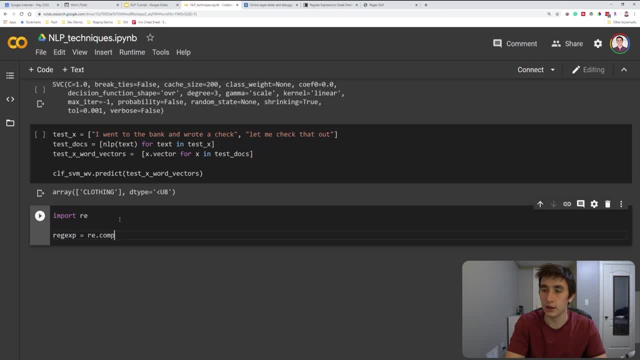 which we can define to be whatever we want. So if we were defining the one I just described, it would be carrot AB, followed by- um, not white space star, and then followed by CD, followed by the end of the line. 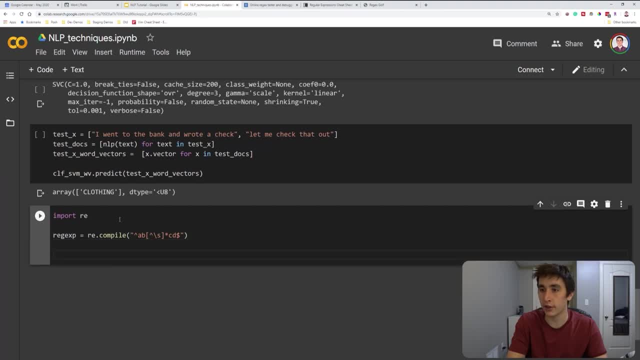 So now we compile that to allow Python to know that that's a actual regular expression, And oftentimes when we're defining regular expressions in Python, we use a R? uh in front of it just to help us highlight and help us know. 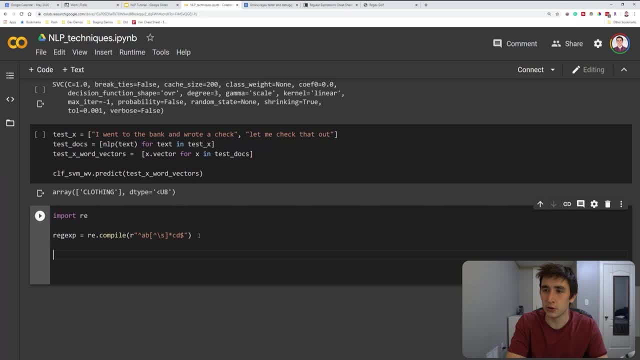 Um, and then we want to do, if we want to see if something has that we could say like test, or our phrases: ABCD, X, X X, AB, X X X CD, AB, space, CD. 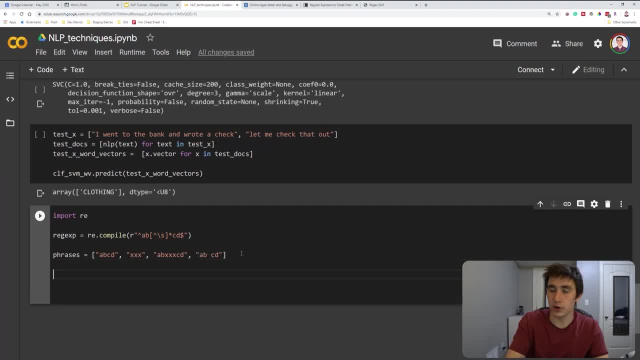 So only the first and third should match. So if we wanted to check if something matches, we can do um for phrase in phrases. there's going to be two main functions that we're going to use when we're checking for matches. 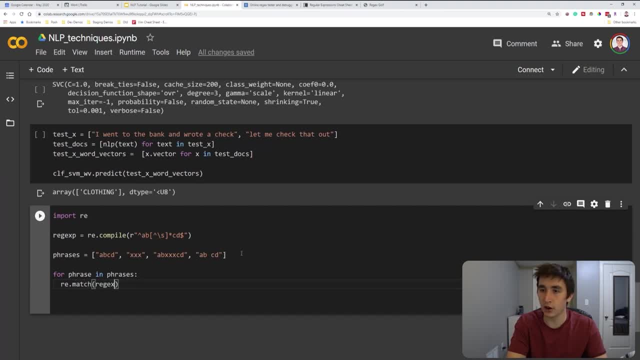 We're going to do a regular expression- dot match. We're going to pass in first our regular expression and then we're going to pass in the phrase that we want to see if it matches. And if it does match, I'm going to make this a conditional thing. 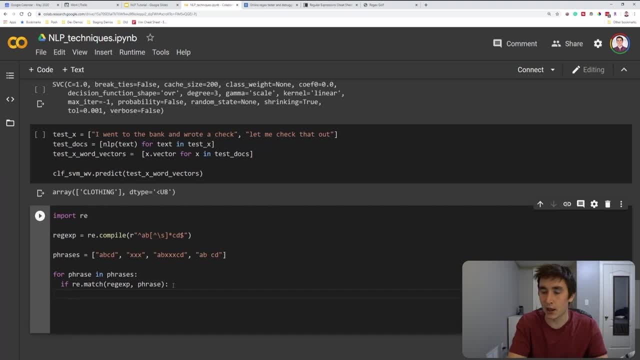 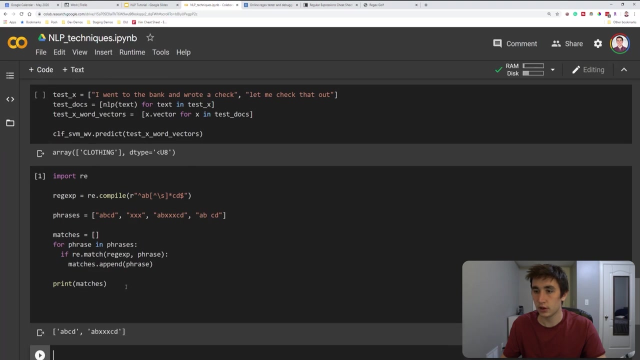 So if the regular expression matches, then I'm going to have it append to a list called matches the phrase. So we'll have to find the matches list, Okay, And then finally print matches Run, Okay. So, as you see, as we expected, 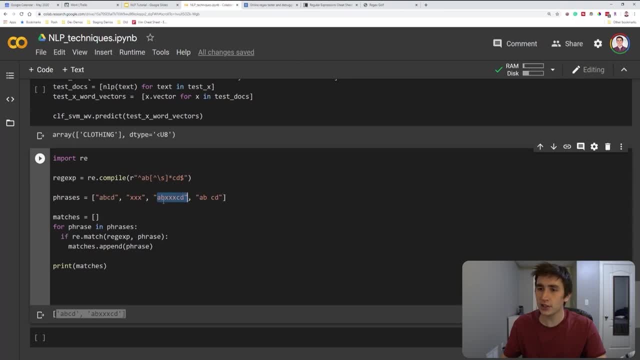 the first and third match. Um, now here's something interesting. Let's say, we took away the requirement of this having to be the first and last thing in the line, Uh, and now we added something like AAA in front and then CCC. 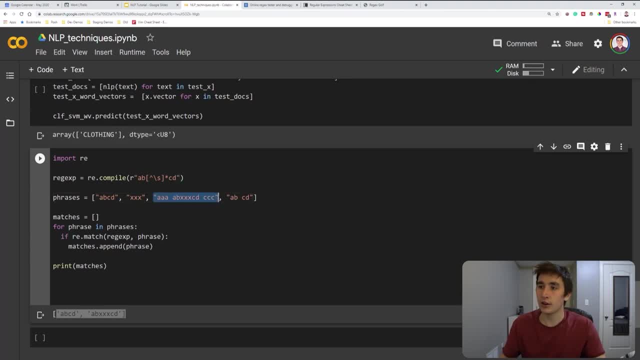 If we wanted to just check if a regex is in an entire string. So here we do have it in the string, but it's not the start, It's not the entire thing. There's places in this that don't match Uh. 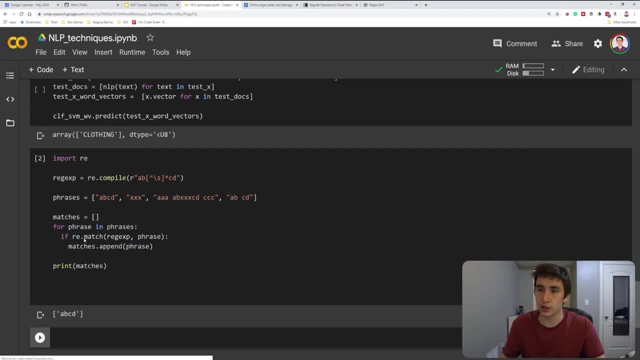 if we rerun this code, you'll see that this regular expression dot match function no longer. uh says true on this one right here. So the other main thing we're probably gonna want to use when we're searching text for regular expressions is re dot search. 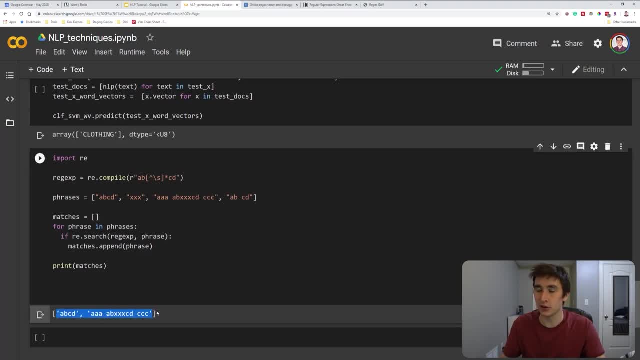 And, as you can see now, it it still matches those, those two. and quickly, just to kind of apply this to our toy example that we've been doing, Imagine we wanted to create a regular expression that matches read story and book. Maybe we're making some sort of hard coded rule to. 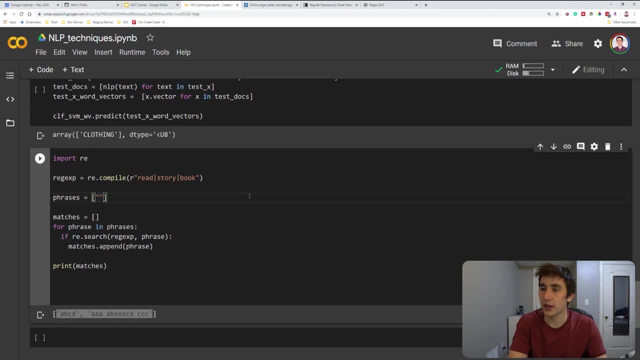 uh, we were making some sort of hard coded rule to find if something's in the books category. So I liked that story. Um, I like that book. Um, this hat is nice. As you can see, this regular expression, this is the or sign. 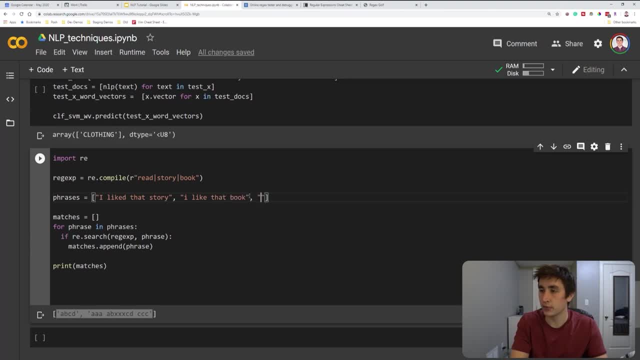 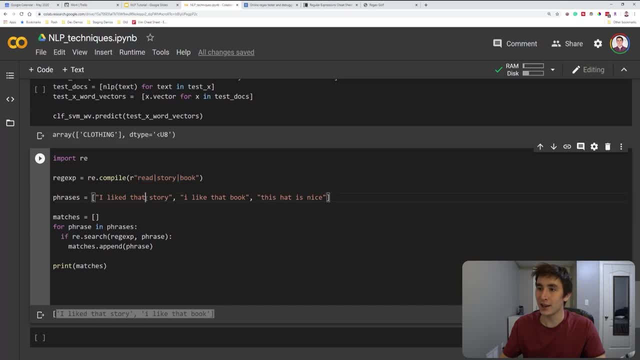 One quick new one. So if we wanted to make our, our reg X, more complicated, is that I can try to trick this and say, like history, like, instead of read, I can maybe say I, the car, treaded up the Hill. 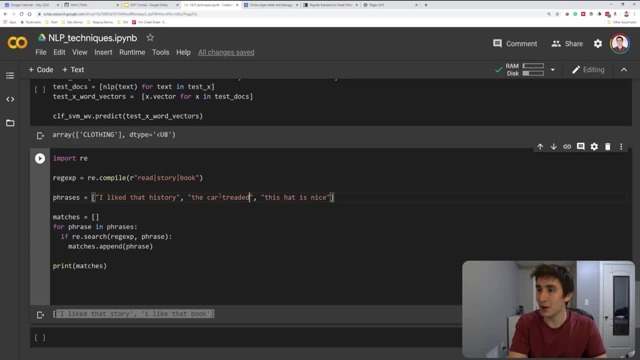 I don't know if that makes sense, but you can see that read is inside of that, but it it is not actually referencing the word read a, We'll notice that still matching the word read, matching those things. so one thing that's useful to know about is this word. 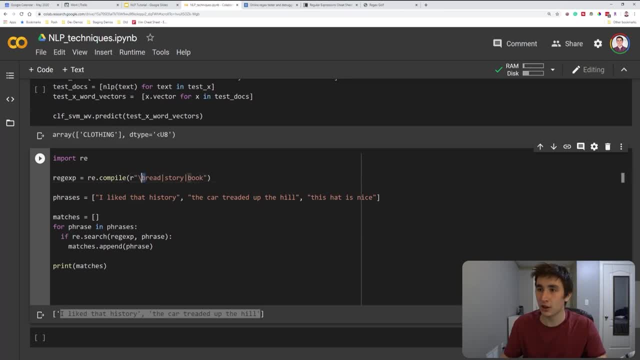 boundaries character within the regex. so forward slash B means it needs to be between word boundaries. and now watch what happens when I run this again: no matches. so it now knows that story has to be by itself. and one thing that's nice too with that a slash B format is that you can have a period or something. 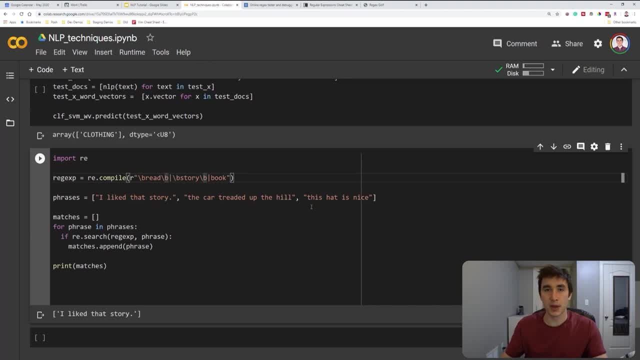 at the end. it knows that that's a word boundary, so that's like one way we maybe would apply it to our example that we've been working on. but there's so many use cases for regexes, all right. next we're going to quickly look at stemming and 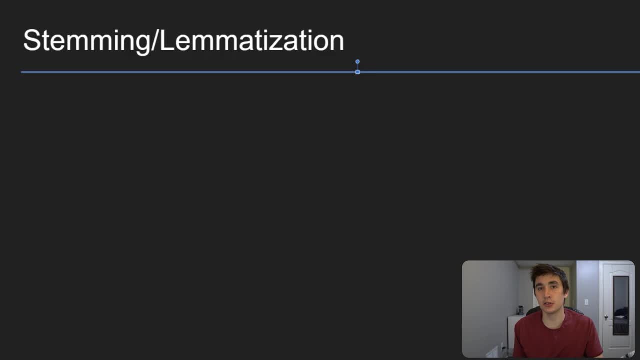 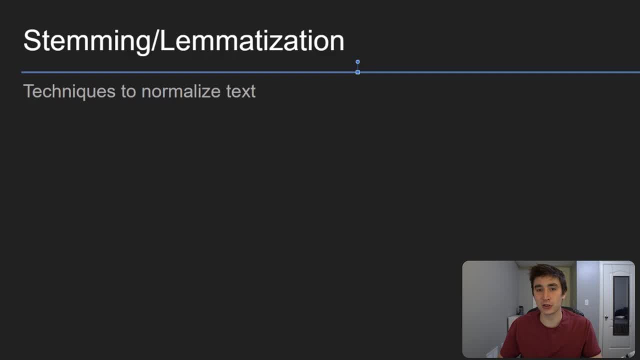 saw an example or a problem where when we train the model with the word book it didn't know the words books, even though to us that's very straightforward. so one example of what stemming and lemmatization will can do is take books and kind of reduce it down to a more canonical form of book, and it can do. 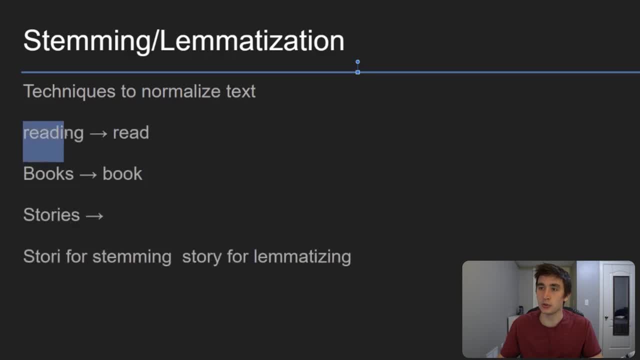 like several different things. so imagine these techniques could help you turn reading, to read books, to book stories. and now here's where, a little bit, there's a little bit of a difference. stemming follows an algorithm and is not guaranteed to give you a actual, physical, true English word, so it might reduce it down to story, whereas for lemmatizing, 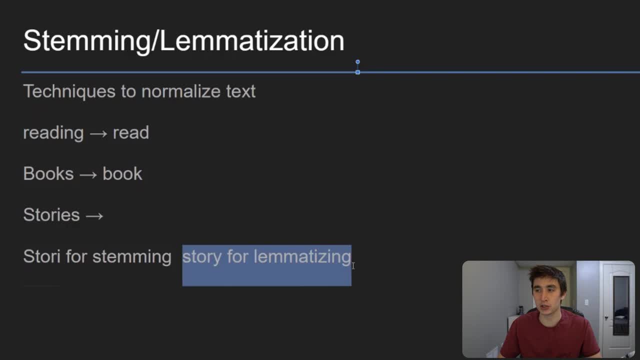 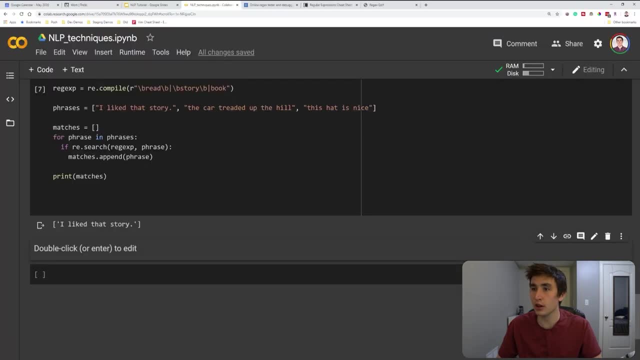 you would take stories, and it actually is using a dictionary, making sure that everything it outputs is an actual word. so that would output story there. so how do we use this in Python? well, I think the library that's easiest to you. ah, what did I say? 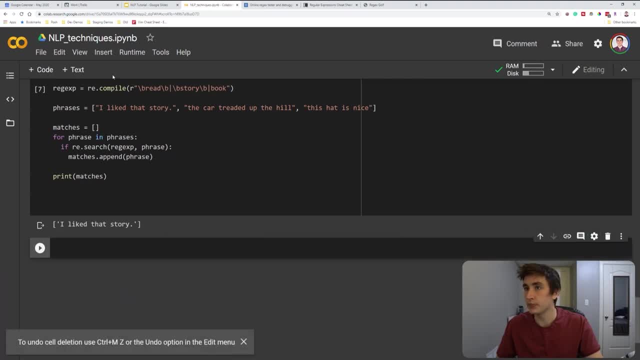 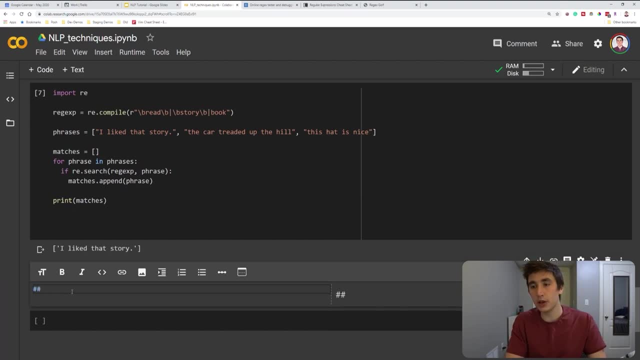 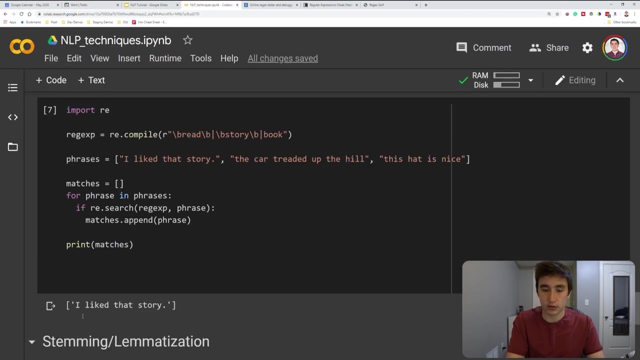 the library that's easiest to access stemming and lemmatization is probably the NLTK library, so we'll use the NLTK library, okay, so first off, we're gonna need to import NLTK, and that NLTK stands for natural language toolkit and series of secondary pages, and we can put it here as a 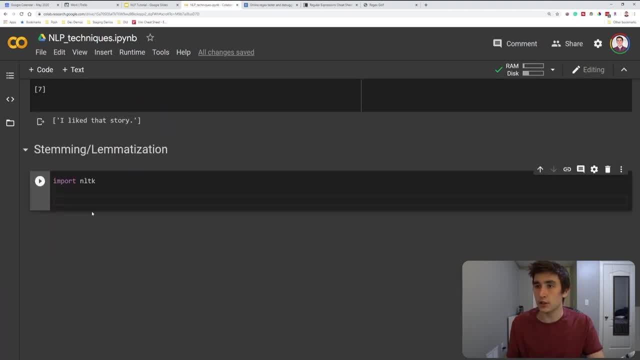 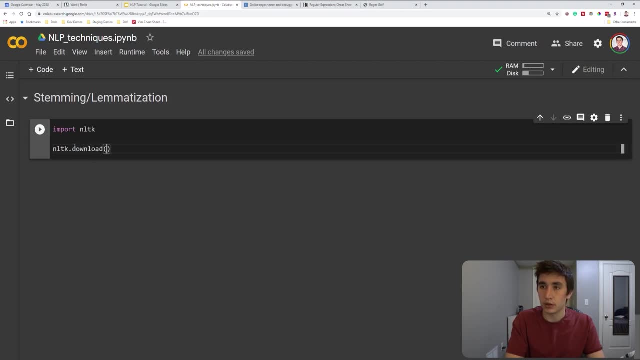 vanishing library here. gotta avoid putting those, like others, desiccating your Dom. the rest of the pages does. there's a bunch of them. they could be submitted, but I'm just gonna go there so that we can sort them out here, so that I don't have to actually insert me here, because that just doesn't contact driving. we're just gonna go there and make that link per record. we are just going to enable it. but if you're not going to underline this type of document, go to how sphsrm post to have a a train of things on it. sorry about that. job. we hit enter right. where is it zoom? got a email that's going to come down. I think fit is the app on the right page. I'm trying to do too much import NLTK and we're also going to need to do is import a couple or download a couple of things for an, etc. and this syntactic. 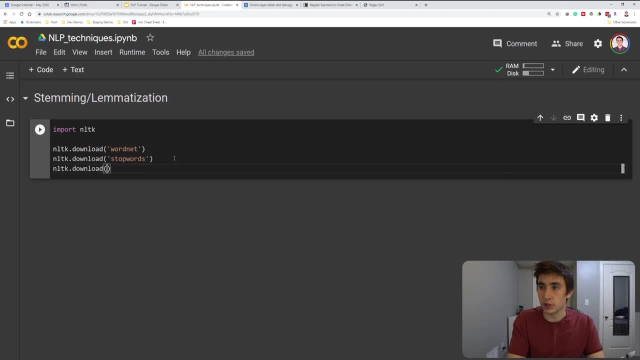 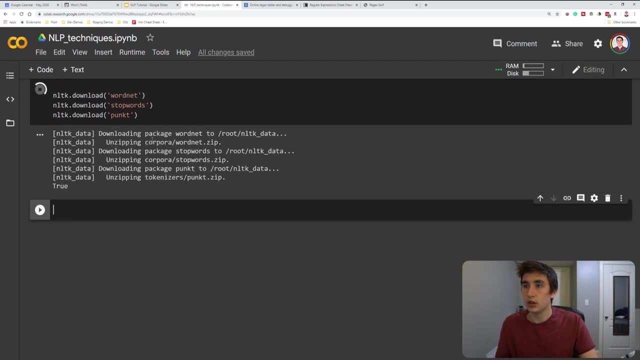 I think the stop words is going to be for my next example. I don't know if we'll need that for the stemming and lemmatization section. All right, downloading all that, And now let's go ahead and start with a stemmer. 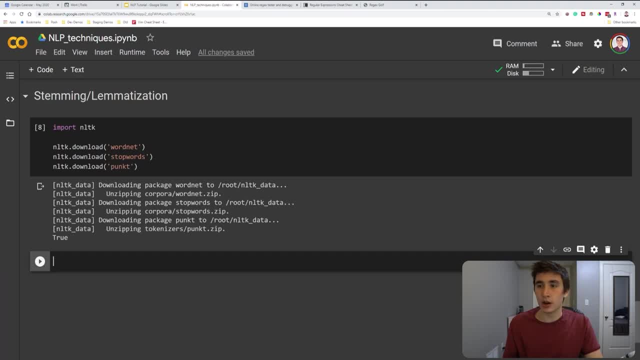 So to get a stemmer, I recommend importing two different things. I recommend importing the tokenize library, which basically can take a sentence and break it into its individual words. So, as well as the actual stemmer- And we're going to use the porter stemmer for this example- 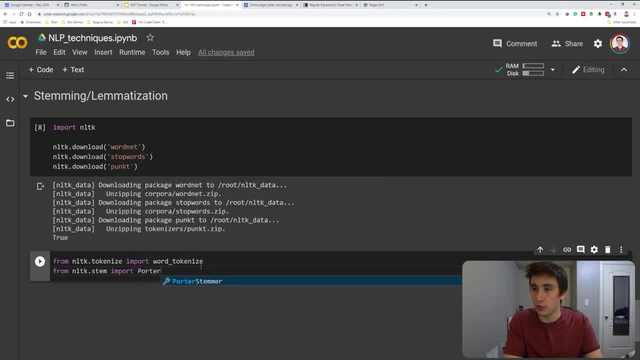 So I'm going to do nltkstem and we'll import the porter stemmer. And now let's go ahead and initialize that stemmer. And now we can just type in like a test phrase: Okay, so reading The books will say: and to first we'll need to tokenize that. 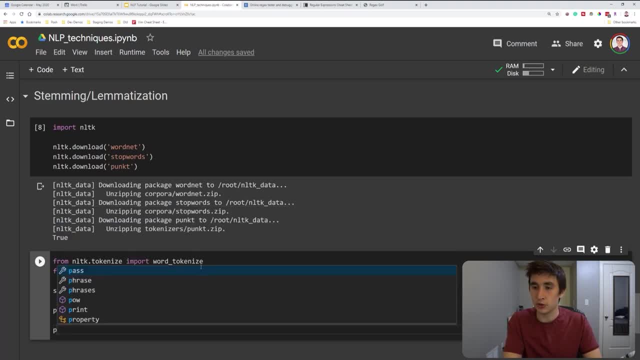 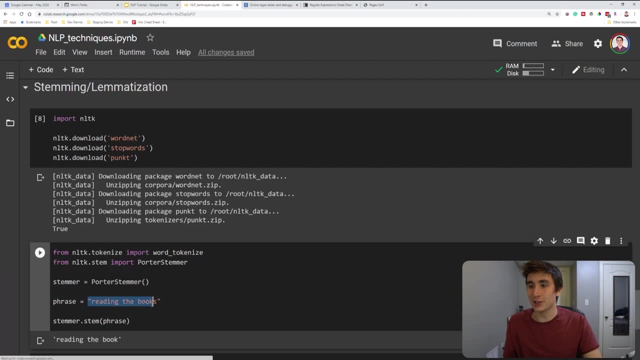 because if we just try to stem- but just try to- I do stemmerstem. This is all you have to do to stem of the phrase. It doesn't know how to process this because this algorithm expects a single word, So we're going to have to tokenize it. 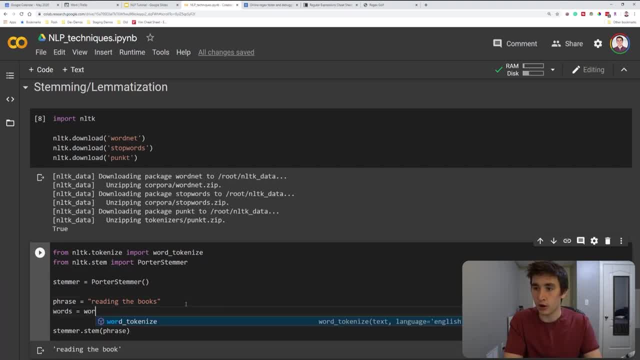 So we can just say: words equal word, tokenize of our phrase. And now we can just do stemmed words. We're going to do this in a for loop, So that for word in words, we're going to stem the word, Stemmerstem of the word. 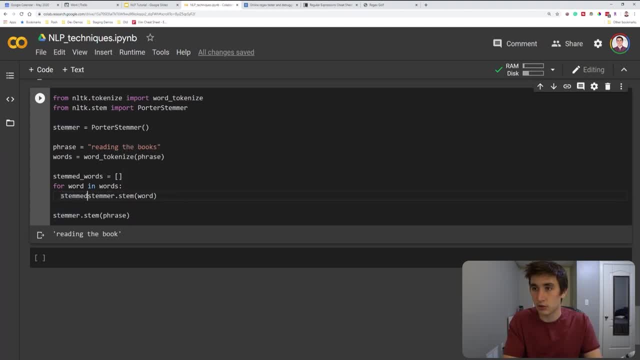 And we're going to append that to our stemmed words. Okay, Okay, and now we can do a join by spaces of the stemmed words as the final thing. so we started with reading the books and the stemmer. now it got us down to reading the book and this immediately can be seen to be very helpful for like. 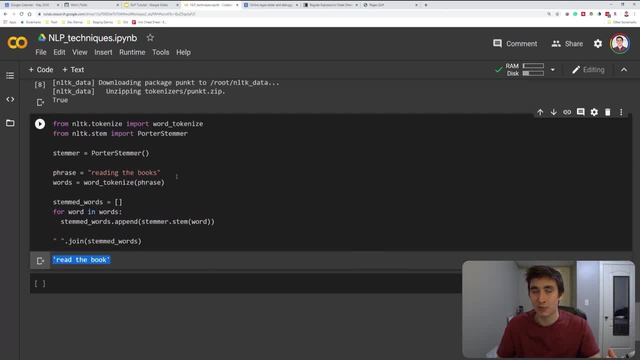 that bag of words model that we built earlier, where if you didn't have many training examples, if you did stem the training examples you did have and stemmed any incoming phrase that you didn't hadn't been trained on. it would probably help improve accuracy there. a couple examples to see. so if I did, I 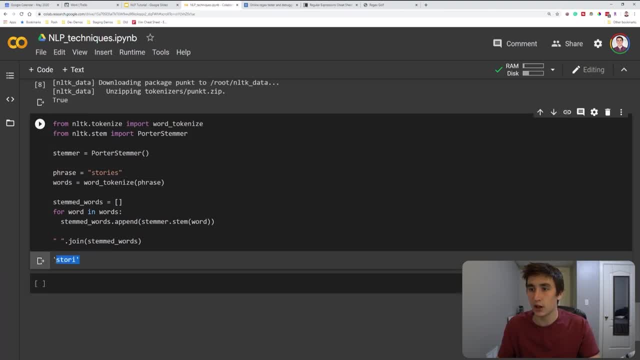 said stories was one that was a little bit weird. see how it stems it to story. so it's not guaranteed to have a word, and sometimes you'll get collisions on two words that aren't necessarily similar. so there are some drawbacks, but it's a nice little quick trick to have, I think. I just want to check something. 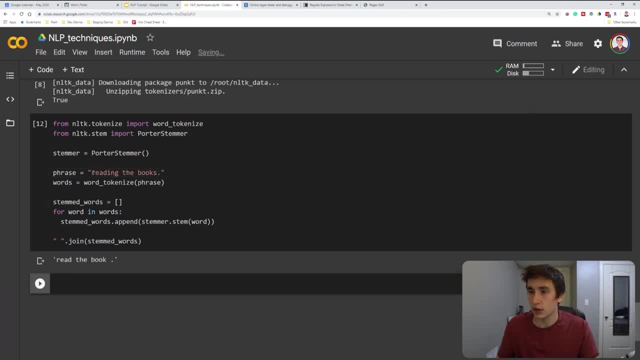 with that whole tokenization. one thing to note is that you also might want to like strip out your punctuation or handle that a little bit separately if you're trying to return a phrase that makes sense because, as you can see right there, it uh at least the 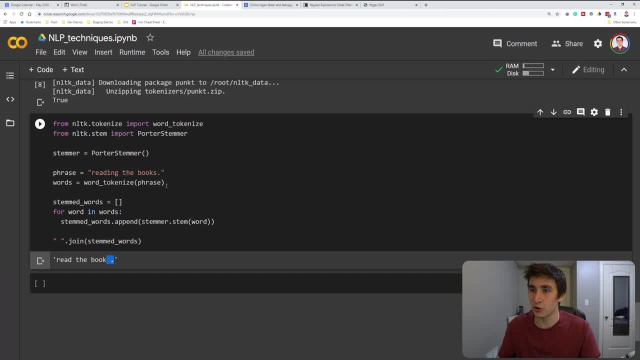 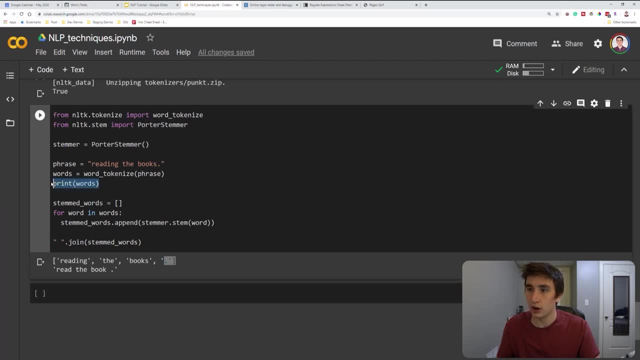 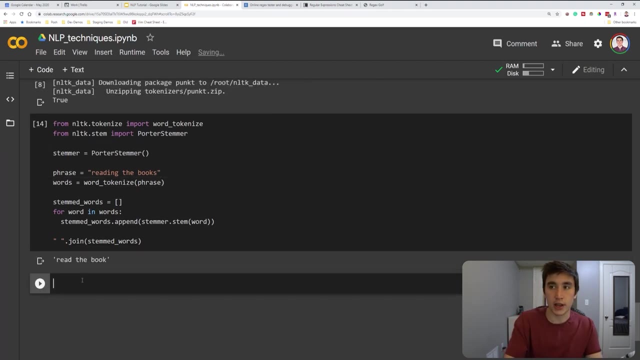 way I define this. you have to be a little bit tricky, because when you tokenize this, I print out the words. it treats the punctuation as its own own word. all right, moving on to lemmatization. let's now from NLTK dot stem import the word net lemmatizer. so this is using this. 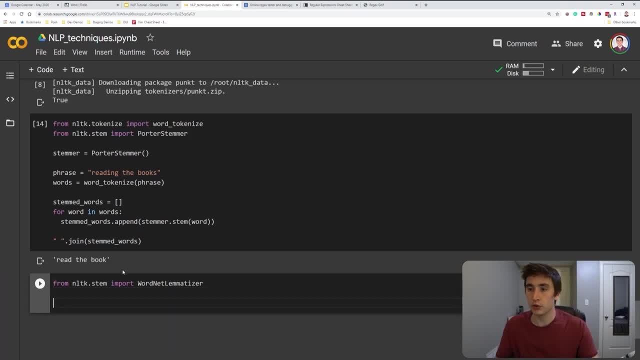 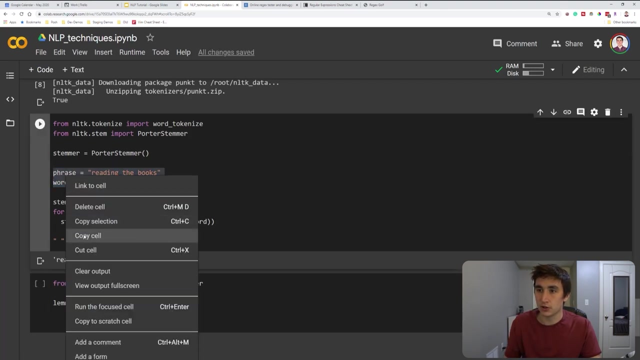 corpus called word net, to help reduce these words to a more simple form. all right, so pretty similar to the last one we could just do: lemmatizer equals word net, lemmatizer and same thing for the example as before. we need to tokenize whatever phrase we use. oh my god, I didn't mean to. 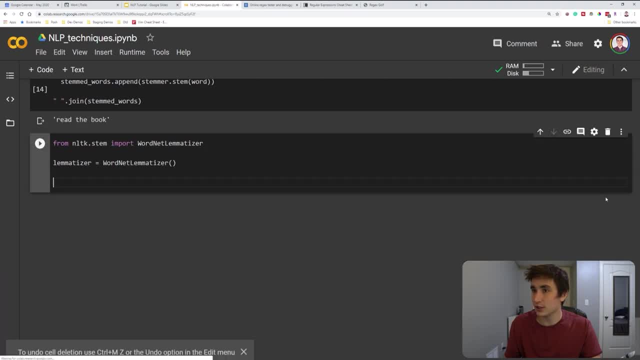 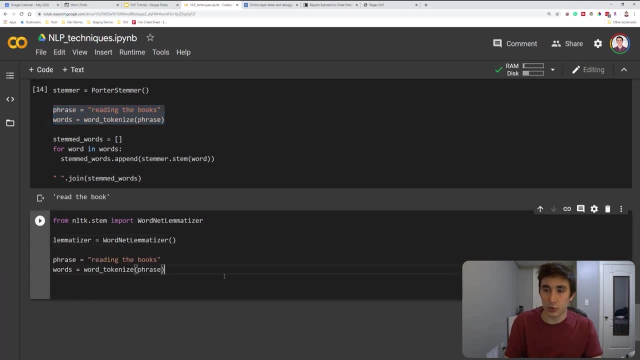 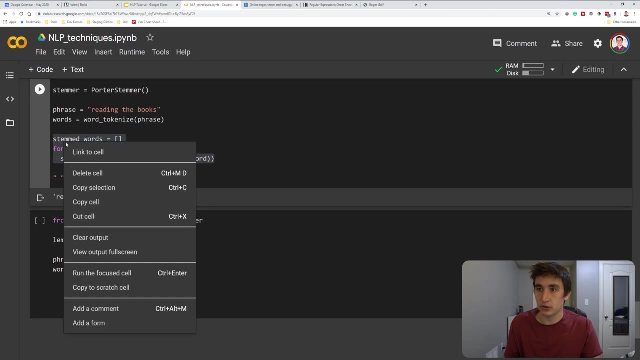 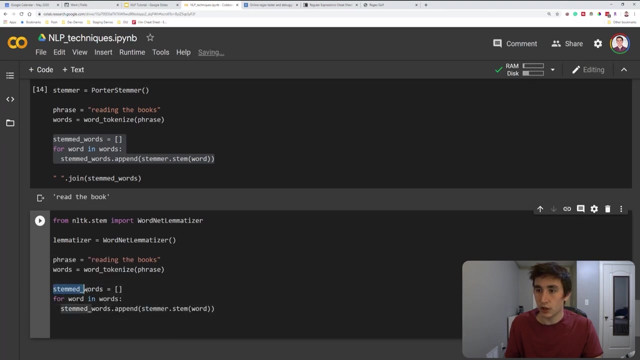 copy the cell. no, delete this. I just wanted to copy this part. all right, so, reading the books, let's see what happens if we. I'll copy this to: no, not the cell, just the piece, the sheathe punishing, and this will be lemmatized tithed words. 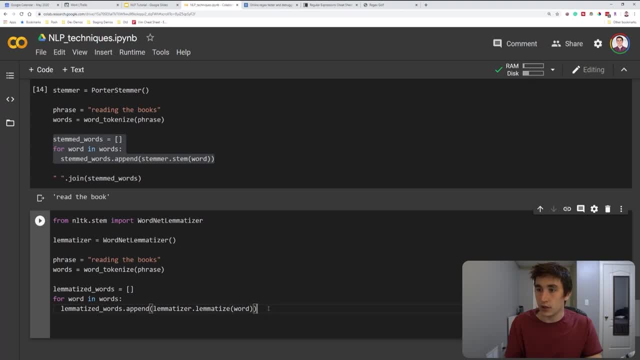 dot, and it's pretty straightforward: instead of stem, it's lemmatize. it's two M's the word, and let's see what happened here. oh, this will be lemmatized. it does a待 print lemmatized, or i guess we'll do. we'll join them again: dot. join of lemmatized words. 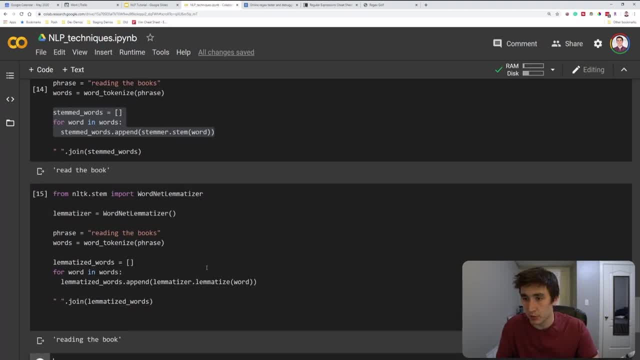 all right, run that. what's gonna happen? reading the book, okay, hmm, it's a little bit different than our above example that turned it into read the book. and here's one uh thing that's a little bit trickier about using the lemmatizer with nltk: is it expects for each of these words, it expects. 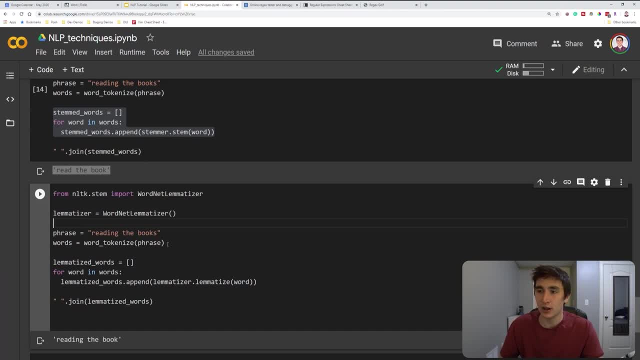 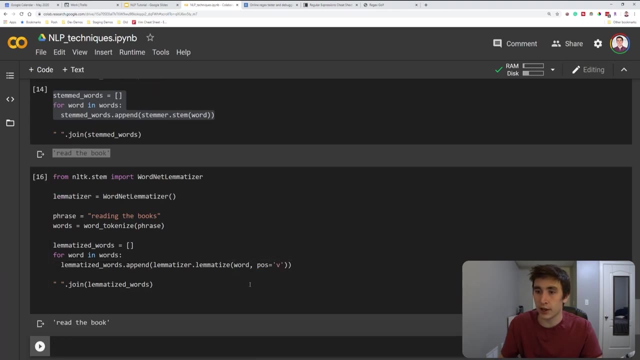 the part of speech and by default it um says that each token is a noun by default. so that's why it converted books to a book, but not reading to read. if i instead said these were all um verbs, we'll see that it is read the book. i guess that's interesting. uh, still made books book. 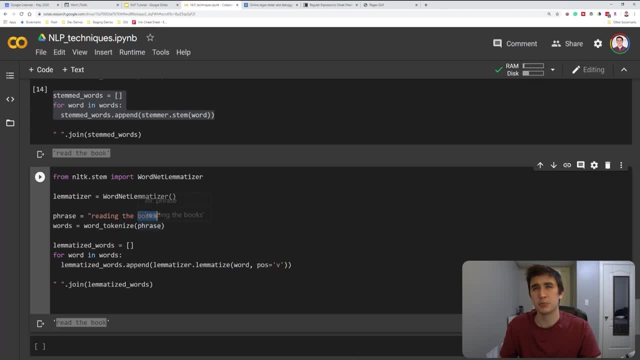 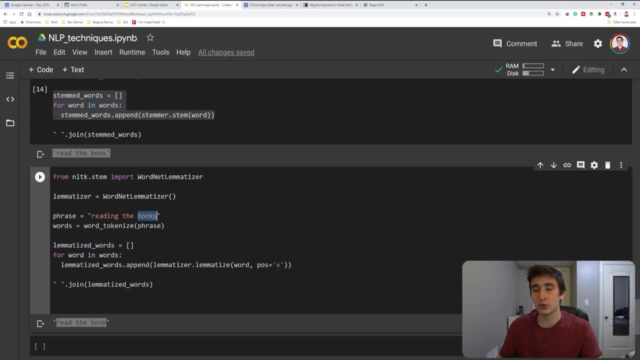 is a verb: books. but yeah, the one caveat is you, if you're trying to effectively utilize this, sometimes you have to do some sort of part of speech tagging- which i believe i'll get to in the tutorial- and then maybe utilize that part of speech tag here to like. 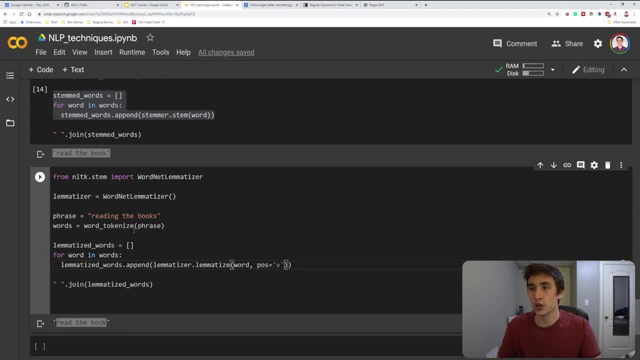 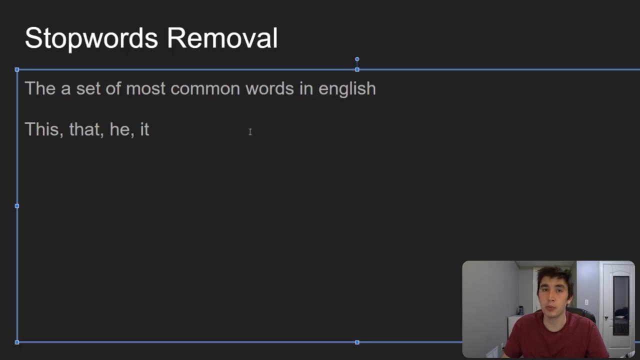 truly reduce down all the words, but it might be also helpful to just reduce down all your, your noun phrases or all your verbs. um, so that is lemmatizing and we'll, we'll, move on from there. next, while we're still looking at nltk, we're going to quickly go over, stop words and basically stop. 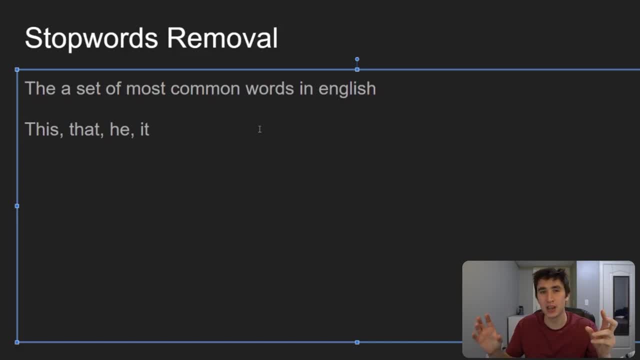 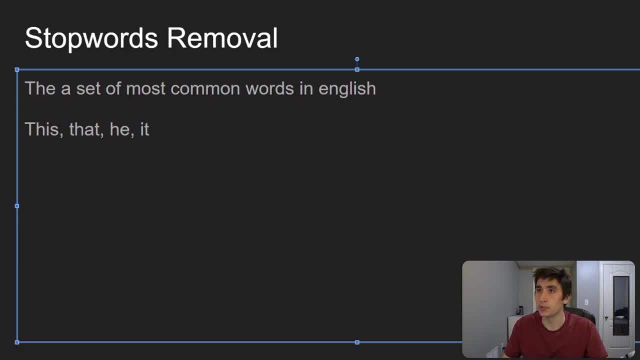 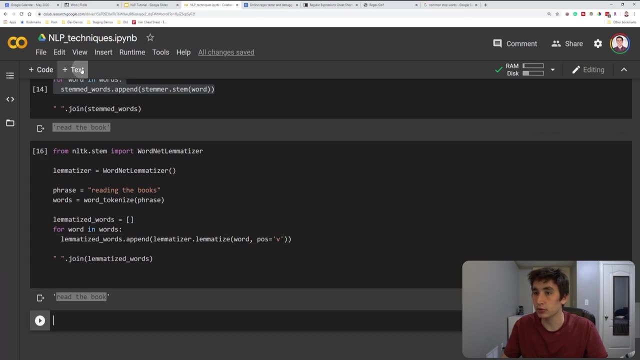 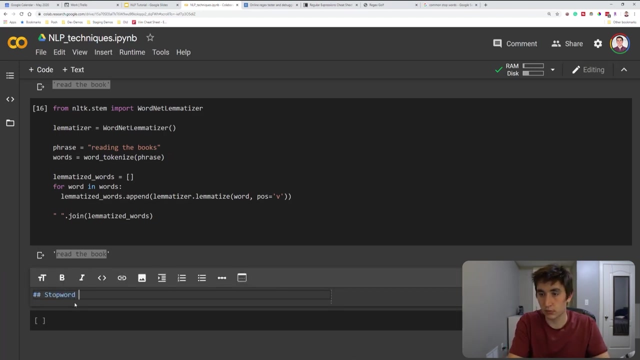 it. uh, the these, them, those types of things. so we can easily do this in nltk. so here we go. okay, so we're going to continue using nltk. we've already imported it at this point and we're going to do um, actually, maybe just for help they'll. be helpful is if i 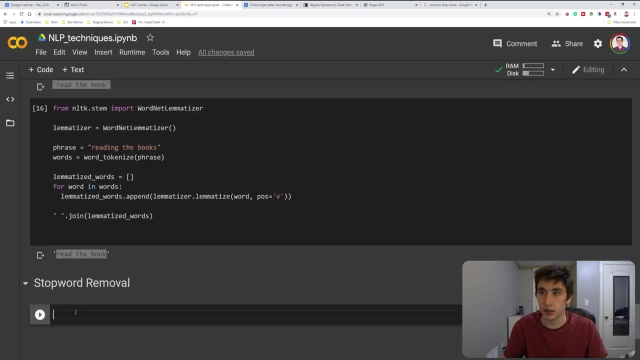 copy in this, just in case people run these independently: uh, paste in that, and then we're also going to have to copy in, uh, the actual stop words. so we're going to import stop words and here we go. so our stop words are going to be: um. 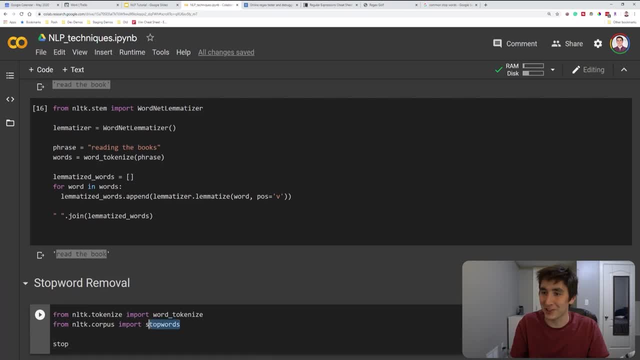 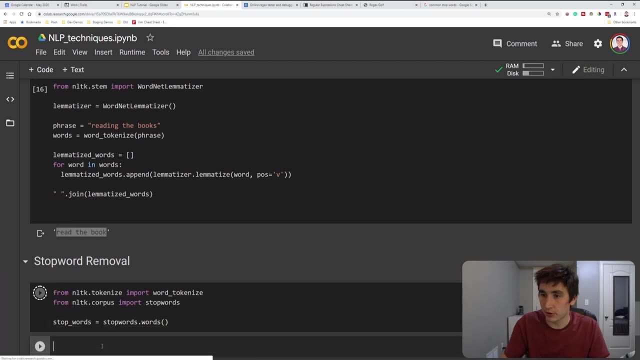 i don't want to do stop words because otherwise i'll overwrite this import of stopwords. So I'll just say stopwords equals stopwords dot words, And then we have to pass in that we want English. I believe, Actually, maybe it would work without doing English. 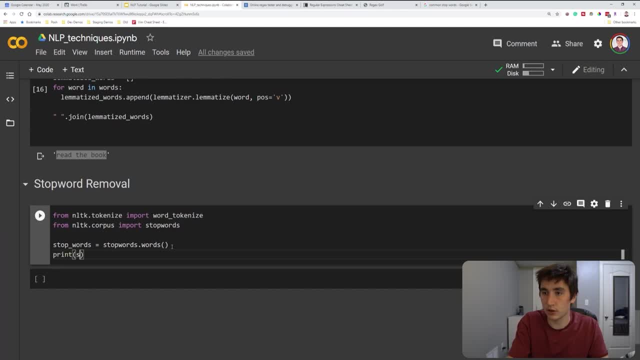 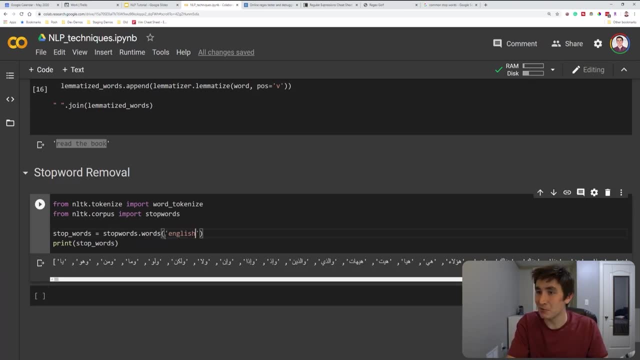 So let's print out stopwords. I think it's. oh, I guess. I guess you do have to specify English, because I don't know what that means. Cool, I me, my myself, we, And I'm curious how. 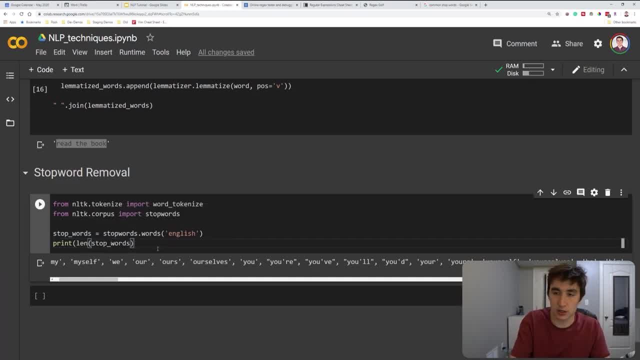 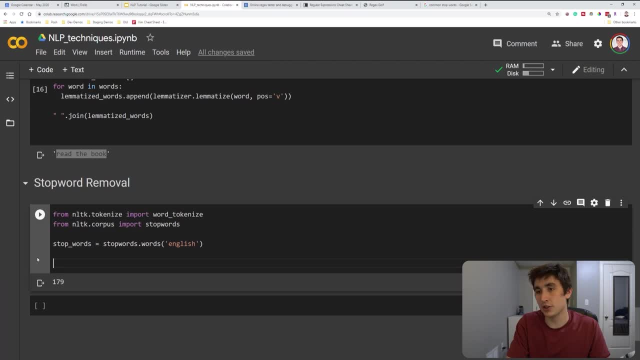 many of these are there. So length of stopwords: 179.. So there's 179 words we might want to extract out, And this just gives us a nice easy interface to do it. So what we could do is we'd have a phrase just like before. So here is an example sentence. 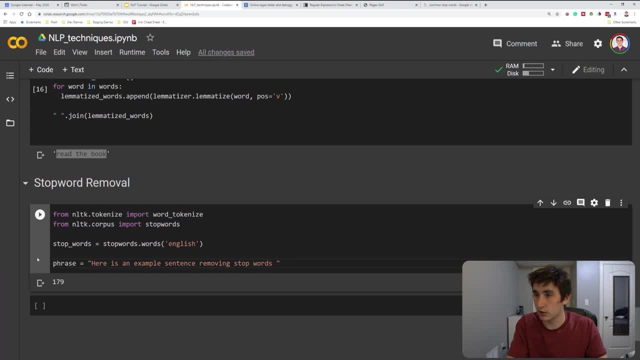 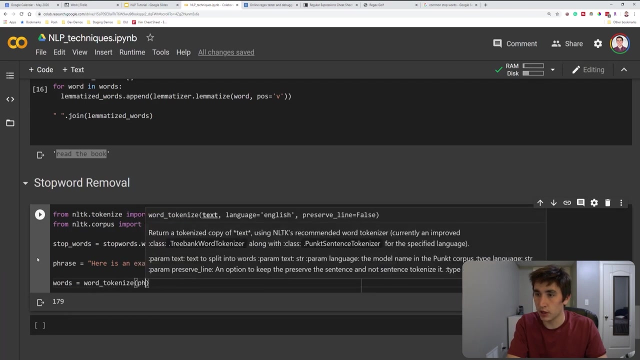 Removing stopwords, I'll just say demonstrating the removal of stopwords. So that's the phrase to begin with, And now we will tokenize that, just like that we did before. So our words will equal word: tokenize of the phrase and then forward in words. Well, 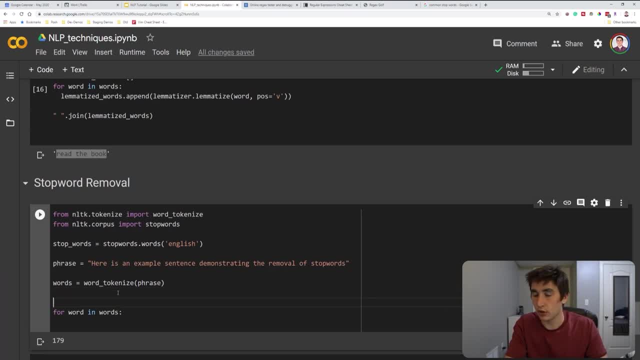 I guess our stripped phrase- I'll call it that- equals. So if word not in stopwords, then we can append it to the stripped phrase. You probably could do this in a list comprehension too. So whatever you prefer, And then we can do join of the words, Or we could just keep this as a list, because I guess 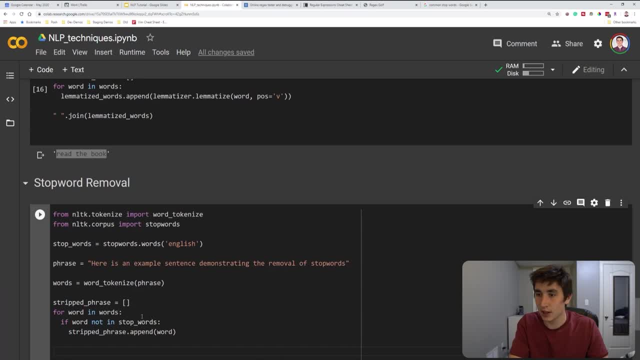 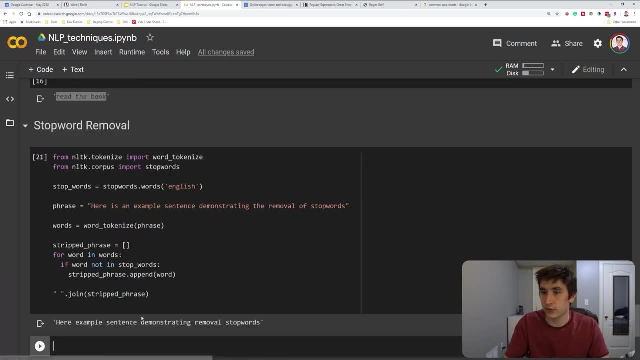 it might not fully make sense as a stripped phrase, We'll join them anyway. Join stripped phrase. Okay, Here example sentence demonstrating removal of stopwords: So is and the of were all removed as stopwords, And how this could help us is going: 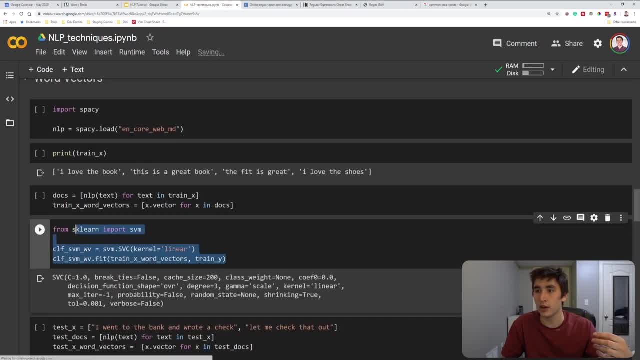 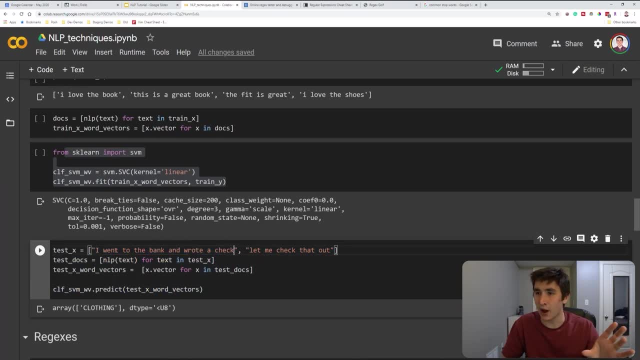 back to the word vector model from above. If we maybe said something like I went to the bank and wrote a check, you know we might get bogged down by some of these stopwords in the actual meaning of this as we average together those word vectors, So removing the 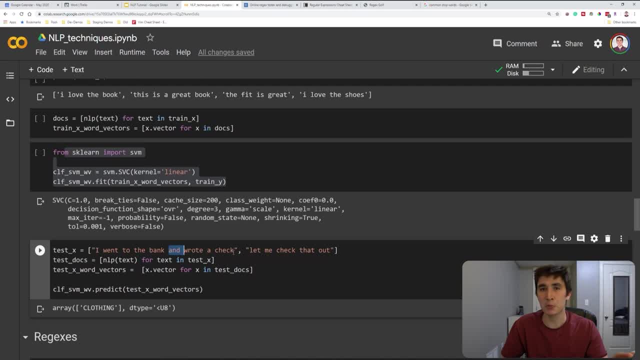 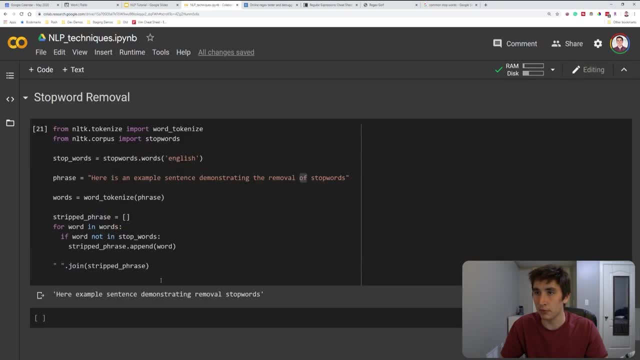 stopwords might give us a little bit more precise capturing of meaning in something like this. That's just one example. There's other examples where removing stopwords is helpful. Next we're going to do kind of a rapid fire round of the rapid fire round, And I'm going to just quickly go. 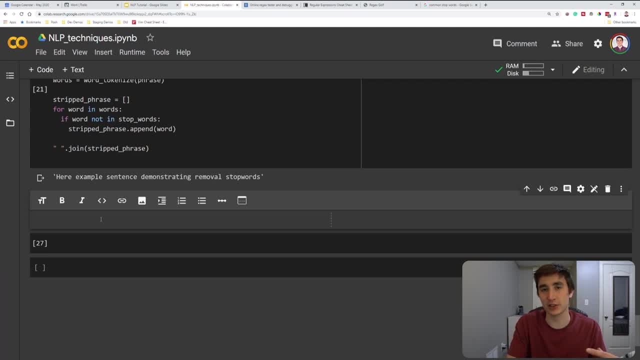 through another library called TextBlob. that allows you to access all sorts of different nice little things with language quickly And it builds off the NLTK library And it gives provides like a really nice interface for doing a lot of different things. So I'm going to just say various other. 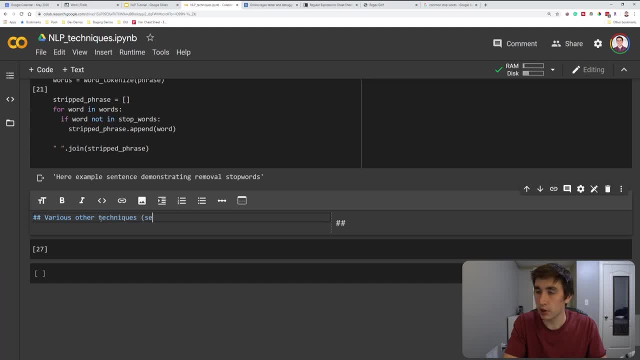 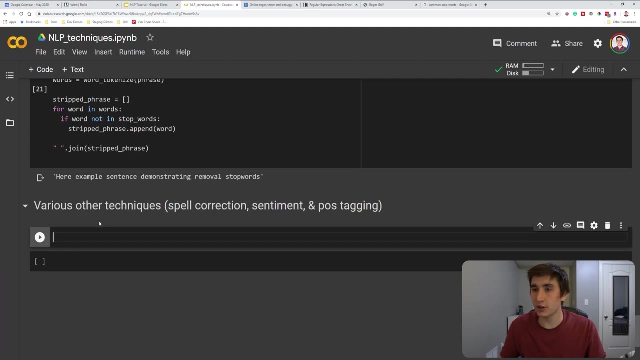 techniques And we'll look at spell correction, Sentiment And, let's say, part of speech tagging, All right. So when you're wanting to use this TextBlob library, I recommend actually just looking at the reference And I will make sure I link this. 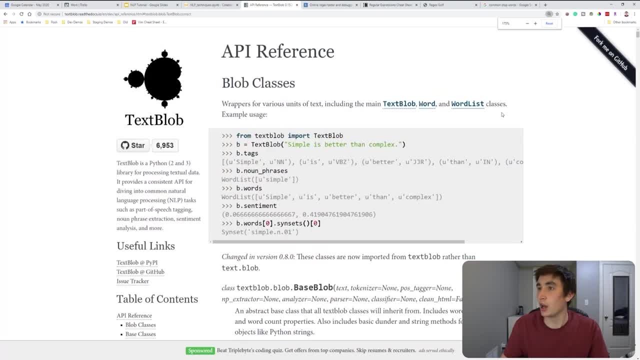 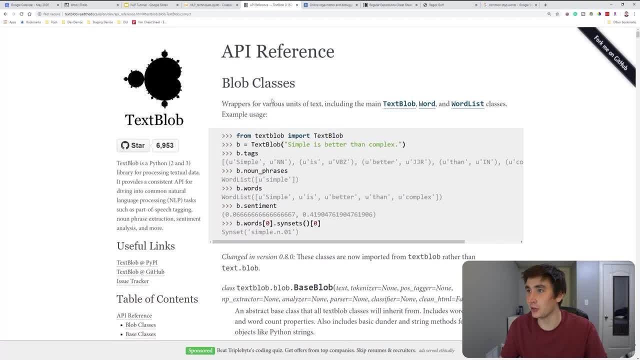 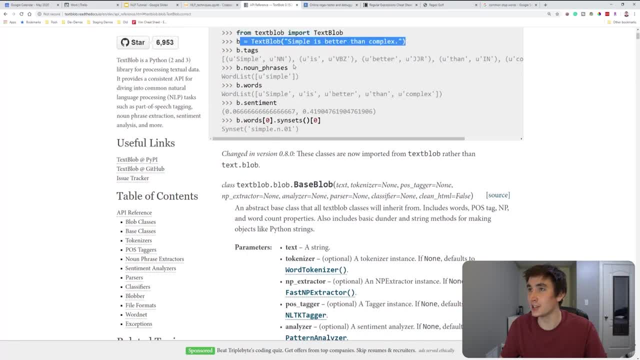 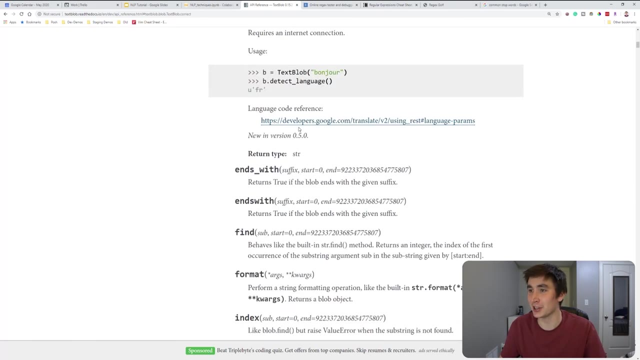 first line, As you can see, you literally just taken a phrase And right here b dot tags. we've already done part of speech. tagging you can do like dot noun phrases, dot words, dot sentiment, do all this stuff with like one line, like just a single dot something. So the first one I wanted to 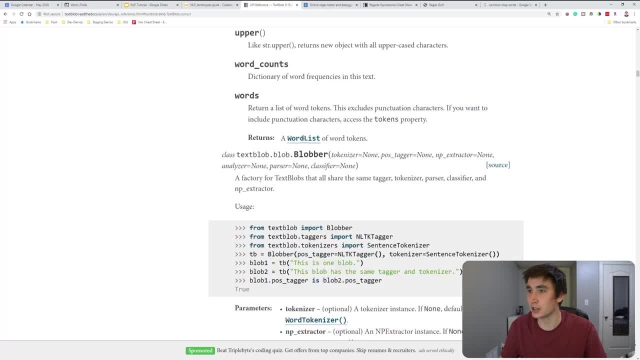 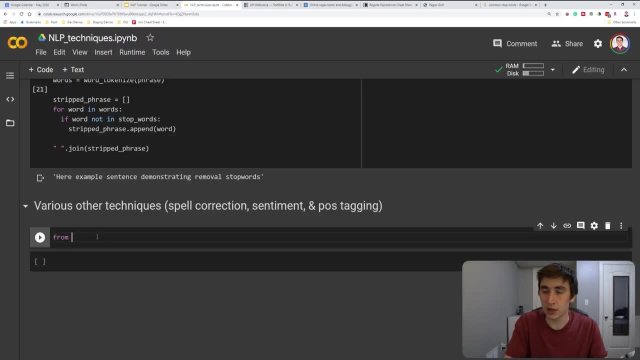 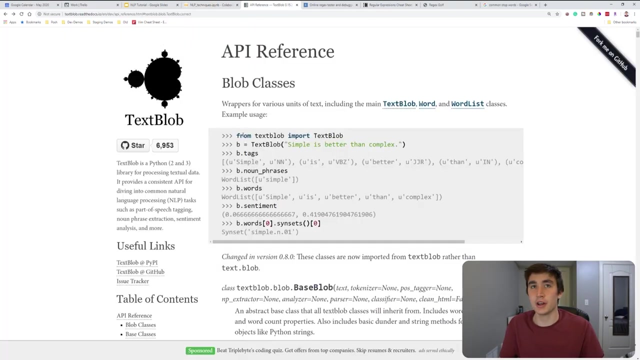 look at, was the spell correct And where is that Correct? Here we go. So let's go to the code from TextBlob. Oh, shoot, From TextBlob. import TextBlob. Cool, Okay, so whenever we do anything with TextBlob, 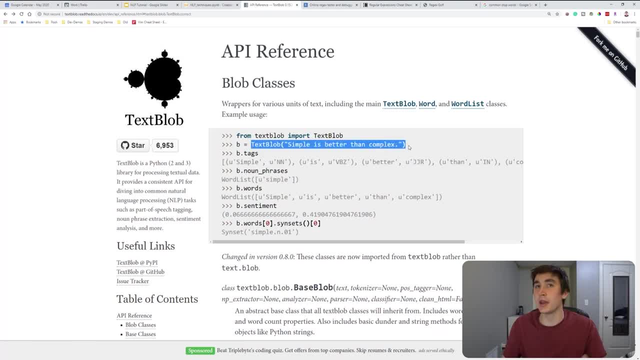 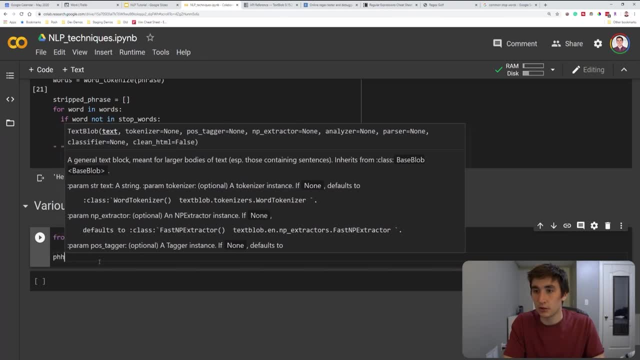 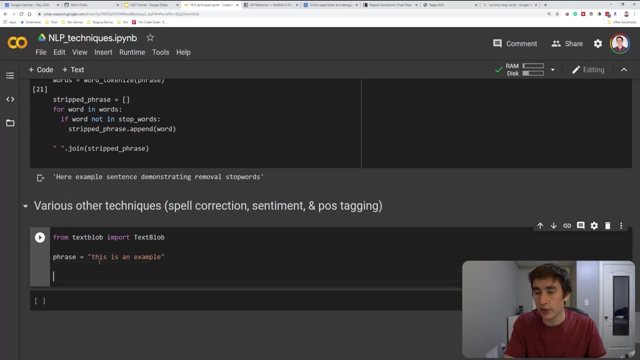 what we're going to want to start with is just basically baking our phrase a TextBlob object. So we're gonna go phrase and say: whatever it is equals- This is an example. And then what we're going to want to do is just do- we're gonna even just surround this or I'll just say TB phrase. 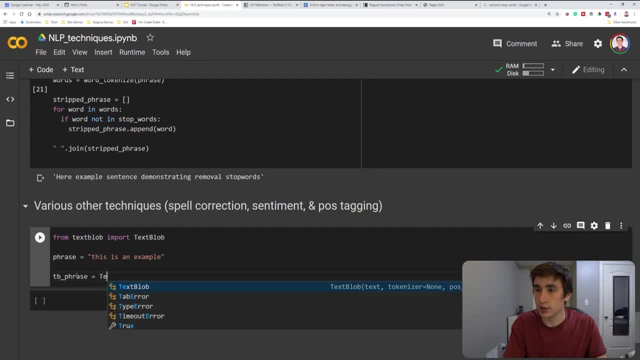 or TextBlob phrase, converting it as text blob, and then phrase: Okay, and now I'm going to do our shape. Now, with tbphrase we already can do all sorts of nice things. So the first thing I mentioned was spell correct. 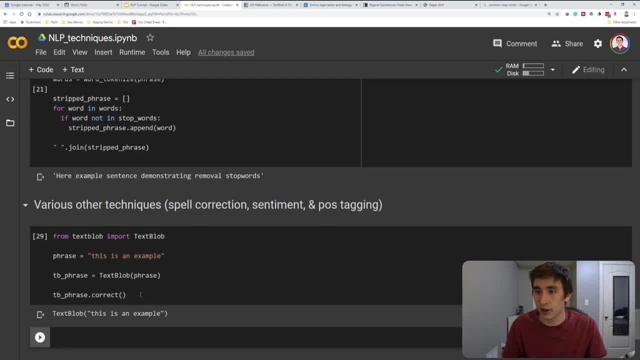 So tbphrasecorrect is all you have to do to spell correct that This is an example. What if I said this is an example and used two e's- See, it's still. this is an example. If I use like two i's here, it probably will still think. 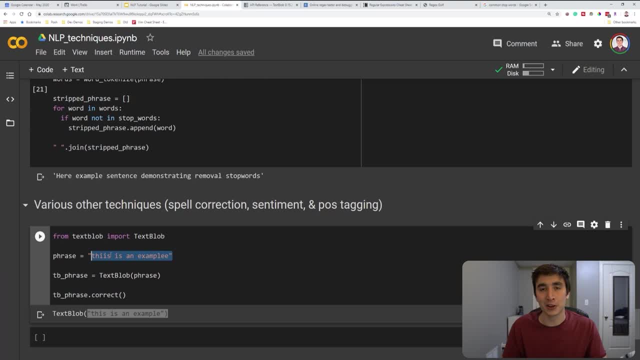 Look at that. It's correcting this very quickly. And when I mentioned that original goal of this tutorial was, you know, taking tweets and processing it, you can imagine that a lot of tweets are misspelled and have this So being able to in, you know we could easily make this two lines of code. 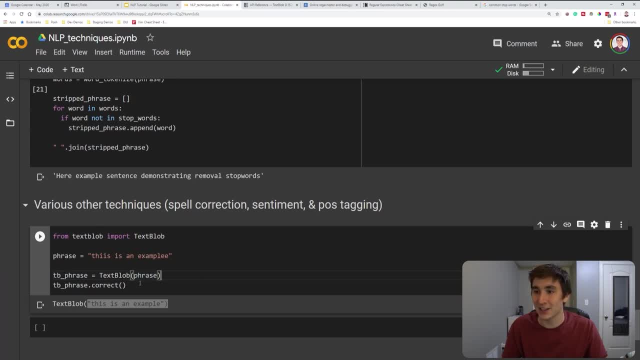 actually even a single line of code if we really wanted to get fancy Do spell correcting on a phrase. That's pretty, pretty helpful. So what else can we do with TextBlob? Well, I mentioned you could do part of speech tagging. 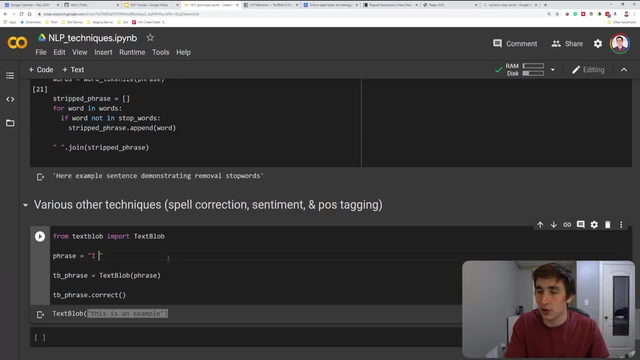 So I'm going to go back to our reading examples. So I read the book. so obviously we don't have any spelling errors there. but one thing we could do is get the parts of speech, and I just have to do dot tags to do that. 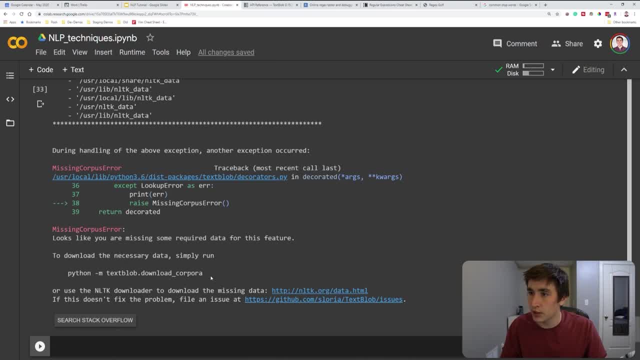 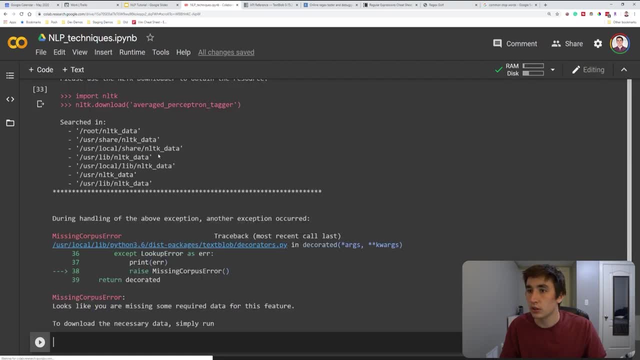 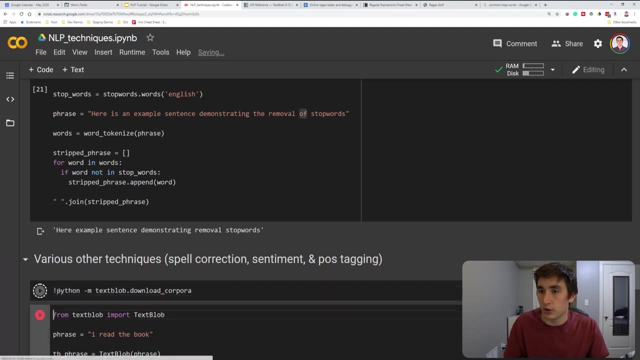 OK, what do we see? It looks like you're missing some required data for this feature. OK, so I'm going to real quick add this to my Google Cloud file and, just like I downloaded some stuff earlier, I will run this. 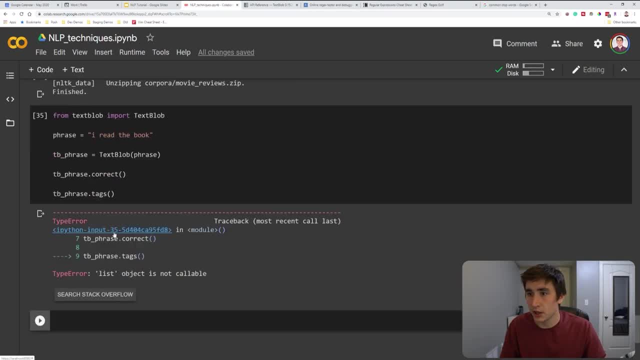 Cool, it's done, and now we should be able to do part of speech. tagging List object is not callable. It might have been just dot tags. It might already be baked in. Look at that. So we have. I, which is a noun. 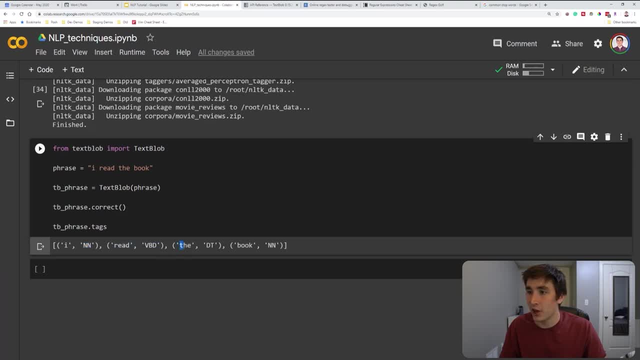 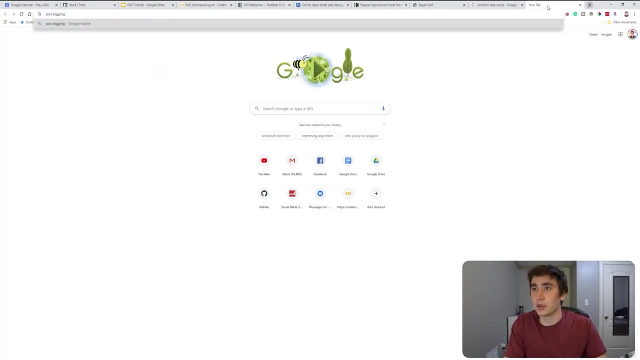 We have read, which is the verb. We have the, which is whatever DT stands for, and then a book, which is another noun And Um. If you just look up like part of speech, tagging Um, You probably will. 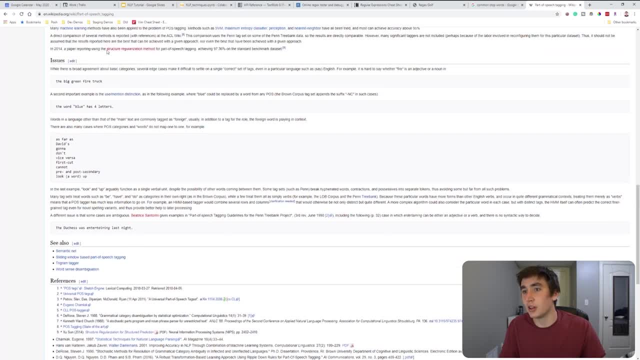 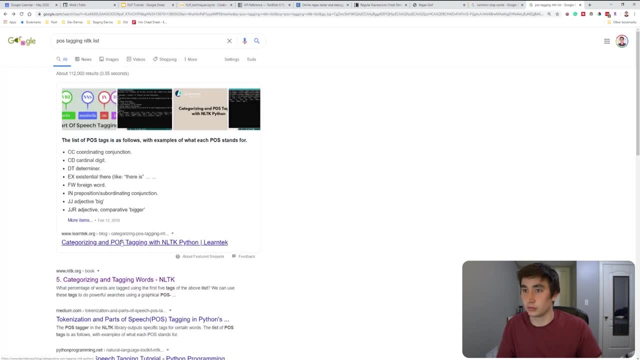 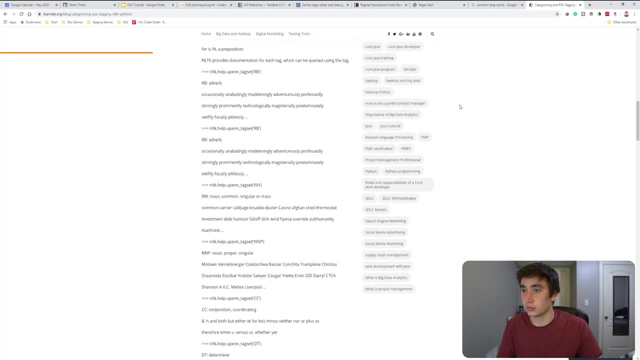 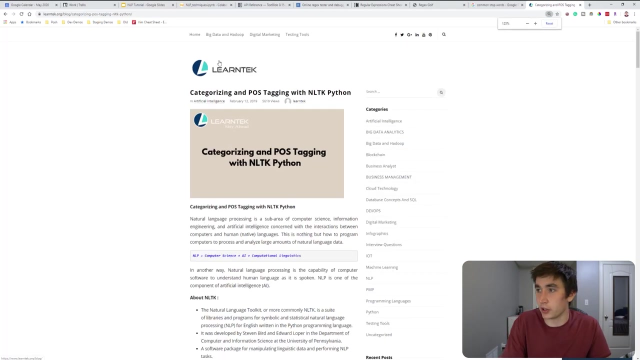 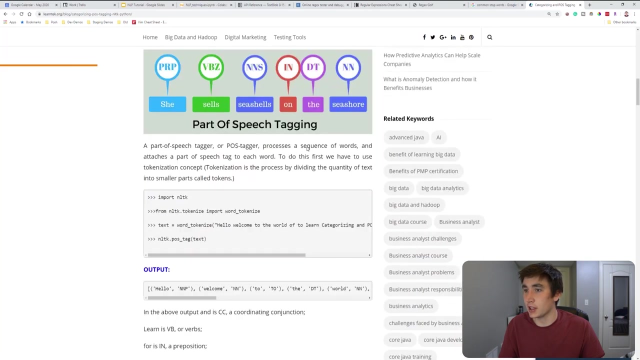 Find information on the different Variants, And so this um I'll link this in my GitHub. I found this page as a helpful resource um to learn about the different things that you see. So you, we did see, OK, like DT is the. uh, what do these things actually mean? 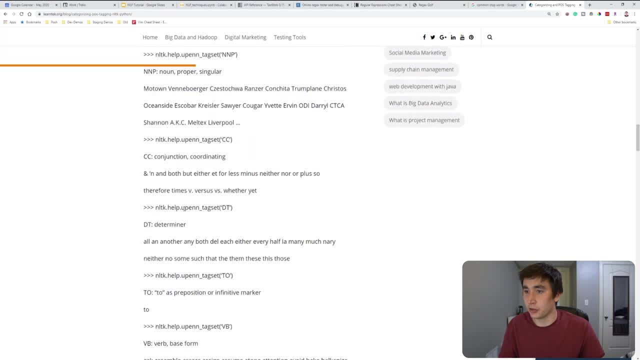 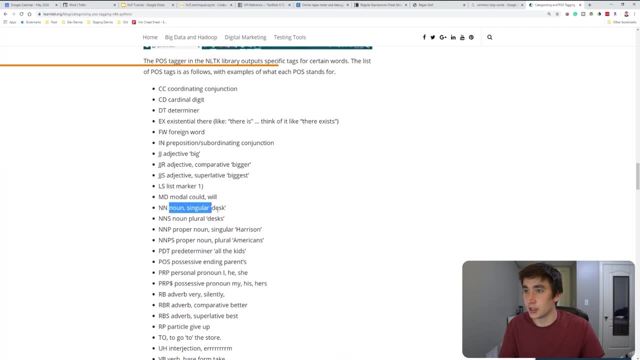 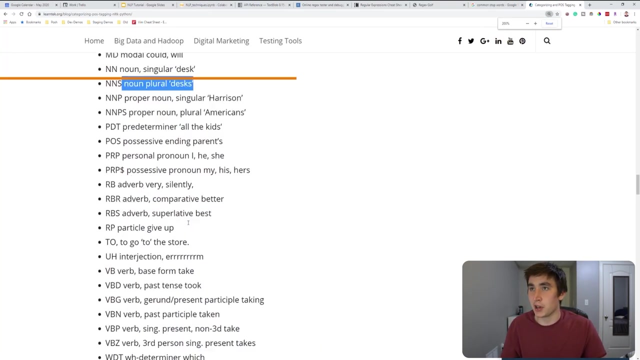 Um adverb, like we can just kind of look through this and help us find. So. this is a terminer. the DT uh noun Noun is a singular noun. Noun S is plural Uh. so yeah, this has all sorts of uh useful information right here. 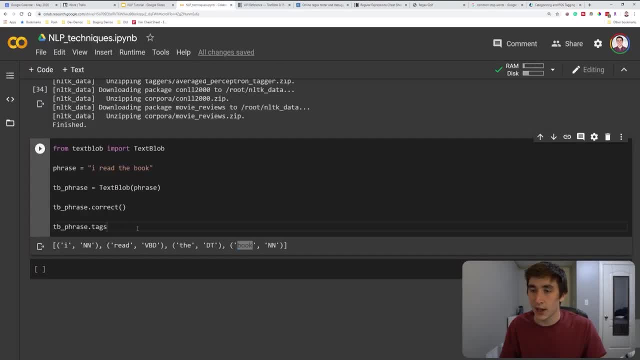 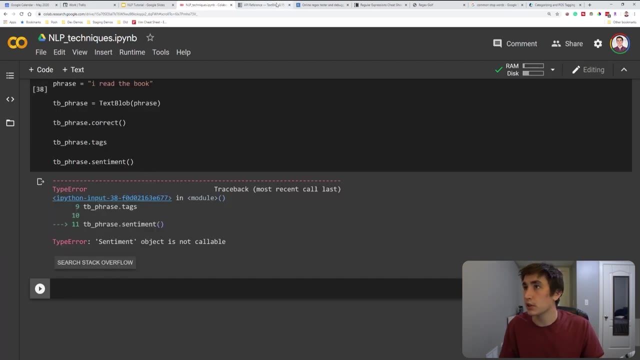 So I'll link this to if you want to know more about the tags here. Another cool thing is we can do dot sentiment. Um, you might have to do a sentiment like this: Uh, let's see. go back to the reference. 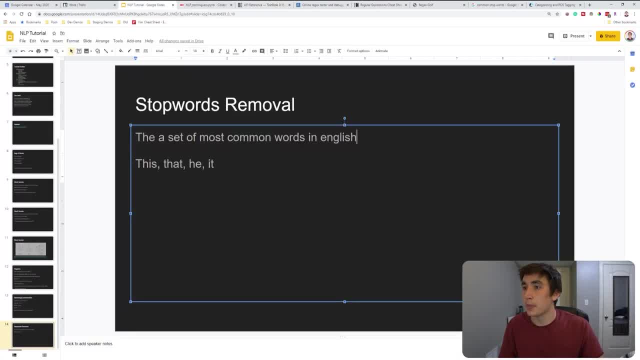 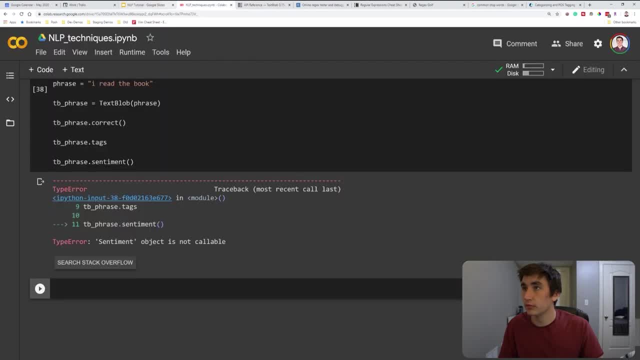 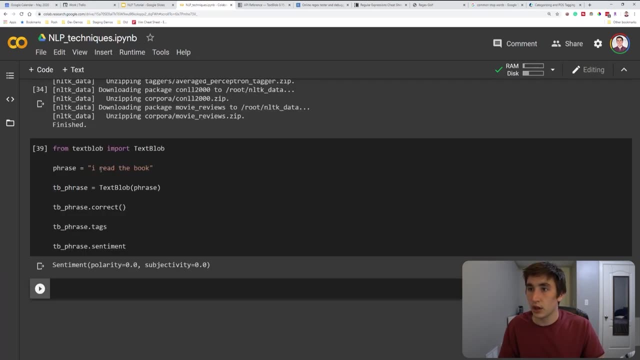 Yeah, it's just that sentiment. Okay, Um So, uh, so the book was great. Um, polarity 0.8.. So high numbers here are going to mean positive. but if I say the book sucked was so bad, right there we see that has a negative sentiment, because this is a. 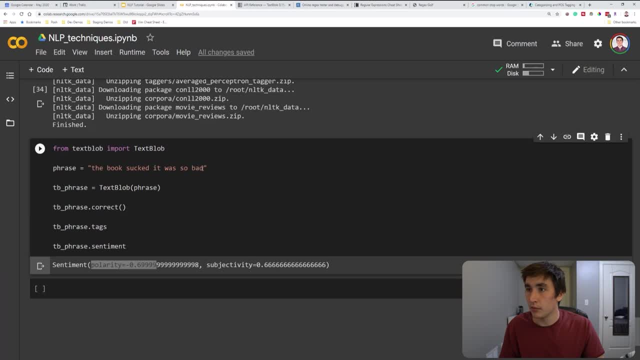 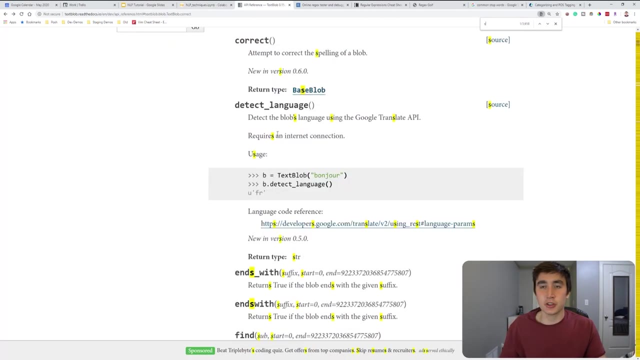 you know negative value here in the polarity. the book is another example. the book was horrible. another negative example here. so you can look into the details of the sentiment to see that. but yeah, in this API reference for text blob there's all sorts of really accessible, easy things you can do, so it's another. 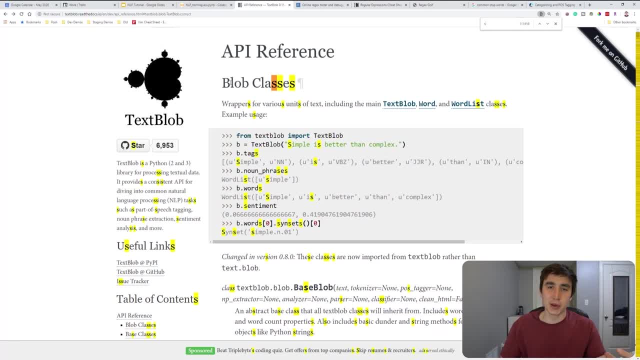 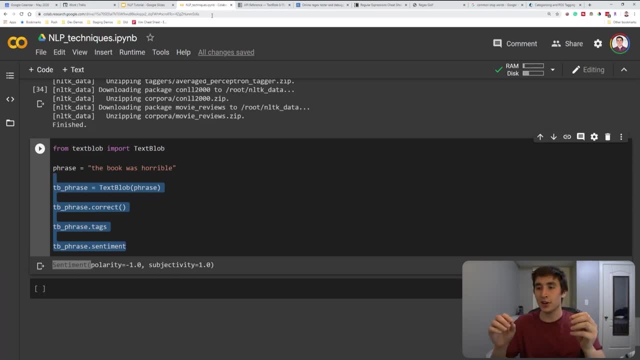 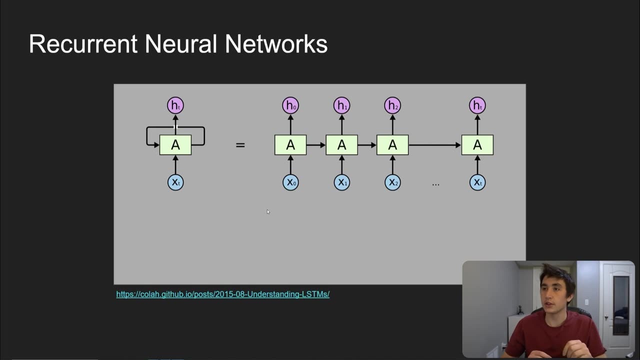 great resource to utilize, and I just want to make the point of one of the main goals of this tutorial is to show you all these different things you can use so you can kind of build upon this knowledge and apply it as you see fit and your own tasks that you are working on, all right. so moving towards the kind 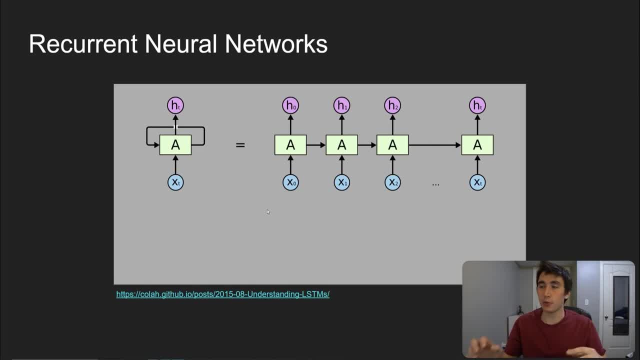 of state-of-the-art models in natural language processing. I wanted to start with recurrent neural networks. so, if you remember, back to word vectors, one of the issues that we had with them was that they were kind of set in stone and once you've trained your word vectors, no matter what way you utilize a word. 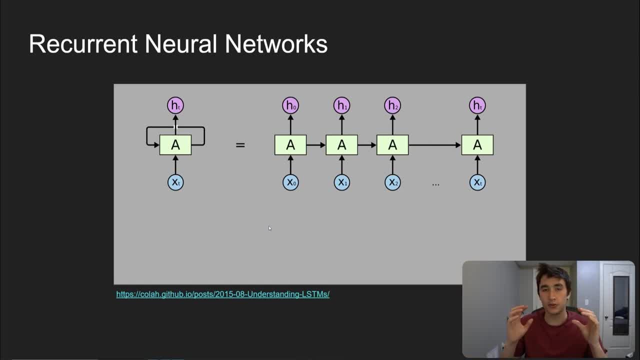 inside of a like bigger phrase. that word vector that you've trained is the same, so we don't have kind of context dependent word vectors when we're just using a preset trained of preset, a pre-trained set of word vectors out of the box, so immediately recurrent neural. 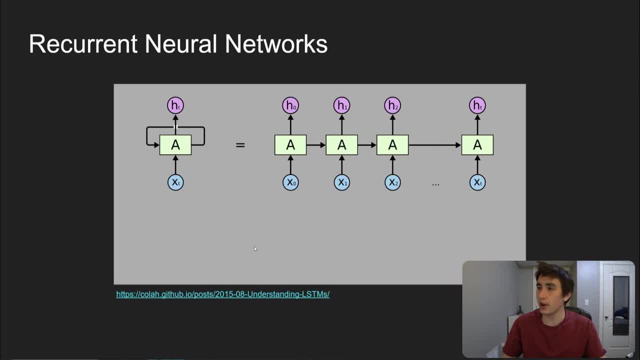 networks can help us kind of solve that problem. so here I have a diagram of a recurrent neural network and so basically how a recurrent neural network would work with language is we would feed in words into the network, one at a time, so we would have something like: you know, the word check come into our. 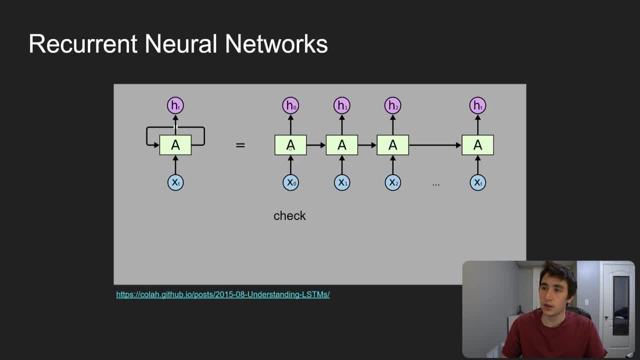 network and so that would come in, the network, would process it and produce the hidden state based off of it and also feed that hidden state to the next, you know, layer of the recurrent neural network. so maybe the next word is out, and so that now we have check and out all feeding into the same network. 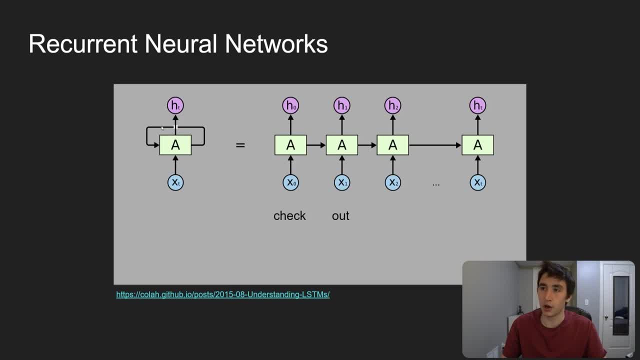 basically we can do this as much as we want. we're always feeding the output from the last input back into the network so we have check out the book. so basically you know we're feeding this in and creating some sort of at the end of book will get some sort of final hidden. 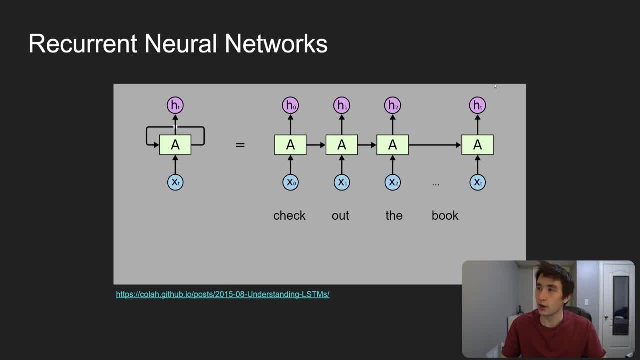 state, and we can use this hidden state in NLP applications, and so what's nice about this is if we had another phrase that was: write me a check. well, the way that check used here is at the start of the sentence. there's no other words around. 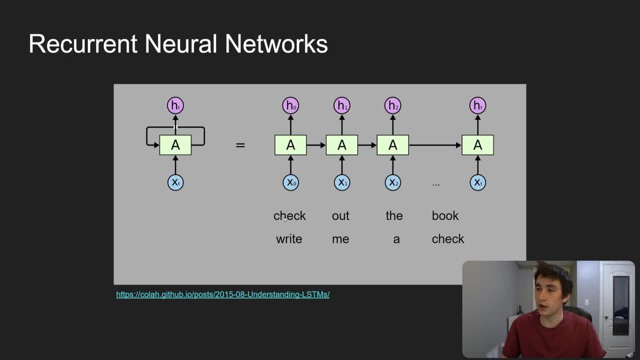 it and you're going to get a different kind of embedding for this check, then you will. when it says, write me a check based on the context of write me a, you know the embedding this final hidden statement be more related to banking versus check out the book. would be kind of a more related to a hidden state that. 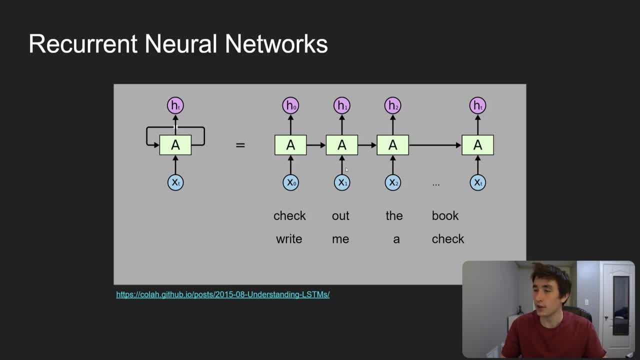 more represents check as in, check it out, so that's like a little toy example, but that's ultimately like one of our goals, with something like a recurrent neural network. but the recurrent neural network, you know, for a while this was kind of the go-to to build all sorts of state-of-the-art language models, but it 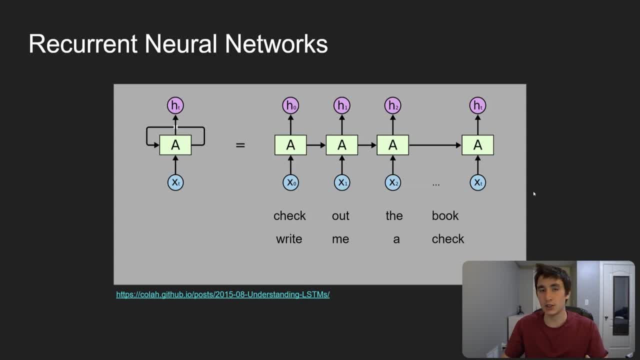 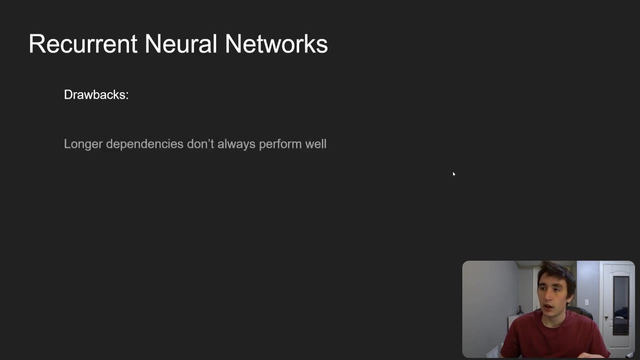 did have some drawbacks, which ultimately got replaced by, like the open AI GPT to model I introduced at the start of the video, and some other other types of models. so what are those drawbacks? well, the first one, I would say, is that the long dependencies don't always work well with a recurrent neural network. so imagine you. 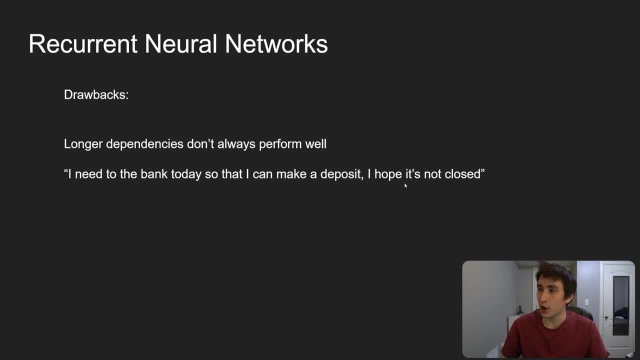 have the sentence like: I need to go to the bank today so that I can make a deposit. I hope it's not closed while we are feeding in. we would be feeding in each of these words to the network and, like always, that hidden state would have had some influence from each of these words. 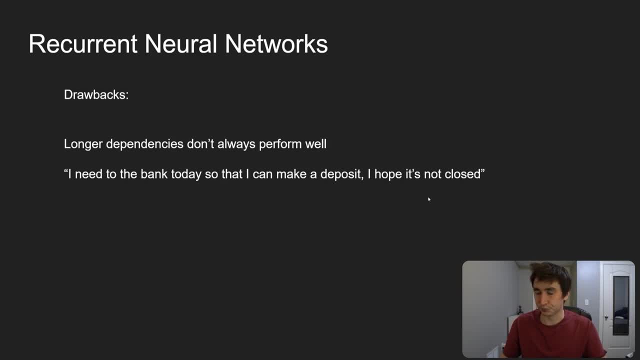 by the time we get to closed, a word like bank is pretty far away. so in the final output embedding that hidden state, it might not be clear to the network that the thing that we're talking about that is closed, is the bank because it's so far away in this sentence. so that's one drawback with recurrent neural. 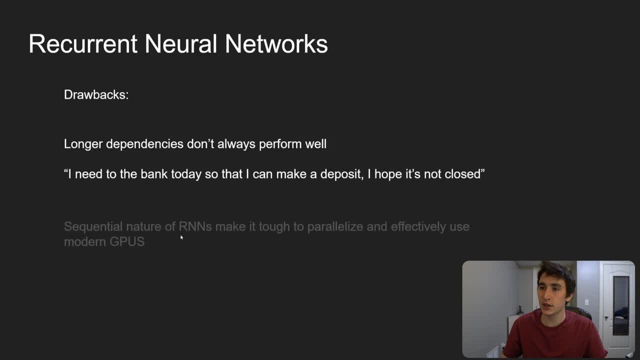 networks. another drawback is more on a performance side of things- is that because we're feeding these one token at a time, the sequential nature of that is that makes it tough to paralyze the training and utilization of RNNs and language models. sometimes, and you know, we can't as effectively utilize modern. 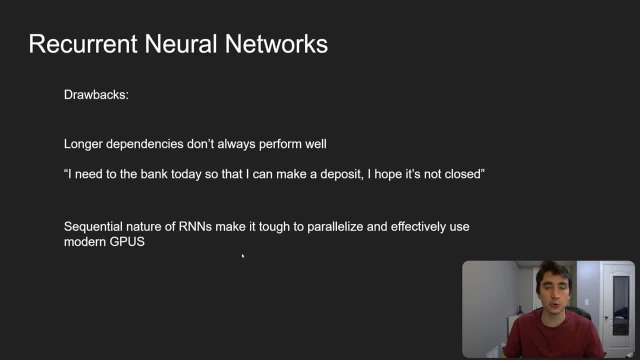 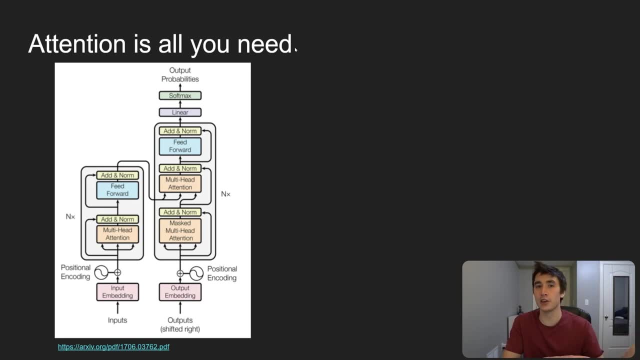 GPUs right. so that leads us into attention, and a big paper that came out was called attention is all you need, and this kind of set off a whole new wave in natural language processing. so what is the difference with attention? well, basically, you can feed in a phrase and as you iterate through the tokens in that phrase and 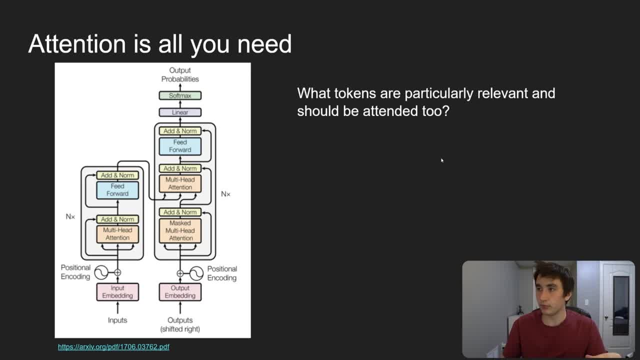 you can basically figure out what needs to be attended to. so, if you like, walk through this sentence: I need to go to the bank and write a check. well, you know, right, when we get to the word, when we get to the word check, let's say we're. 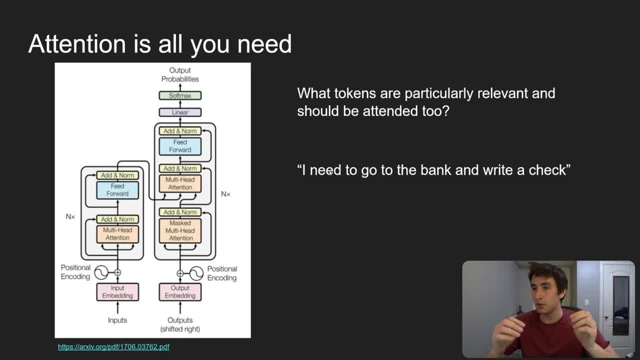 feeding these all in. and this is all being fed in at the same time using these positional encoding, so it doesn't have to be one after the other. but basically, if you get to a word like check, well, we can, it will probably spike off write and bank as like relevant items to check. I need to go go might. 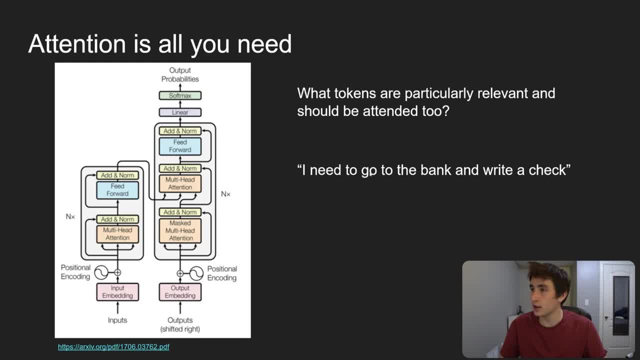 like set off. if you're looking ahead, bank might be triggered as like an important indicator to go. you basically were based on what word we're looking at. our network kind of learns to attend to other words and figure out what's most important given a certain token that we're looking at, and to kind of bring that to a high level. the 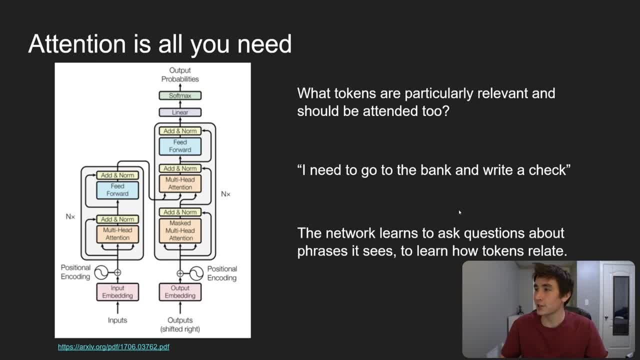 network we can kind of think of, learns to ask questions about phrases it sees. and these are not you know, they're not actually asking you know, human questions, but baked into these attention networks, They're basically looking at each token, asking all sorts of questions on that token. 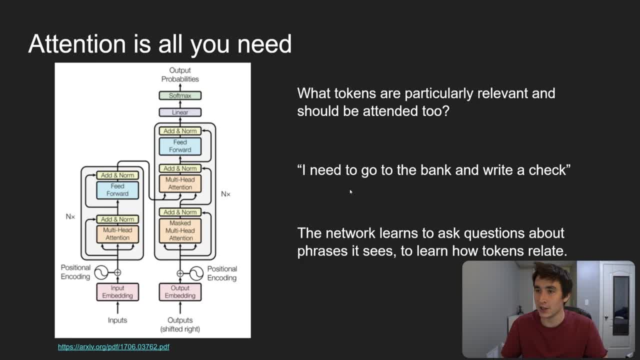 and learning. based on that token, what else is important in the phrase? And this is a super powerful technique And also this attention can work at a longer range of dependencies than in a traditional RNN, So this set off all sorts of really impressive stuff. 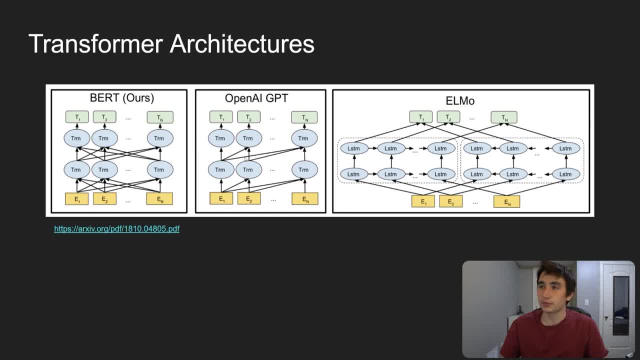 in the NLP world. So the story of the video: I mentioned the OpenAI GPT-2 architecture. One thing to note about that is it's a forward nature. So basically, the task that this is trained on is language modeling. So, given some words, 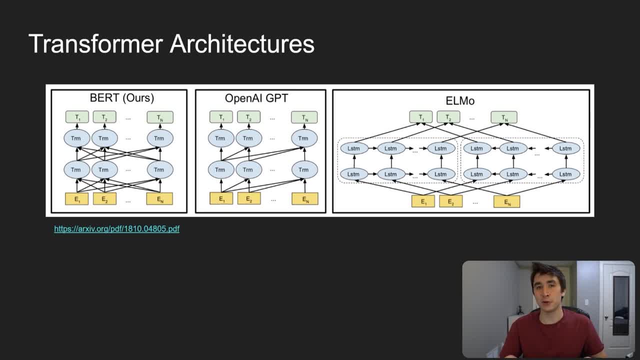 what are the words that are coming after it, And that's why it was really good at being able to auto-complete like a story And when I typed in a phrase, it could utilize the fact that it's been trained on figuring out, on predicting what the next word should be. 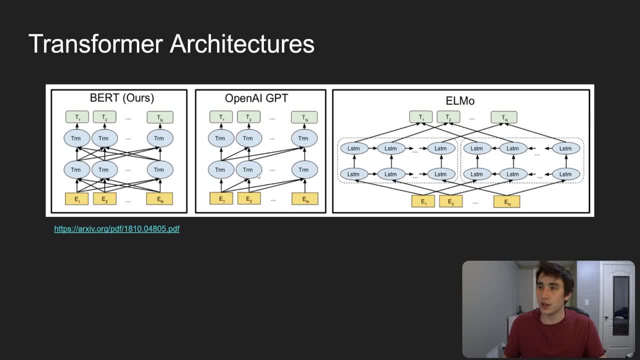 based on what it's already seen. So that's OpenAI GPT-2.. Then there's this ELMO network that's also listed here. I just wanted to note this one. I don't know as much about ELMO network, but one thing to note is that it uses LSTMs. 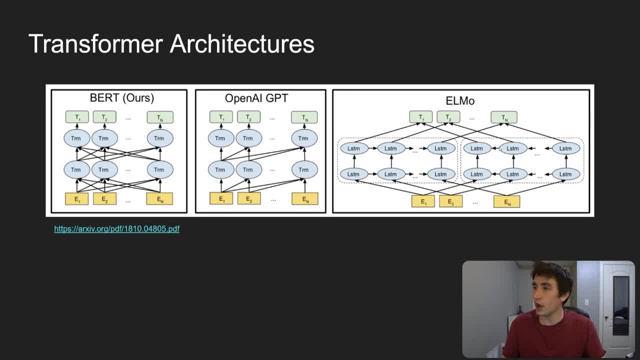 and it's kind of the core of it. And an LSTM is a type of recurrent neural network. It's supposed to to handle longer dependencies a bit better, but still compared to attention, And actually, and actually I wrote the header as this: 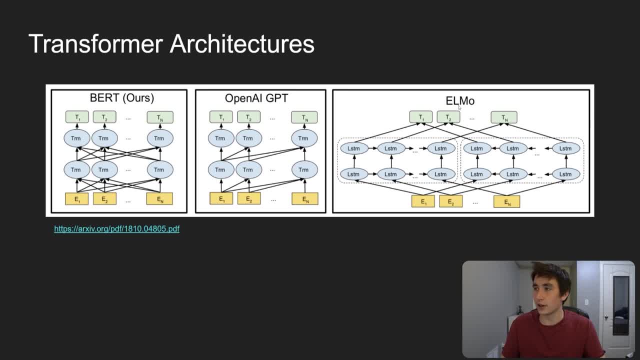 as transformer architectures, but ELMO was not technically a transformer architecture, It's just another powerful language model. And then, finally, what we're gonna focus on right now is BERT, which is a bi-directional transformer architecture And, as a result of it being bi-directional, 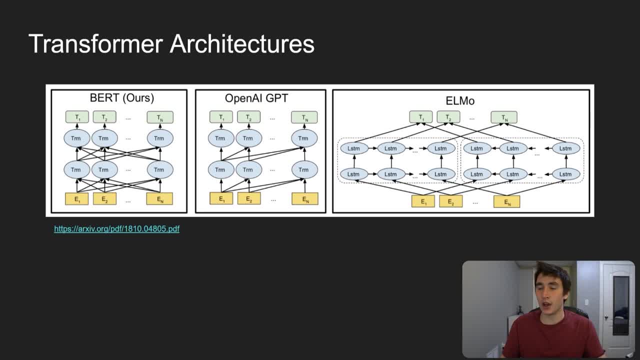 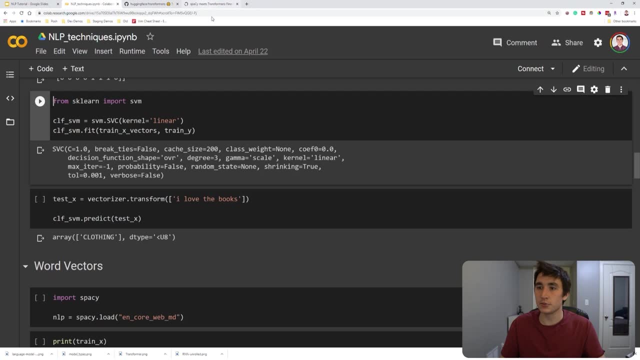 it really captures a lot of very impressive things about language that even like the OpenAI GPT model can't. So we're gonna just look at how we can use Python to interact with the BERT model real quick. Okay, so to do this we're gonna use spaCy again. 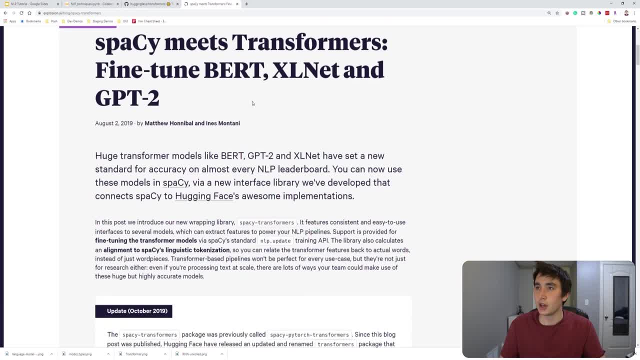 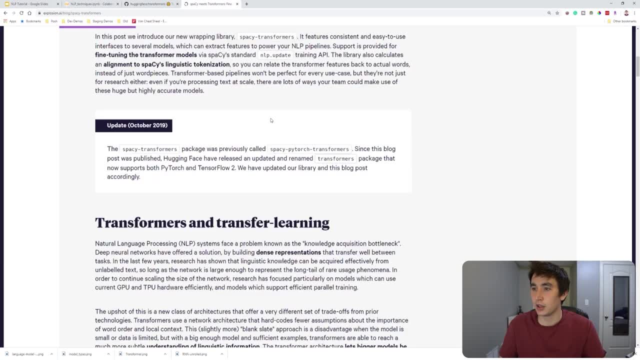 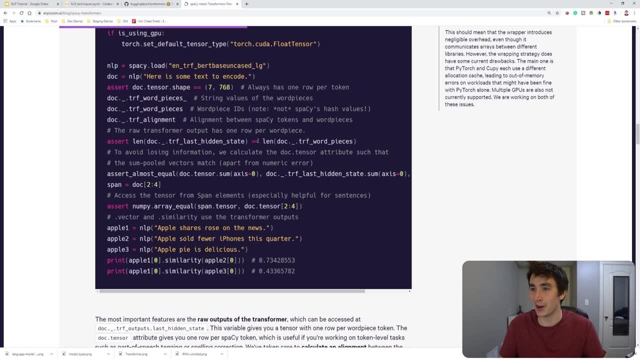 So I'll link this article on my GitHub page. But basically, spaCy provides us with a really easy way to interact with transformers And if you just follow this link, basically it gives you all the lines you need very quickly to get up and running. 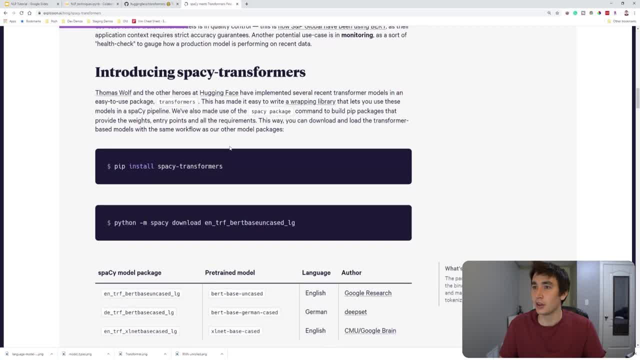 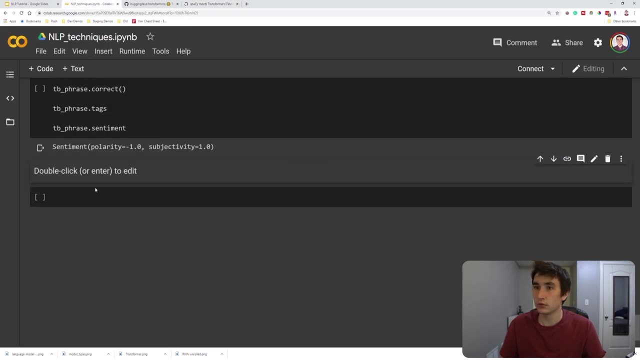 So let's utilize spaCy real quick. So the first two things we're gonna need to do is pip install spaCy transformers and python-m spaCy download this model. Okay, So I wanna make a title, not an italicized title: Transformer architectures. I'll say: 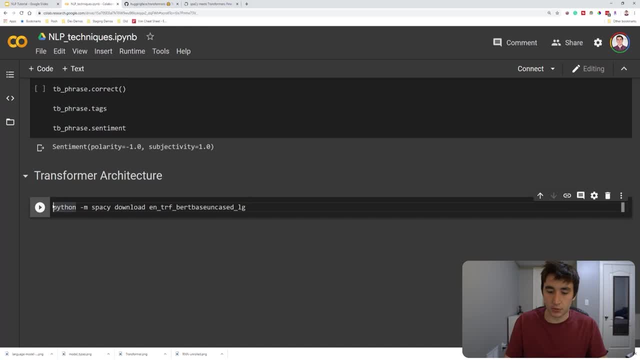 All right. so we wanted to download this large model and we also wanted to do a pip install of spaCy transformers. So we're gonna do a pip install of spaCy transformers. And what these explanation points mean, I'm pretty sure, is that this should only 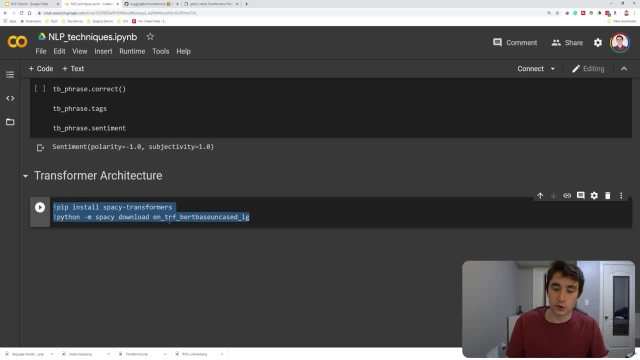 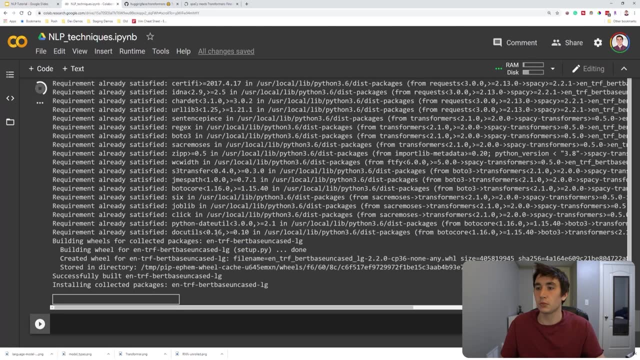 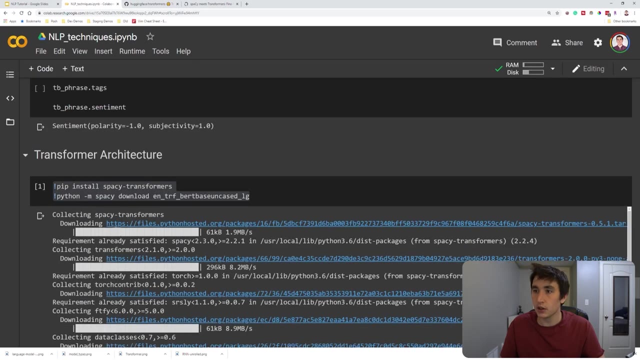 this cell should only be run once within Google Collab, So we don't accidentally download the model again. Okay, downloaded and took a little while, but ran successfully. Cool, All right. and now? how do we actually, now that we have it downloaded? 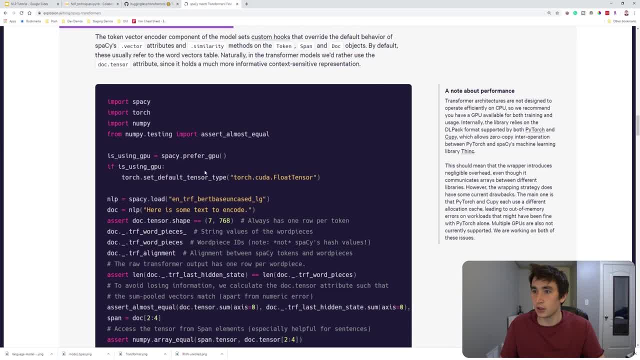 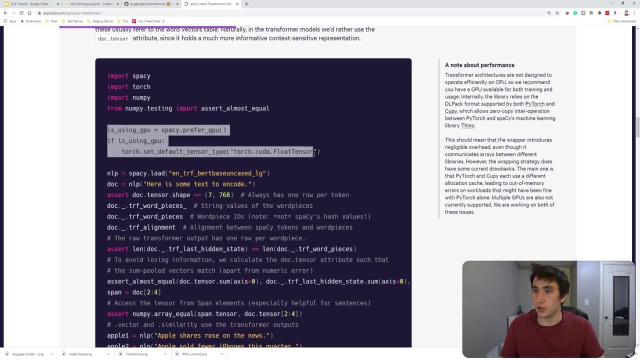 we can go back to that article and see how we can actually use it. It looks pretty straightforward And you can. if you're using a GPU, you could utilize these lines of code and you'll note some details about that. I'm gonna just I'll copy this in real quick. 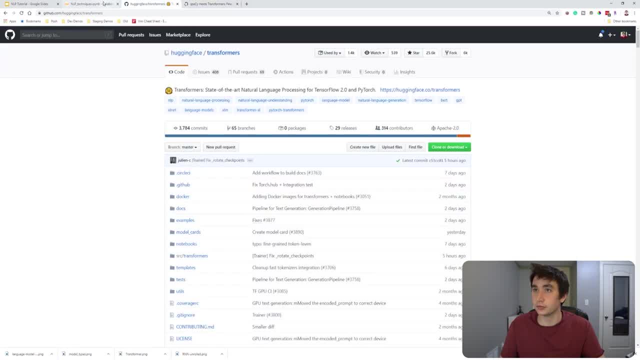 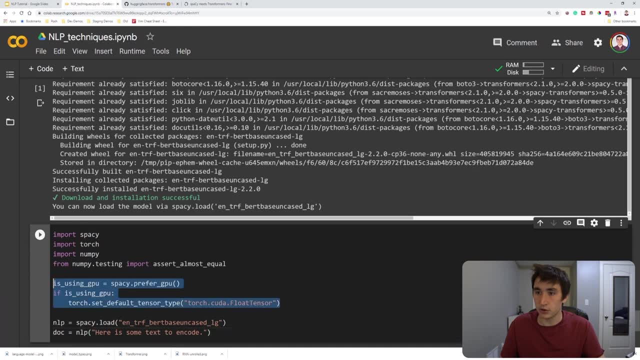 I think all I need is gonna be- I'm not gonna use this right now, I'm not gonna use my GPU, Don't think we need NumPy right now. So I think you need to import spaCy and Torch, and it should be good. 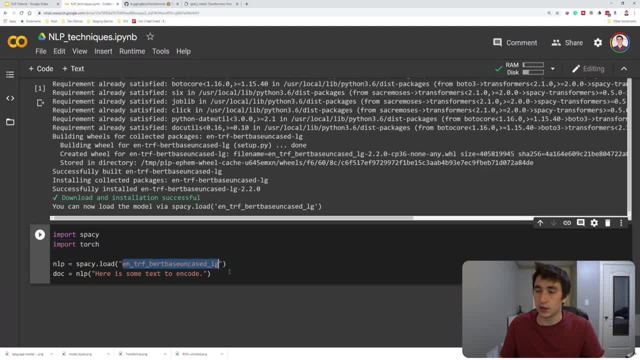 And then we're loading this large BERT model. And one thing to note about when we're using transformers: when we're using transformers, we're not gonna train it. When we're using like BERT model, we're not gonna probably train it from scratch. 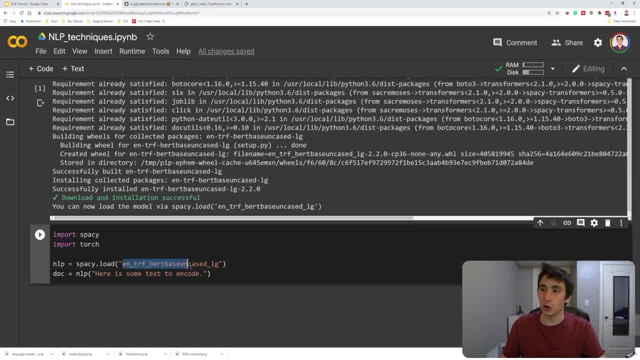 The BERT model itself is super, super massive. It takes multiple days on, like some of the most powerful tensor processing unit machines, to train this model. So it's not something you're gonna wanna do at home, But luckily they open source these models. 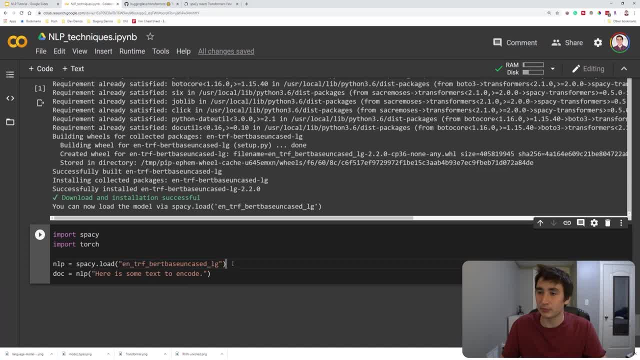 and we can utilize them effectively. And one thing to note, too, is that even if you are loading in this model, that's already been pre-trained. One of the nice features about one of the nice features about models like this is that they can be fine tuned. 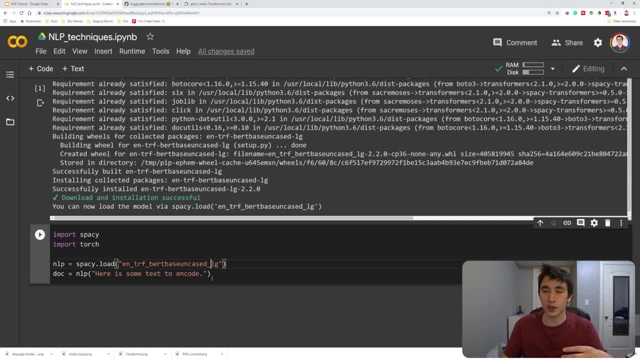 So you can fine tune them on your specific task and you can get some really impressive results by doing that, And that's a lot easier of a step than retraining it from scratch. Okay, so run this. see if it loads properly If you're using Google collab. 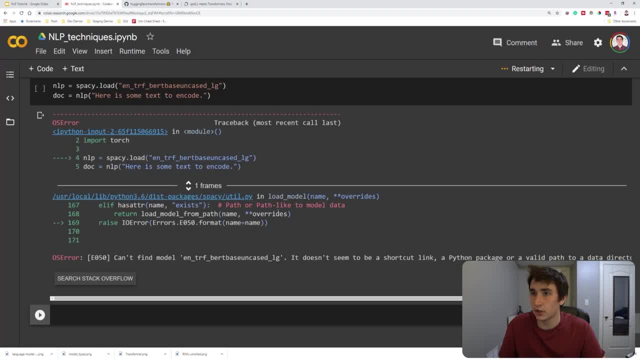 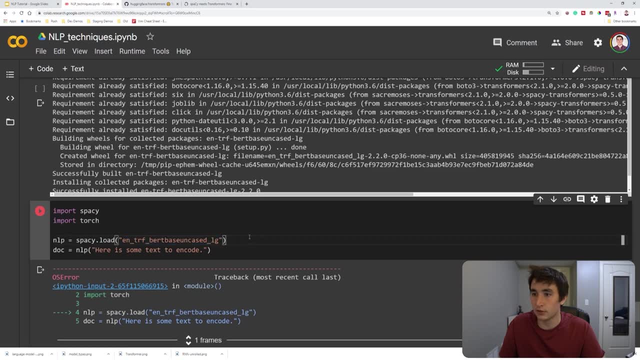 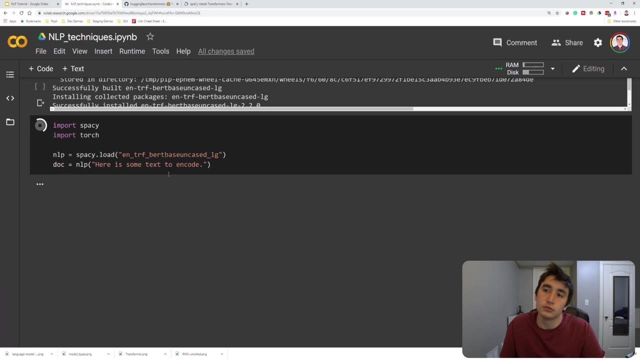 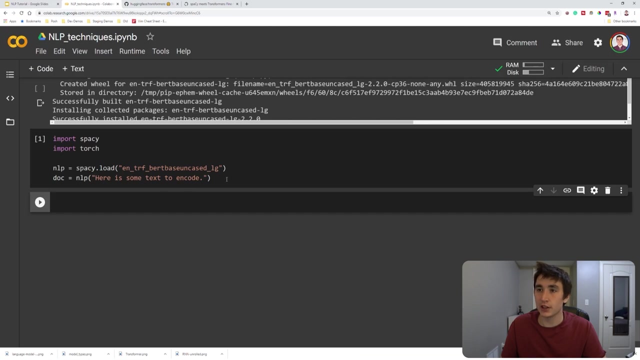 you probably have to restart the runtime. Sometimes it doesn't realize where this model is, unless you do that. Okay, cool, we have it, And now it's just like. it is like if we're using spaCy, now that we've loaded in this. 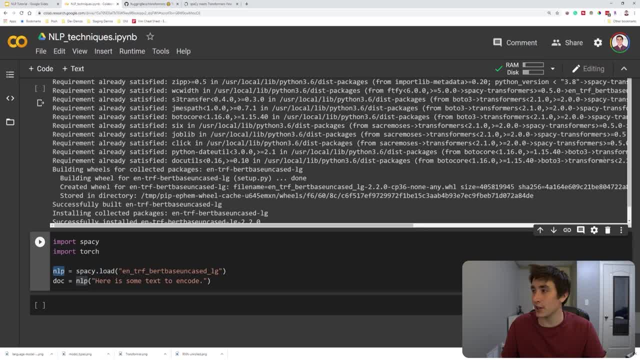 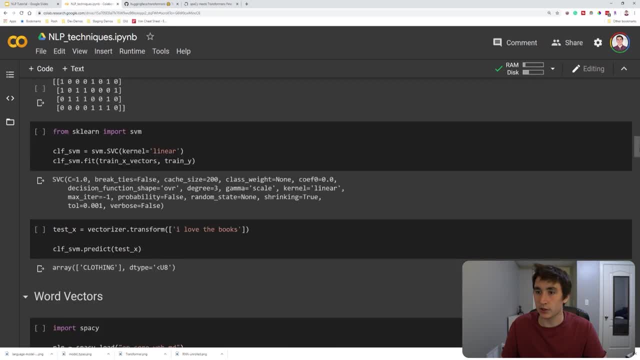 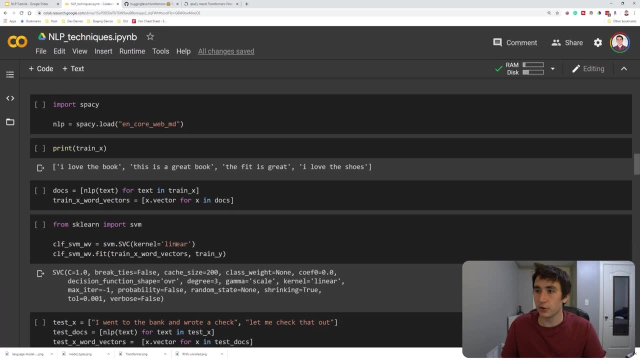 BERT model as our NLP engine. basically, we can do the exact same stuff as we did for the word vectors when we were in that section of the tutorial. So here we go. So basically, what I think I'm gonna do is just to find another set of training utterances. 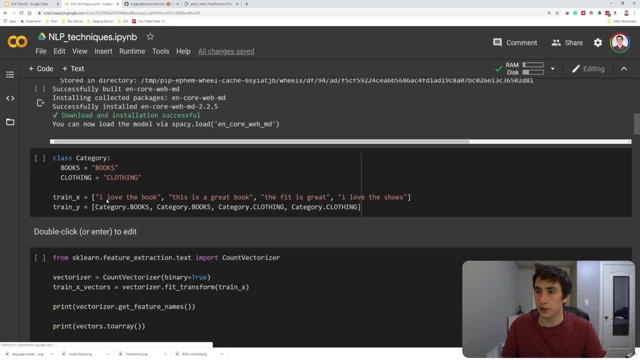 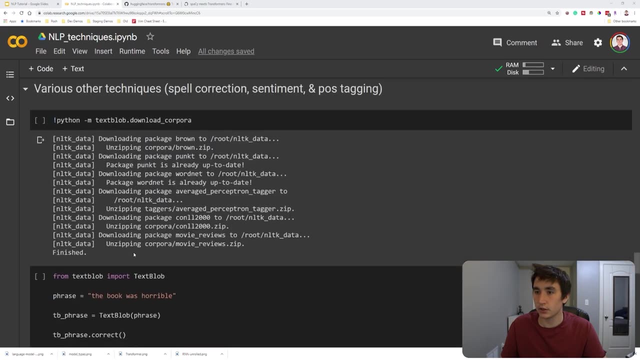 and test utterances, just like we did here. I'm actually gonna copy this in real quick, because I don't think it's necessary to write it, because I want to change the example up a little bit. All right, So we're about to see the power of BERT. 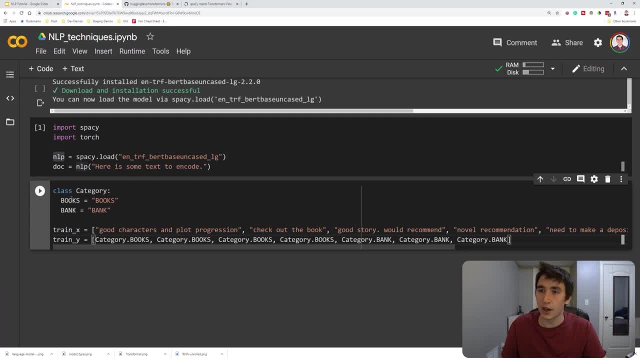 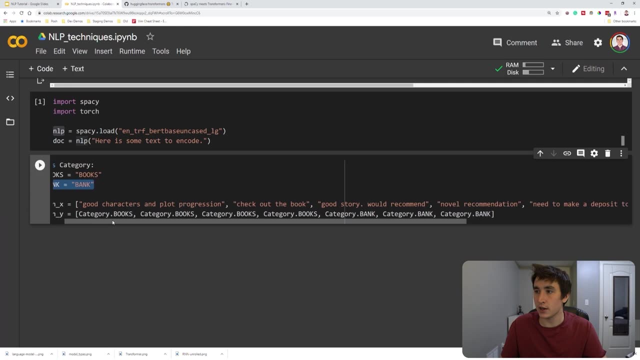 and transformers in general. Okay, so this time I am defining another category class, but this time, instead of the difference between books and clothing, our two categories are book related items and banking related items. So here we've defined seven different utterances. 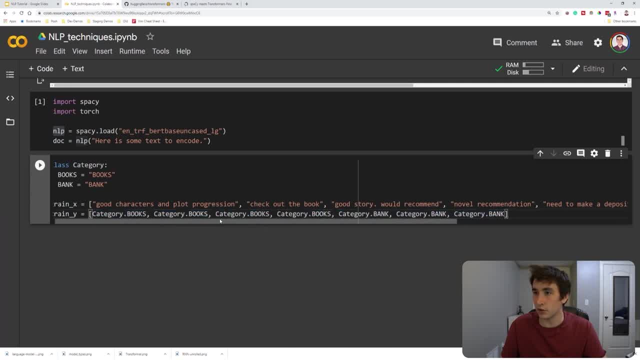 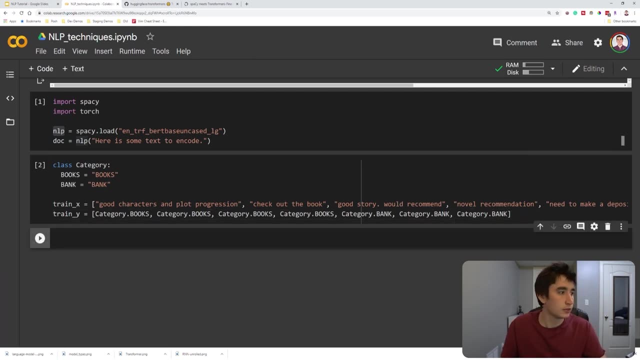 each with their associated category, And we can read through these real quick. Okay, cool. So let's build our model around this, And this is the exact same code, basically, that we used before. We just need to now. all it changes is that we have this model as our NLP engine. 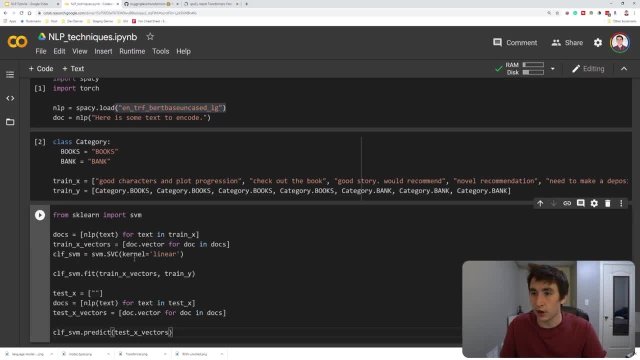 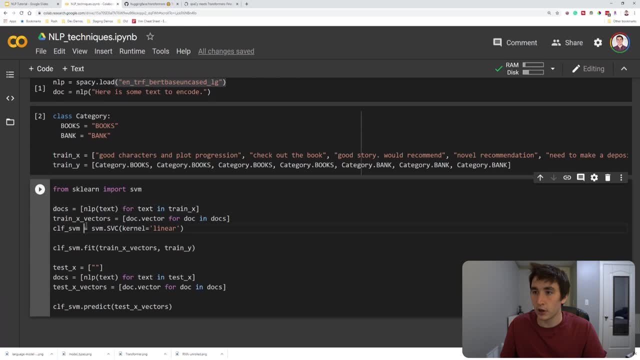 as opposed to the word vectors that we were using earlier. Okay, so I'm just copying in some code here. This is: yeah, as I said before, this is the exact same code as we were using before, So we can train it on the train X here. 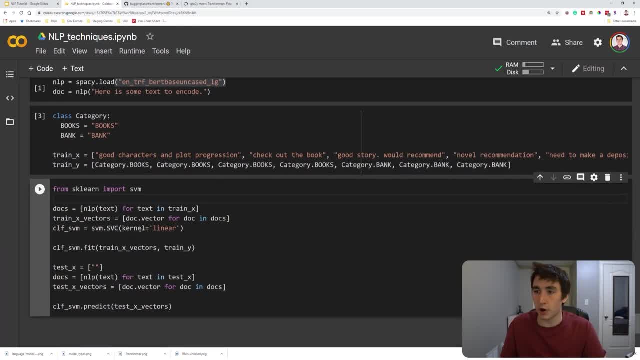 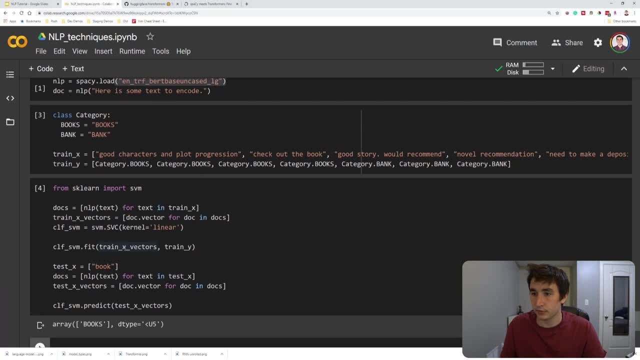 So I'm gonna run this cell real quick, So we're gonna wanna train our model on that and we can predict new utterances here. So I'm gonna just start as a toy example. say book Okay, and as a result it says books here. 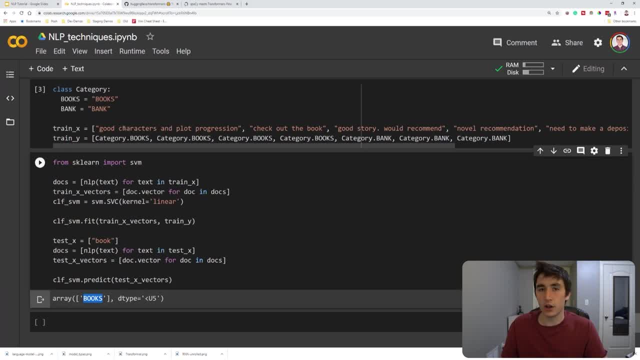 That's what we expect. One thing I wanna note here, though, is one of our training utterances is check out the book, And so, with that example I was kind of walking through, is you could say, check out the book, but if maybe you're writing about more banking related terms, 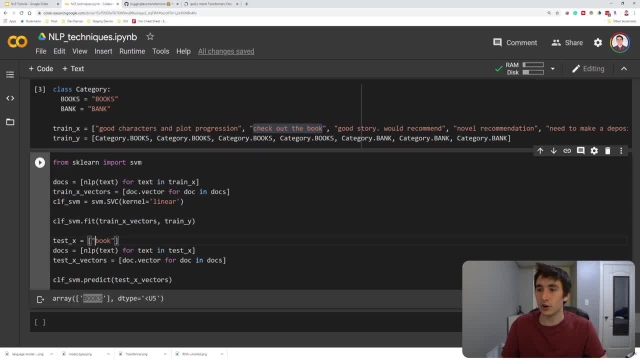 you might say: I need to write a check. So I'm gonna just, I'm gonna just type in: you know I need to write a check And you know, in our trading utterances here check, the word check only appears in. 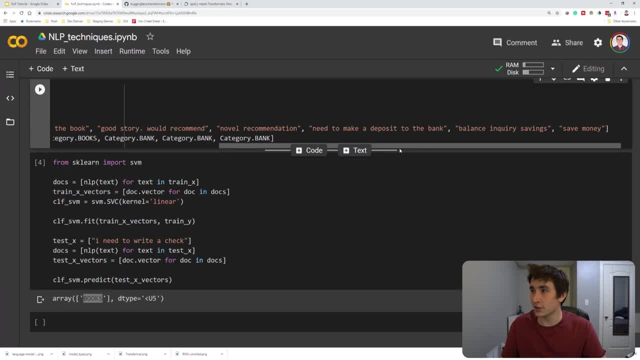 the books category of our trading utterances, And these three back here that are about banking need to make a deposit to the bank balance. inquiry savings, save money. There's no mention of the word check, So a true test of the power of the book. 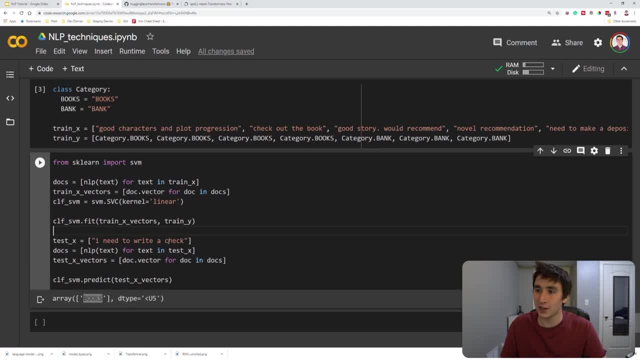 a true test of the power of this BERT model is that. oh, does it know that when we say I need to write a check, we're talking about banking and not talking about this word? we've already seen in the other category. 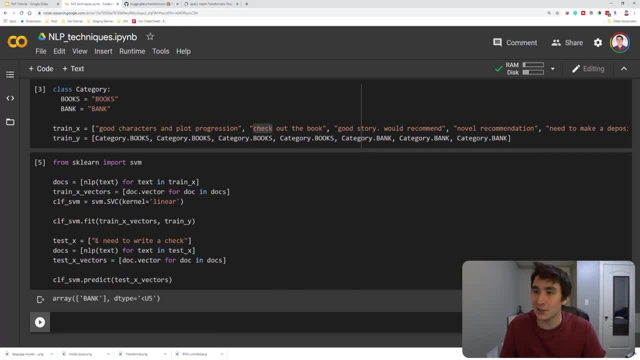 And let's mode of truth And look at that. I need to write a check Utilizing the power of the BERT model And, just like some small number of training examples, we see that it's banking related, which is crazy. 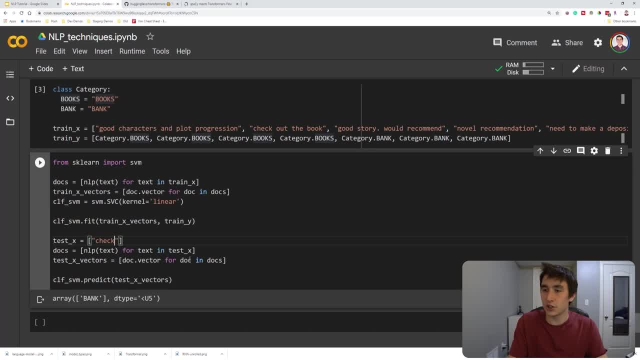 And you know, maybe you said check this story out. You know once again it knows that check in this context is is about books. So it's really impressive the capabilities because we've trained such a big model leveraging. it is really really powerful stuff. 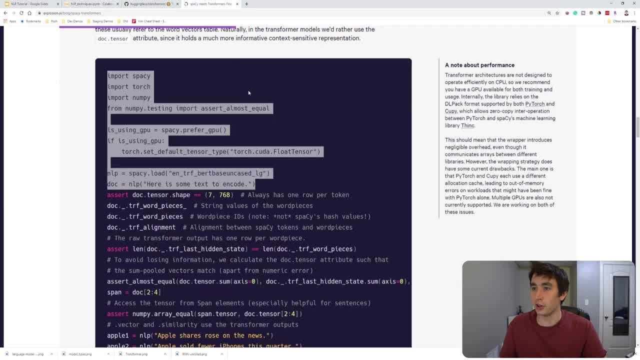 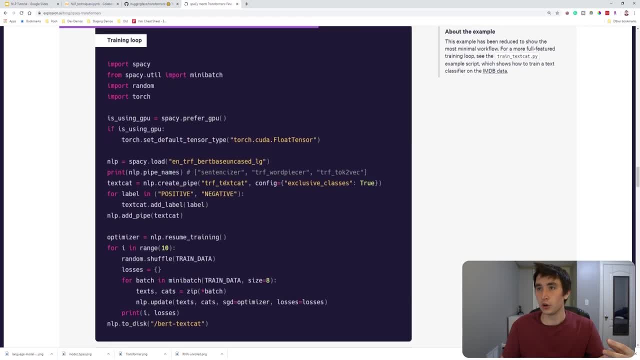 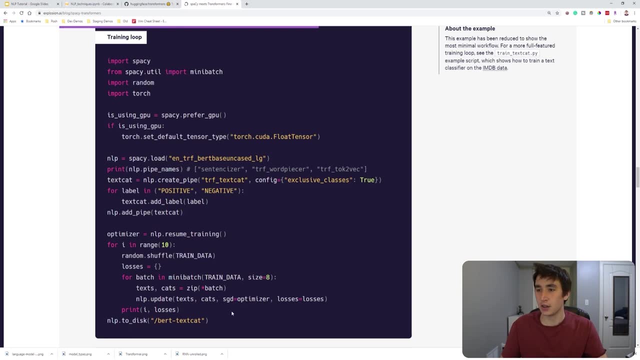 And you can continue playing with this. One thing I recommend looking into, as I kind of alluded to, is one of the nice things that you can do with a pre-trained model like BERT here is you can fine tune it to a specific task. 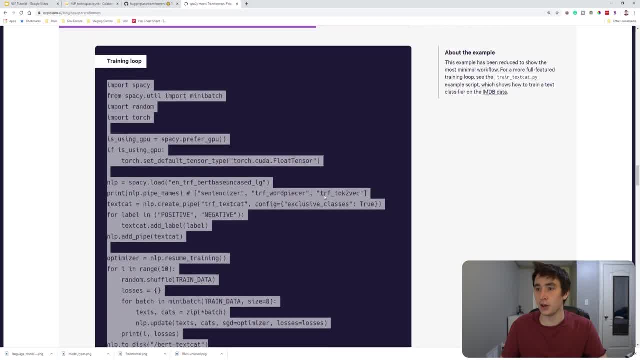 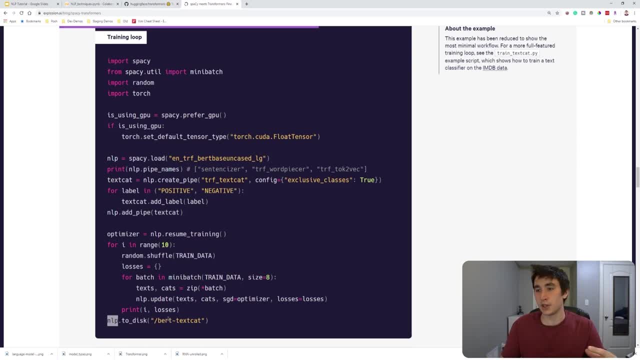 So here's some code that they use in spaCy to show you how you would fine tune this NLP you know model to a specific, you know maybe, classification task. So that's really useful. The next thing I want to mention is this: 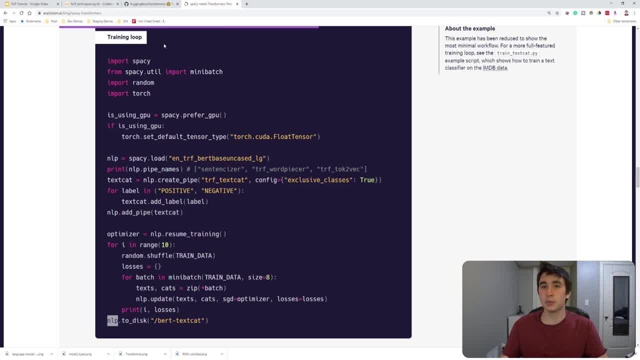 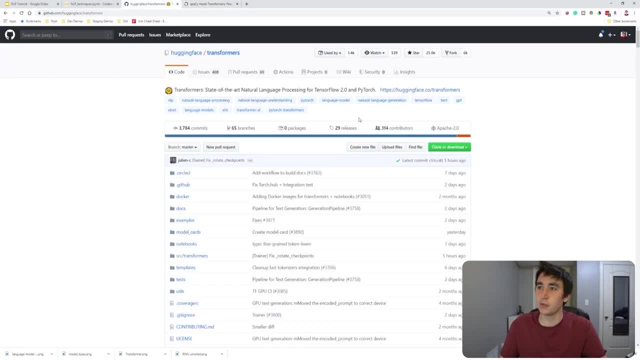 this interface that spaCy provides to BERT is really nice, but there definitely is room that if you wanted to build off of a model like BERT, you can't really do that. So if you wanted to dive deeper into these types of models, I recommend checking out HuggingFace's Transformers GitHub repo And in that they have pretty much all of the most popular you know, And in that they have pretty much all of the most popular different models that have come out recently within natural language processing. 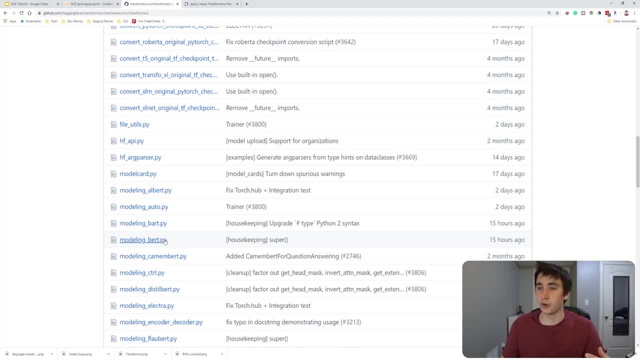 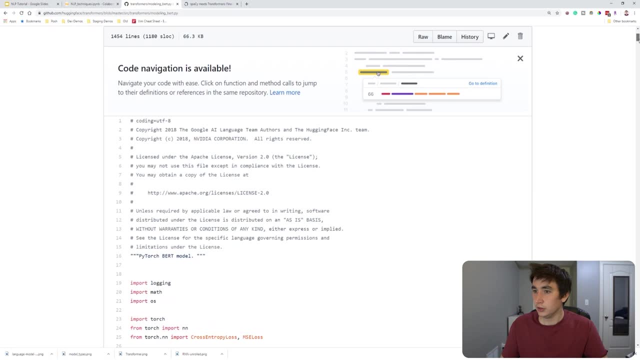 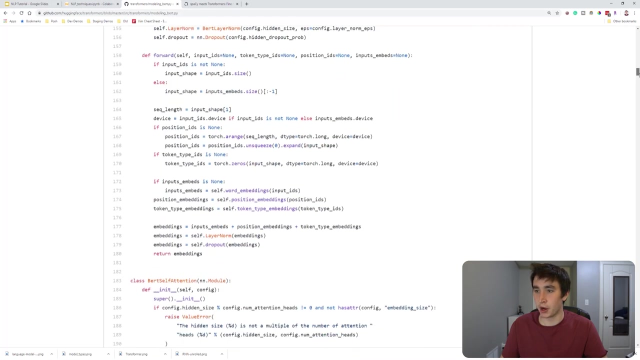 They have those models written in PyTorch that you can look around with. So, like BERT here, this modeling BERT file, you'll see that pretty much a entire PyTorch model is defined here. So if you wanted to build off of BERT, 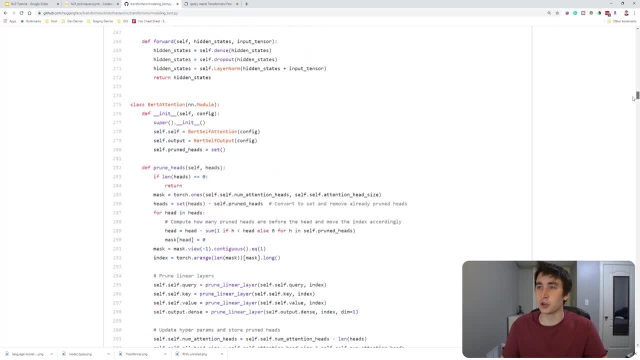 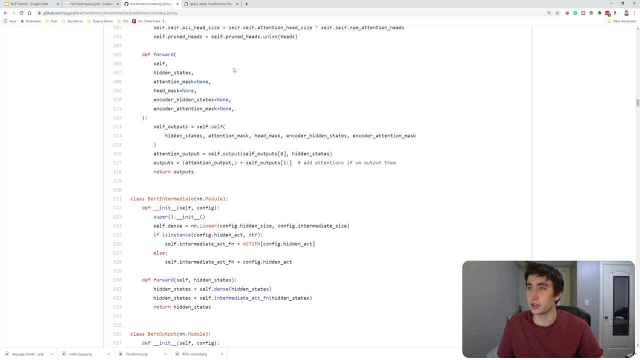 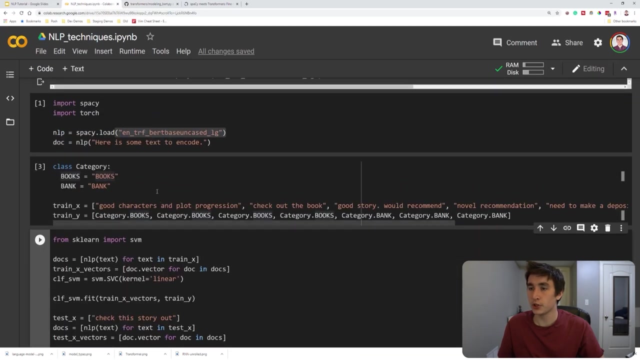 and you know, fine, tune it specifically or something. you could use this HuggingFace library, All right. so that's what we're going to talk about for Transformers and how the code would look to easily interface with that, And one thing I want to note is that 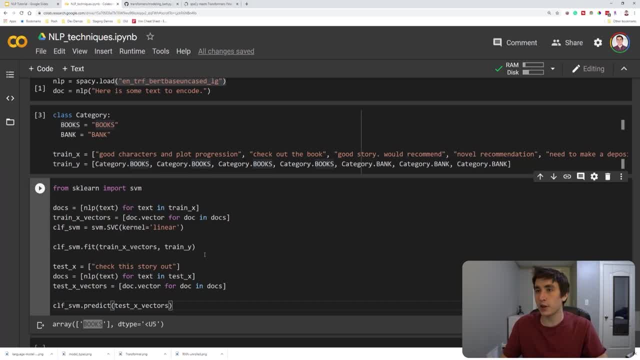 I can only teach you so much about the actual inner workings of BERT. in this tutorial I was kind of more focusing on quickly getting up to speed and using this in Python, but I will list out on the GitHub repo resources that you can go to learn more about these types of things. 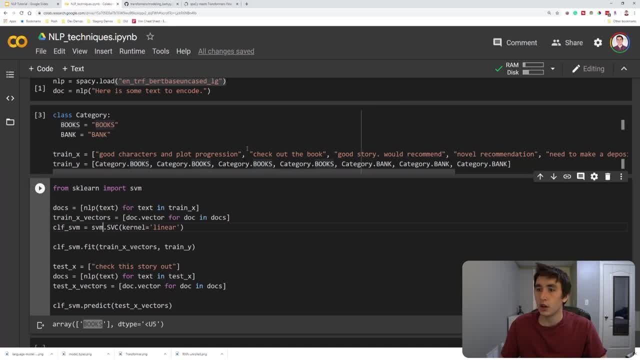 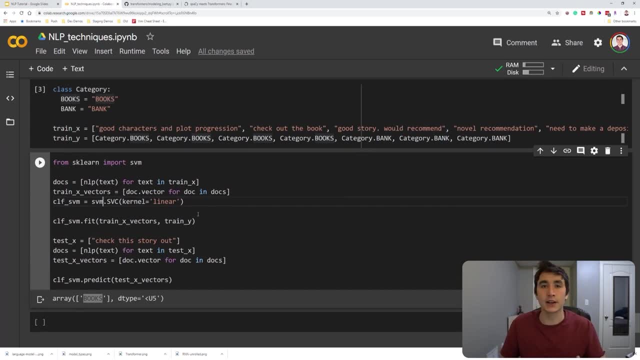 that I've found useful myself. All right, that concludes most of what we're actually going to do in the tutorial, but I will leave this tutorial with an exercise that you guys can kind of tie everything together and really try to build your like. 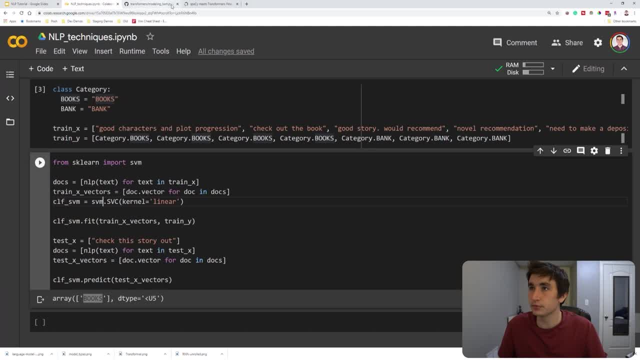 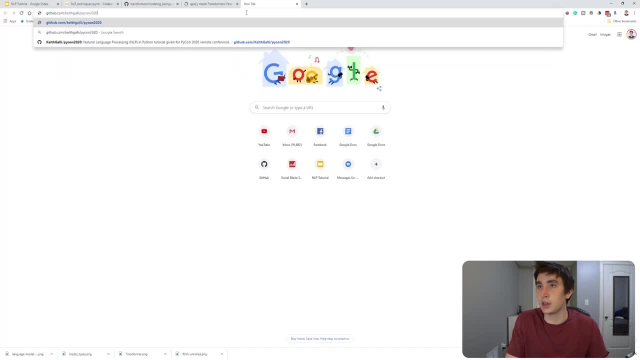 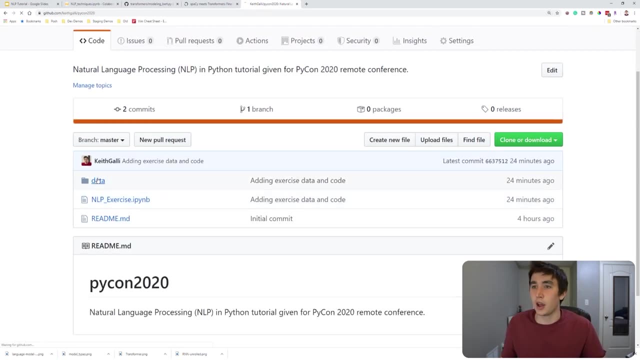 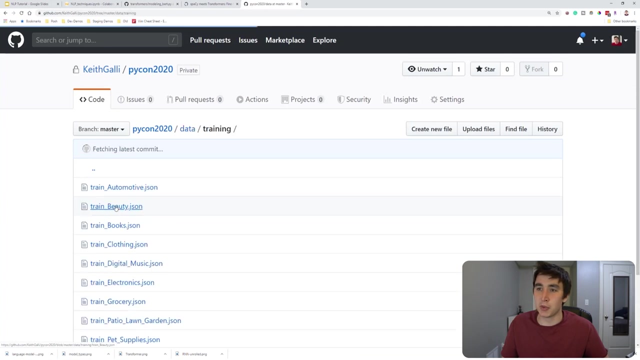 keep building on your NLP skills. So if you go to my GitHub page, githubcom- slash, keithgalley, slash, pycon 2020, basically, I've curated some data for a NLP exercise you can work on and the data it comes from Amazon reviews. 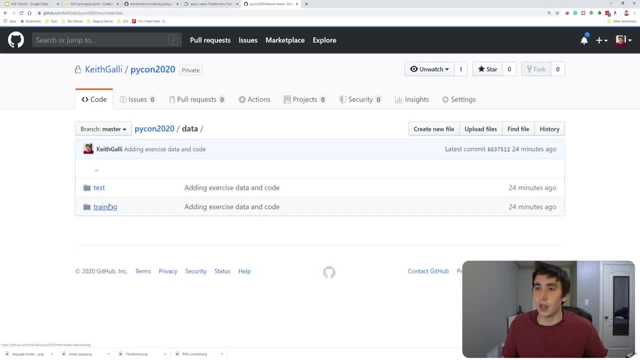 in several different categories And there's a link in the description. there's also a test set of Amazon data in several different categories- each the same categories- And the goal of this task is to basically use this training data and build the best classifier you can. 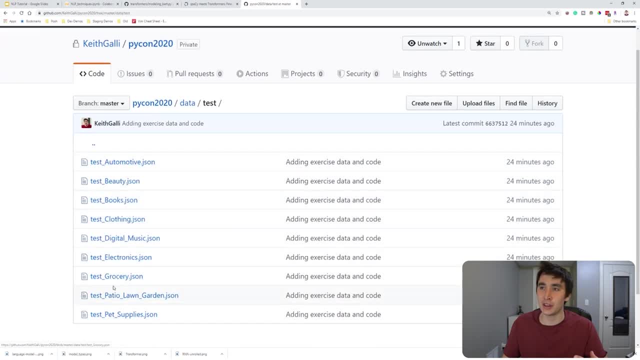 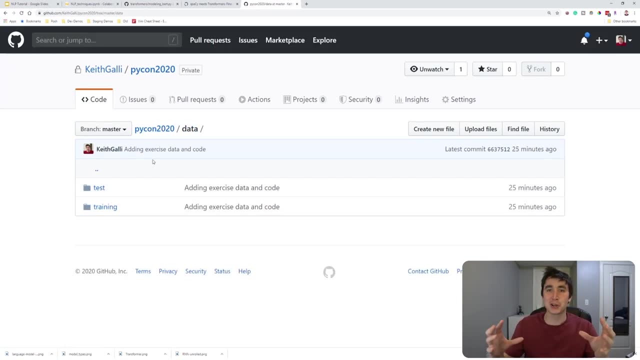 to properly categorize the reviews here in the test set. The kind of bigger picture context you could think about this problem in is: imagine you are in charge of the like social media analytics for a large retail store and you're getting people tweeting at you all the time. 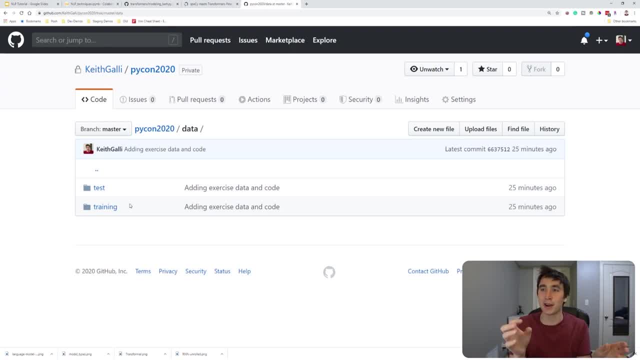 about all your different products And you wanted to build a model to automatically like route those tweets to the appropriate parties that could handle questions about them. then a model like this would be super useful. So there's the training and test data for that task. 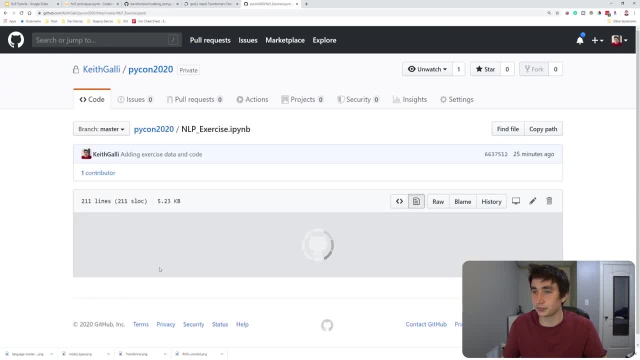 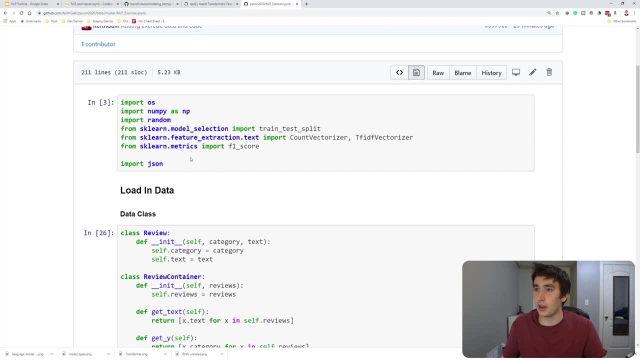 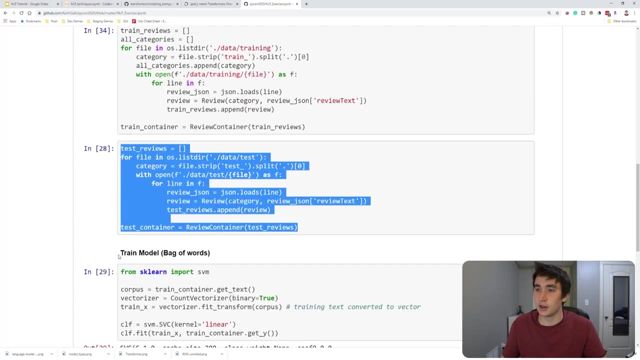 And I also provided this NLP exercise notebook and in this I kind of quickly walk through getting up and using this data, you know, loading it in as training data, loading in as test data, building a model on the training data, which by default the simplest model that I included here. 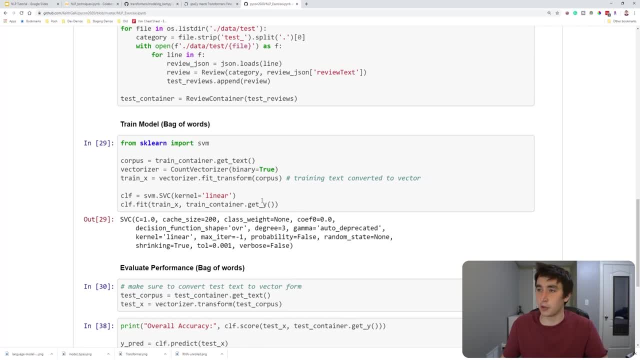 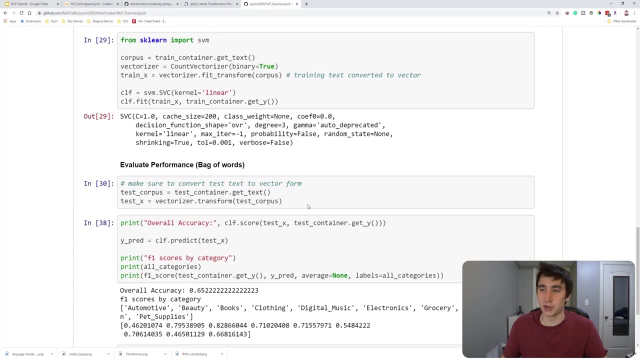 is a bag of words model, but I'm going to be kind of adding: by the time you probably see this video, I'll have met several models included in here, but this bag of words model can help you get started on using this data and then basically, based on that model, evaluate the performance on how you do on the. 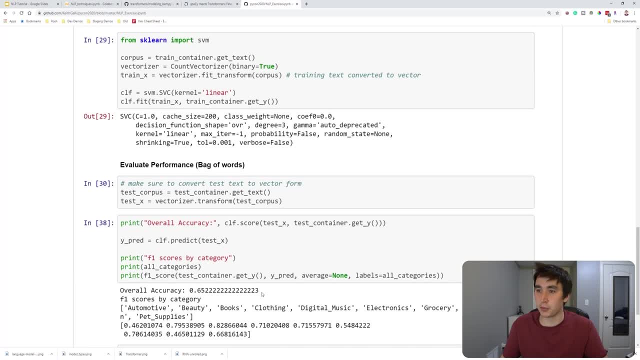 test set. so, as you can see out of the box bag of words, categorized 65% of the test reviews correctly into their category and if you wanted to break that down a little bit more closely, I calculated the f1 scores here for each category and, as you can see like it did, 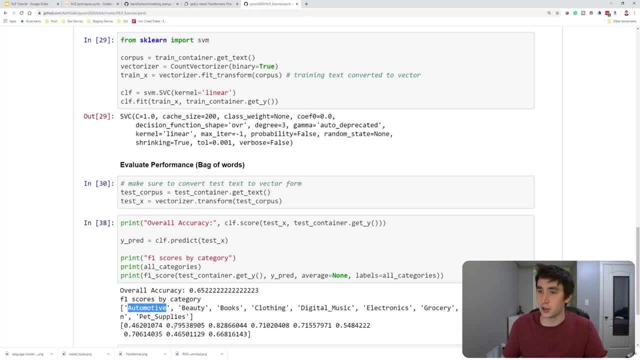 really bad job on the automotive questions but did well on beauty and books, and you can kind of utilize this data as you see fit and play around with building different types of categorizers, classification models, around this. a couple of recommendations I have. I think it'd be really interesting to see how. 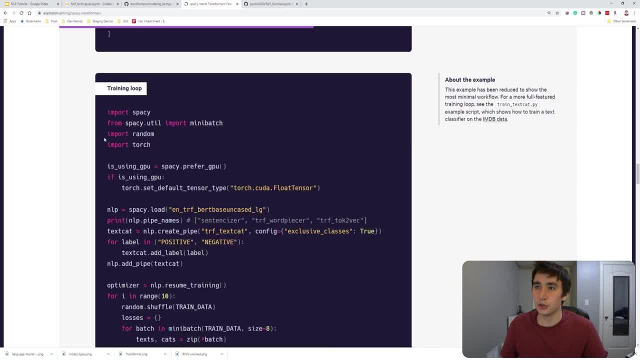 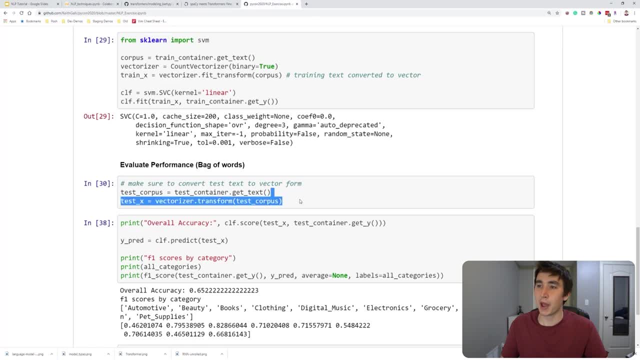 well a fine-tuned Burt model would do on this task. I also think it would be very interesting to take the bag of words model but also leverage some of those other techniques we mentioned. so like lemma, tizing words, stripping away, stop words, you know, maybe doing some part of speech tagging, see if you can leverage. 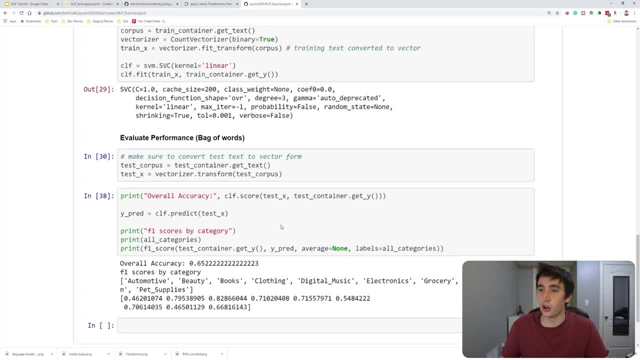 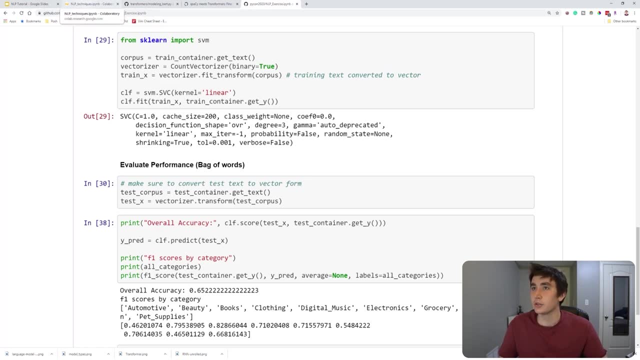 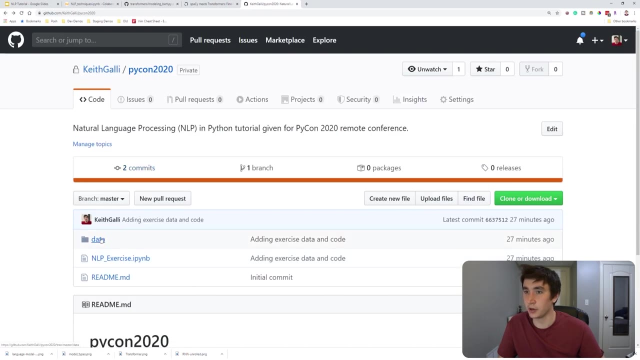 that into make it more important. well, I'll see you next time. all really interesting techniques to try to build more powerful models. what else do I want to say here? I guess quickly. I didn't actually show you what the data looked like, but if I actually clicked on one of these files, maybe something like 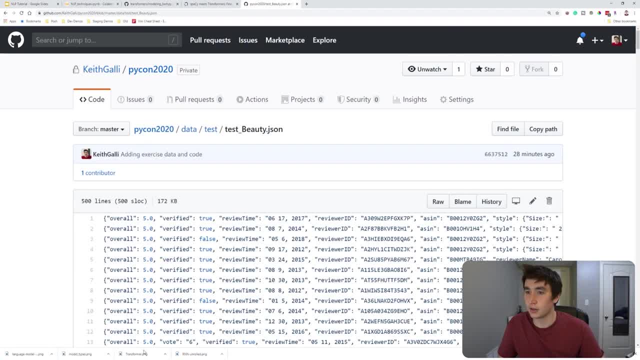 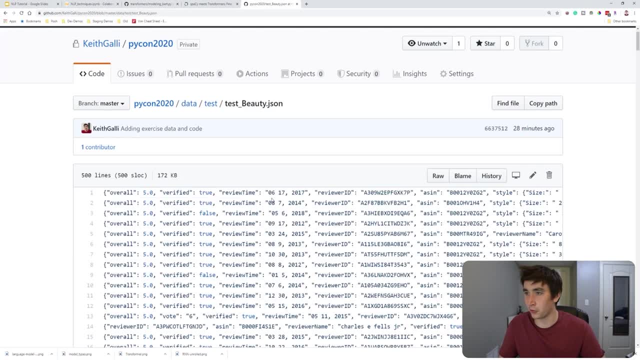 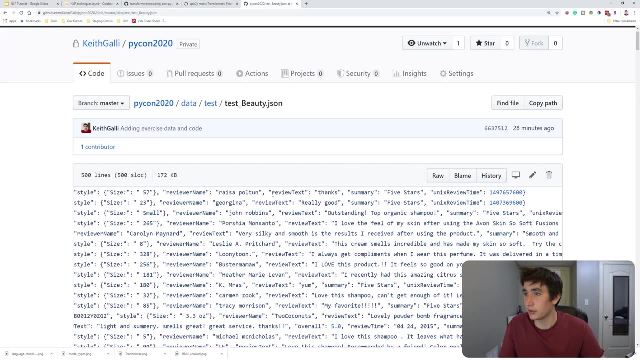 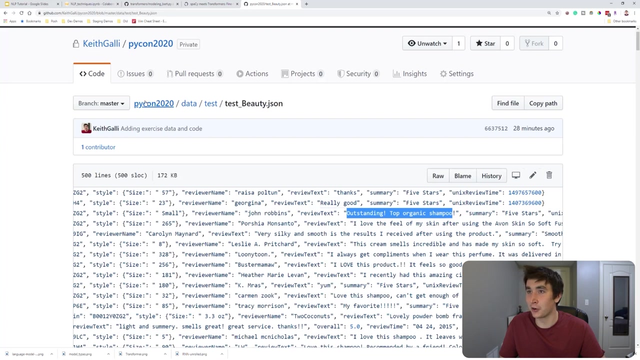 beauty would be easier to see. I also linked my source where I scraped all this data. someone already did a lot of the grunt work for me and I want to give them credit, so I'll have that included in the readme of my github page. but yeah, basically you have this review text, always talking about the category here. 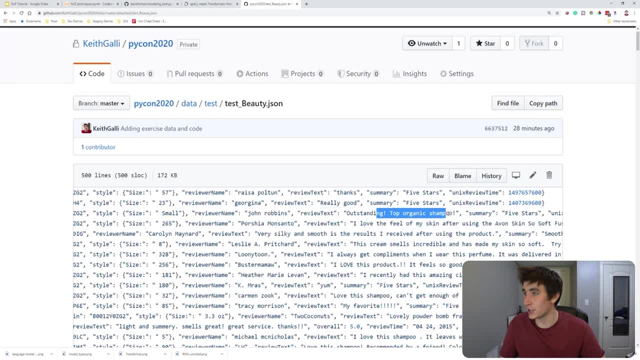 so this is beauty. so like outstanding top organic shampoo, what our model we would expect to learn is off of the shampoo. one thing to note here is: this is not perfect data. you'll get some reviews that are different and some of them will be a little bit different, but you'll get some. 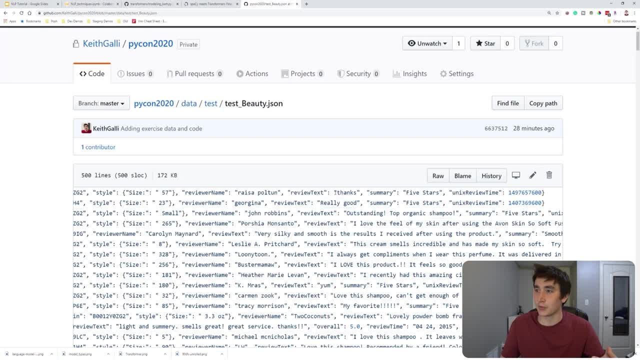 reviews that are different and some of them will be a little bit different, just like really good and thanks, and they don't give us much information. so we're never going to be able to get like a hundred percent on this task. but maybe another exercise you could work on is 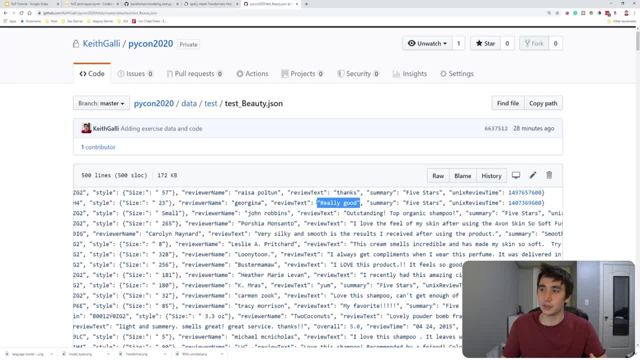 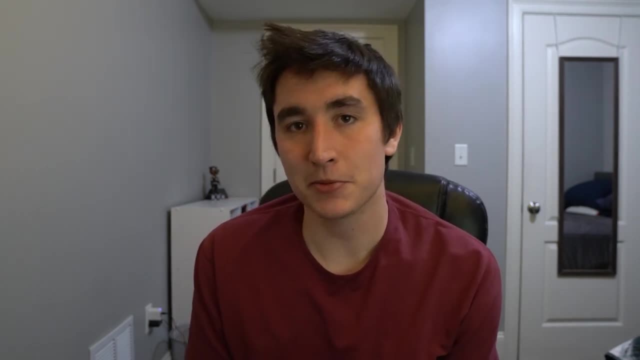 how could we strip out these kind of non-specific types of words and not use them as training information and test information? all right, we're going to end this tutorial here. hopefully you had some fun learning about some different NLP techniques in Python. there's a lot we covered. 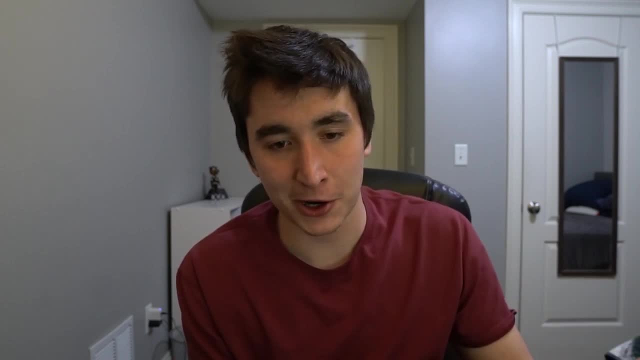 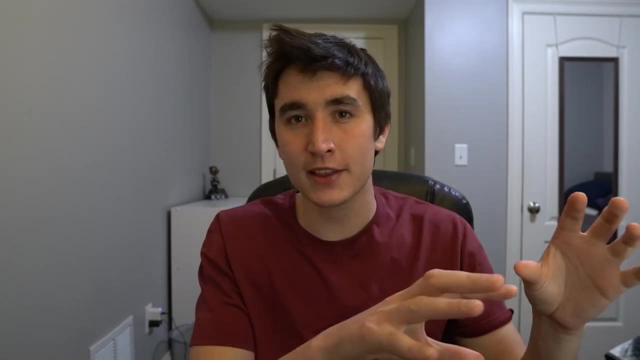 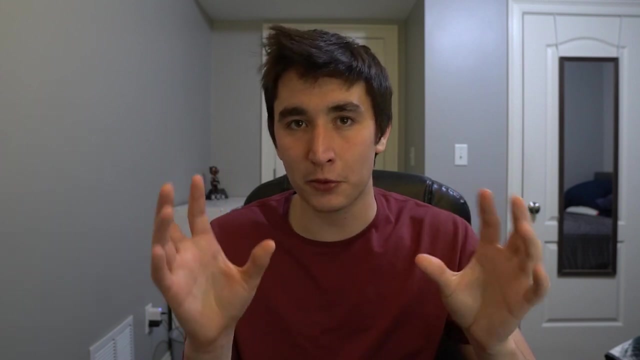 in this video and hopefully my goal out of this tutorial was for you to all see some of these techniques and have them in your mind so that you could take them and kind of build on your knowledge and apply them in different areas. so really it's like seeing all of what you can do.